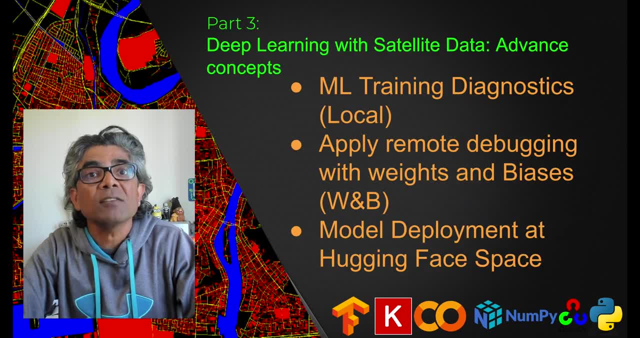 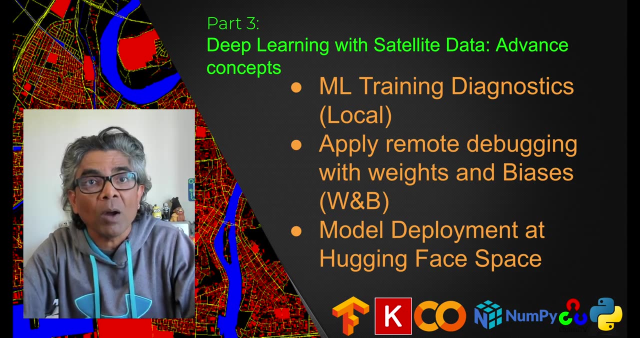 in this model, we will learn how to extract the details or the output related to the activation, as well as the gradients, through our deep learning training process. The model which will be generated as the output of this whole exercise will be deployed at hugging phase, where just passing an 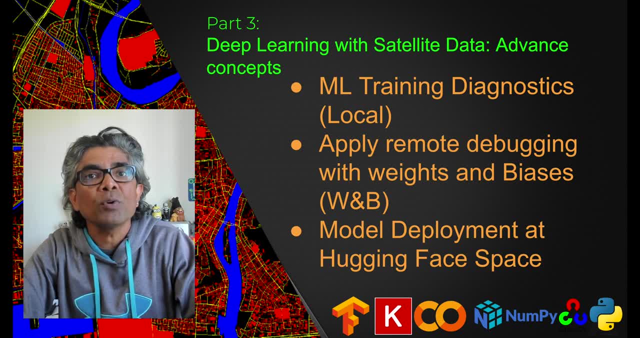 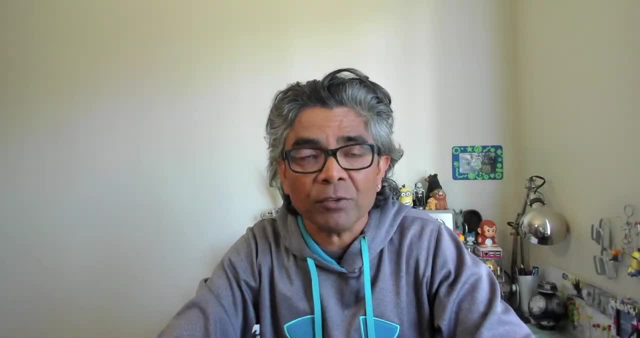 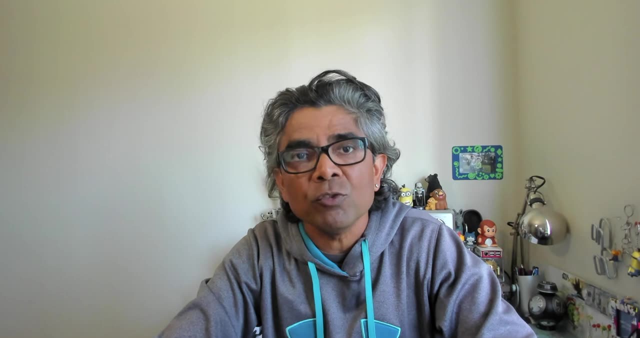 image, you can generate the output based on the classes which we are going to train in our model. Overall, this, This hands-on exercise or the hands-on workshop, is going to be very useful for anyone who is starting their journey with the deep learning, as well as the anyone who is expert, but there. 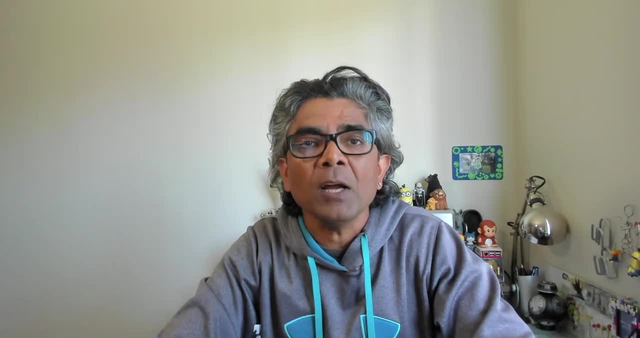 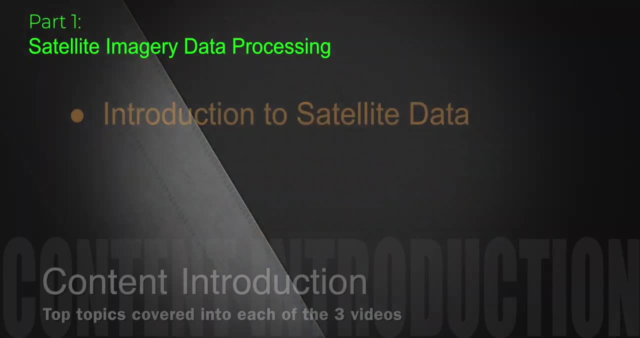 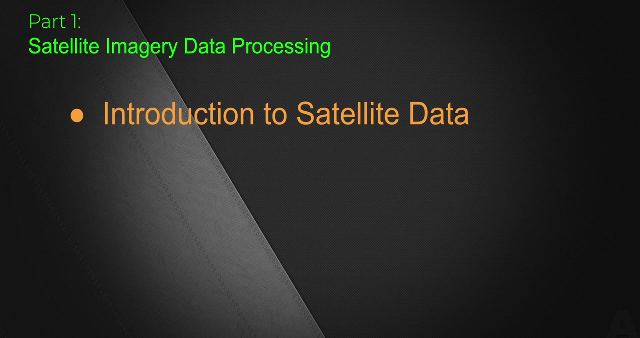 will be a lot to learn for everyone. So let's take a look what we are going to cover, even in details, in each three parts of this web series. The video starts with the introduction to the satellite data: how it is collected, how it is generated and how we really start processing when we perform the training. 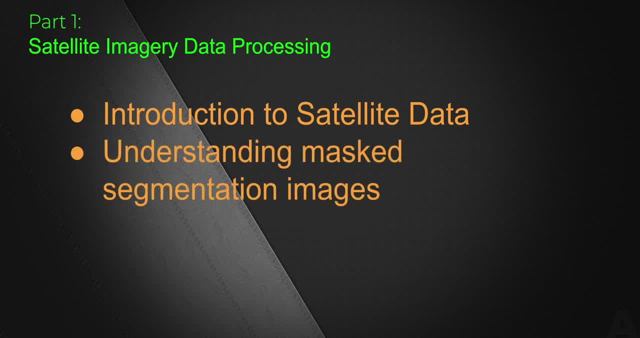 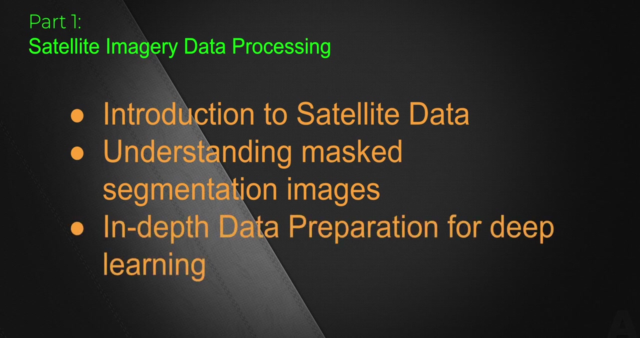 Next, we learn the generation of the masked segmented image for each satellite image tile. The labels generated for the masked image are also being explained. And finally, in a Google Colab environment, by using the Python code and various Python libraries, Such as NumPy, Matplotlib, Pillow, Keras, TensorFlow, Patchify, OpenCV and few others. 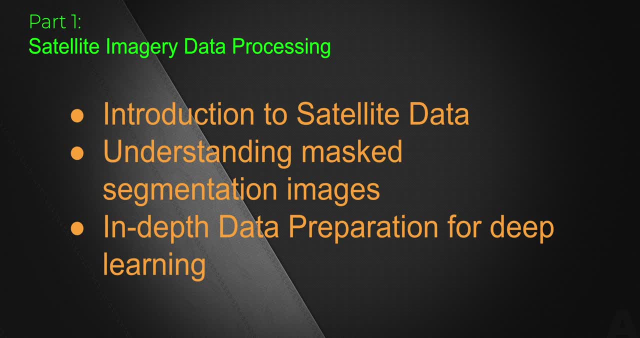 we are going to learn how to prepare our data by combining the training images with segmentation images and the labels to generate our data, which is ready in the form of training and test package for the deep learning process. So the output of first part is going to be: 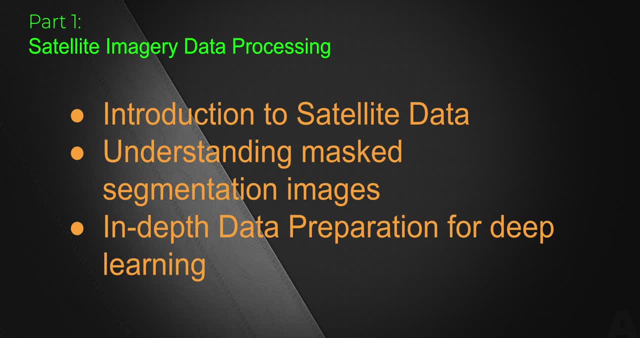 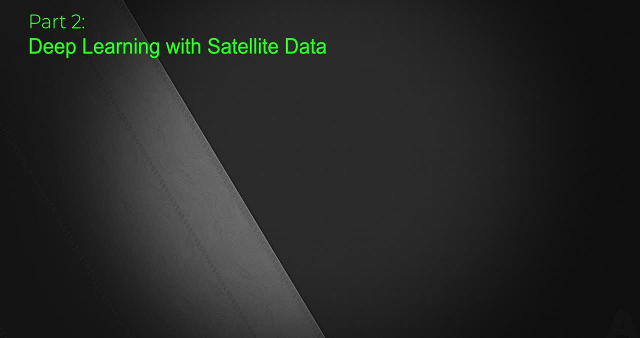 the training data which will be applied into the part two of our video. The part two of our video is all about performing the deep learning with the satellite data. First, we need to learn the U-Net model, which we are going to be based for our deep learning. 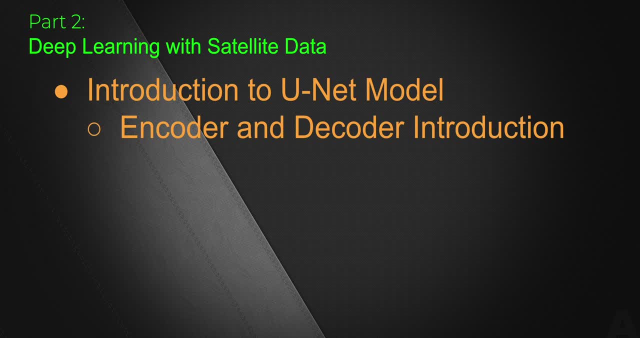 process. So we need to know the encoder and the decoder, which are the integral part of our model architecture. Here we are going to learn integrated model architecture. For that we need to know the process for the deep learning process. So the first part is going to be the training data. 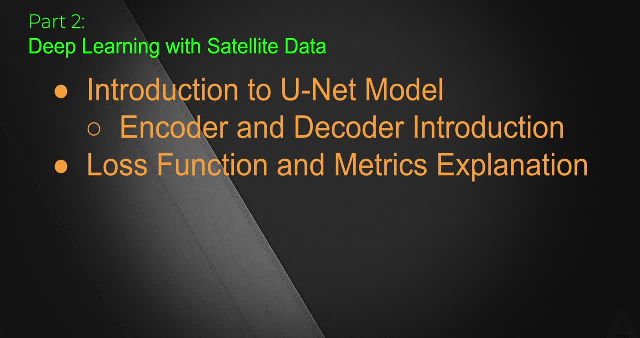 next, we also need to learn more about the loss functions which we are going to use in our training process and the metrics which will help us to learn the deep learning process outcome. by using the jupiter notebook in a google collab environment, we will code our whole deep learning. 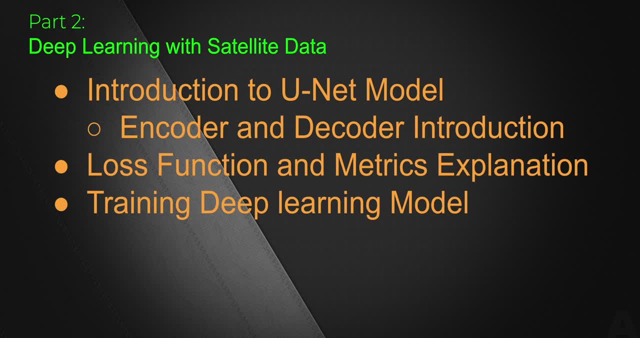 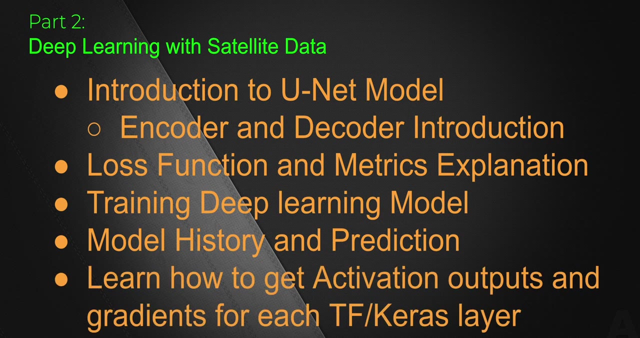 process and perform the deep learning. training and the output of this process will be our model. we will learn the model history and apply the model for serving or to generate predictions. after the first iteration of our deep learning, we will apply another python library so that we could get the activation outputs as well as the gradients for the each layer in our deep learning. 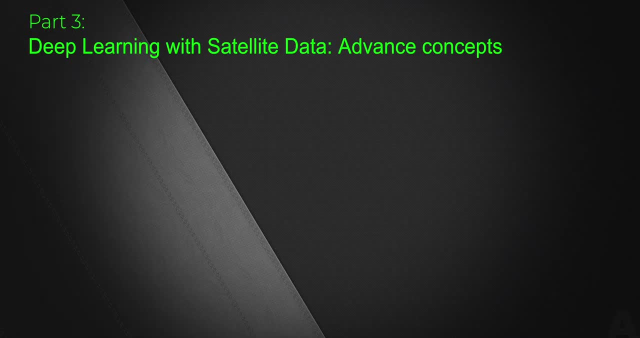 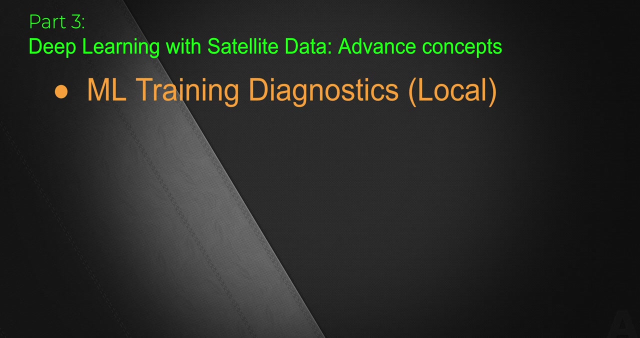 network. the third part will be the extension of our second part, where we are going to apply the various advanced concepts in our deep learning process. first we will learn how to perform the diagnostics for the deep learning process at the local level and then we are going to apply the remote debugging or remote. 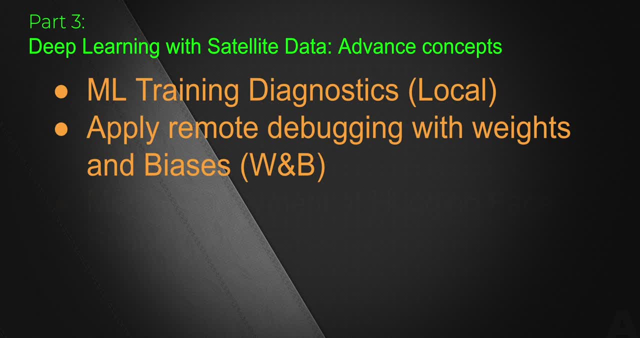 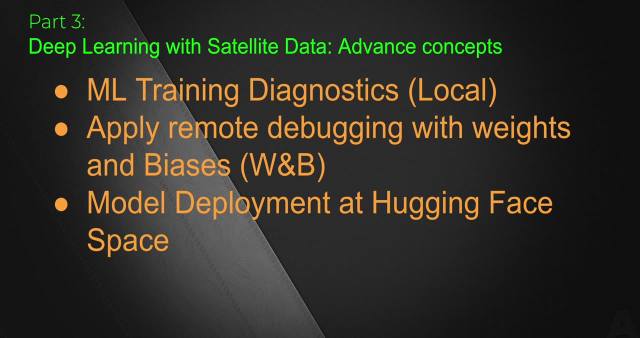 diagnostics by using the weights and bias. in the third step, we are going to deploy our deep learning model at hugging face space and our interface to the model serving will be the radio base ui. we are going to create the gradio base ui, which will take a particular image taken from google maps and our model will perform the. 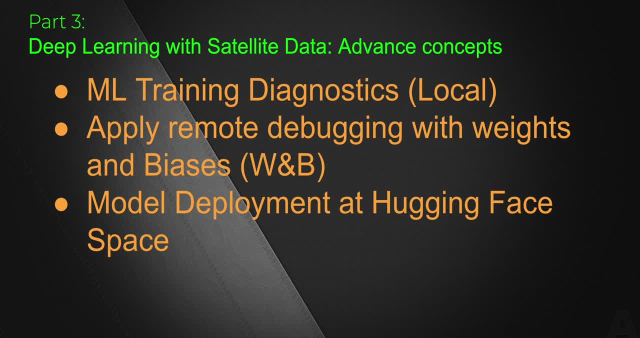 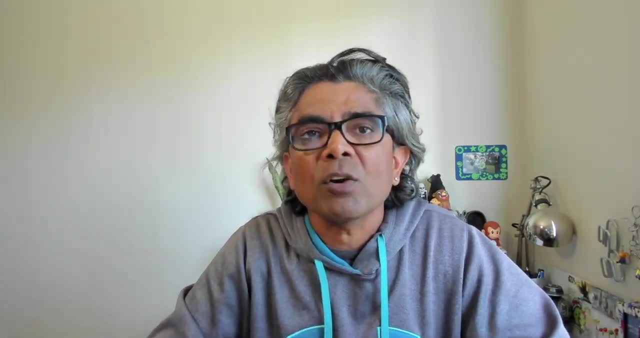 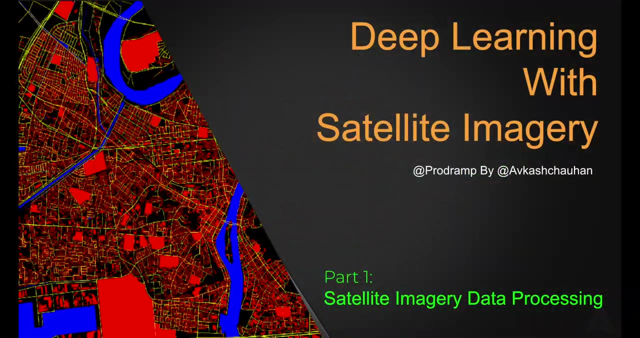 prediction to generate various landmarks in our given image, based on its training class. So now, without any further delay, we can start the first part of our video, where we are going to learn the data processing for the satellite imagery. The foundation for the satellite images are the 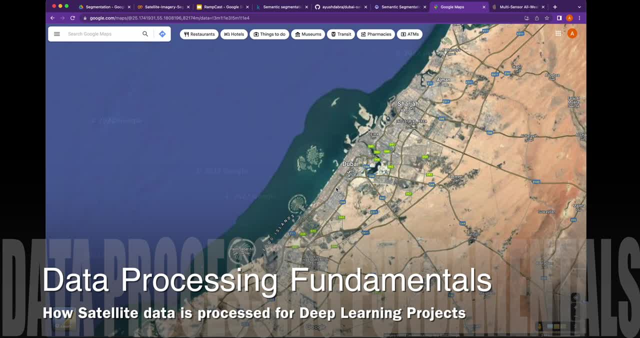 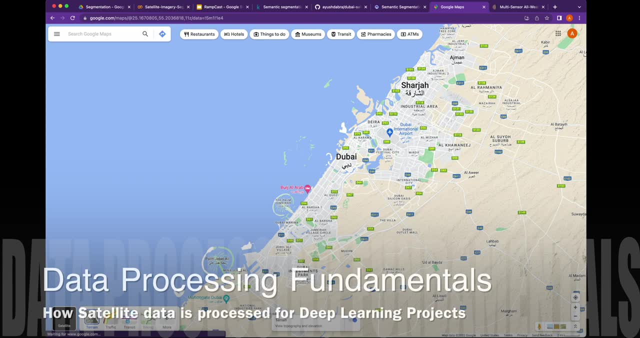 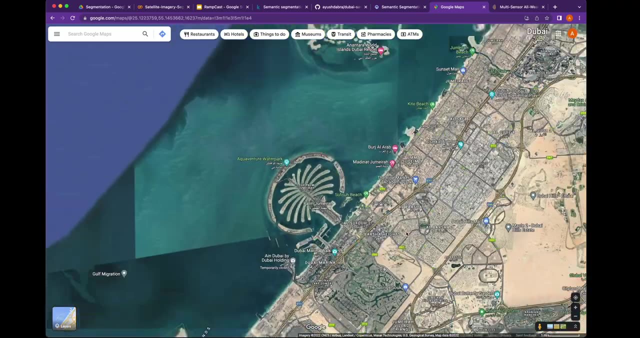 satellite maps which you can get from any mapping service, including the google maps. So, looking at to the google map, then you can really set up the particular layer, which layer you are interested into. but if you look into the satellite view of the layers, that's where you will be able to see. 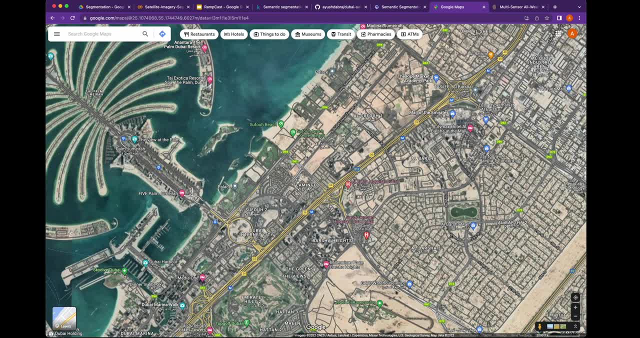 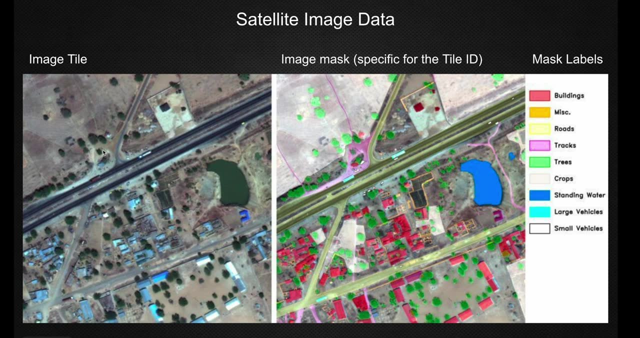 the map and using this map we generate the satellite imagery data for deep learning. This data is the map. data is translated into the three different segments. These segments are the tile image, So the tile image is a one particular tile coming out from your satellite mapping data. 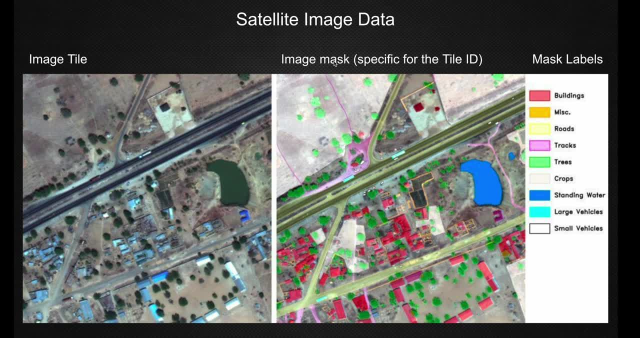 For the label data, we have to create the image mask, which is the masked image of the given image tile. and the mask labels are the list of items which you would want to define in your deep learning model so that you could predict in your input data when you are. 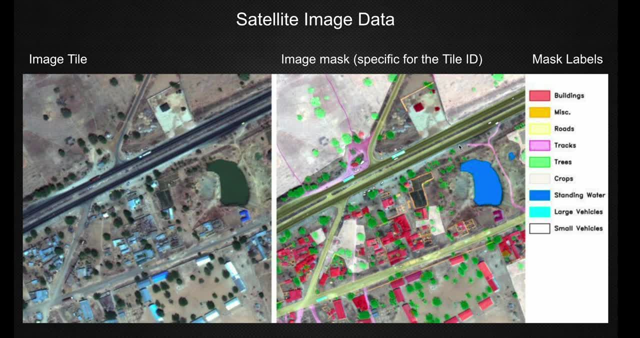 applying your model to figure it out which particular class of items you- your model- can predict into given image. So in the left side is your source tile and in the right side you have the image mask and the mask is showing the particular labels which this given tile has been. 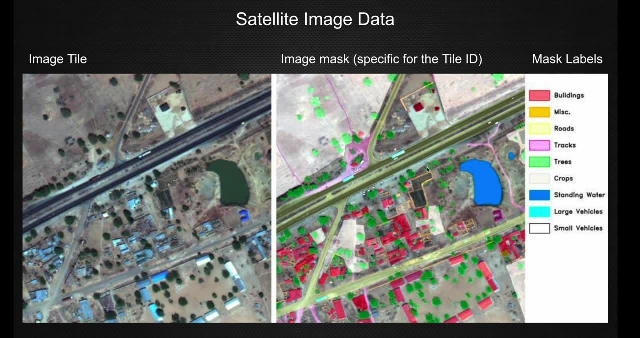 classified to. Here you could see there are various types of labels which are being classified to. Here you could see there are various types of labels which are being classified to. Here you could see there are buildings, there are miscellaneous objects- roads, tracks, trees, crop, standing water, large vehicle. 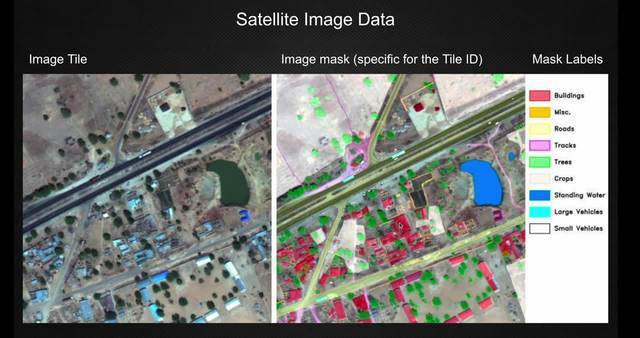 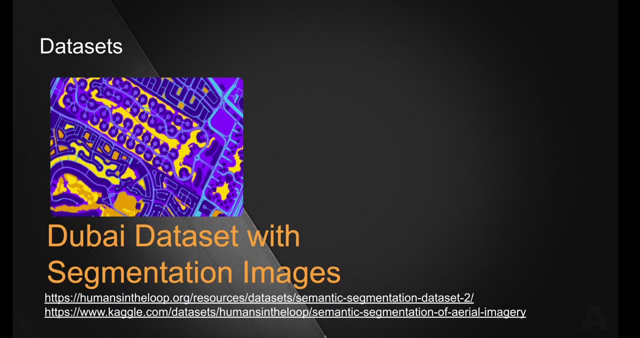 small vehicle, so the limit could be anything whatever you would want to train for. The only thing is that you have to provide the training data which is sufficient enough so that your model can learn from the input data, The data set, which we are going to use in our project. 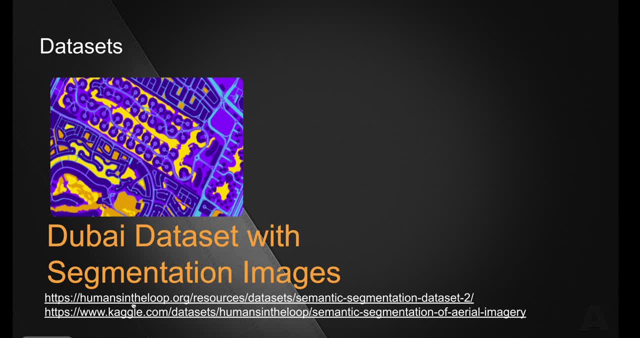 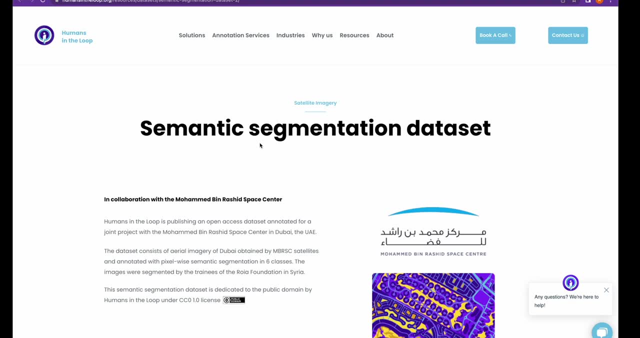 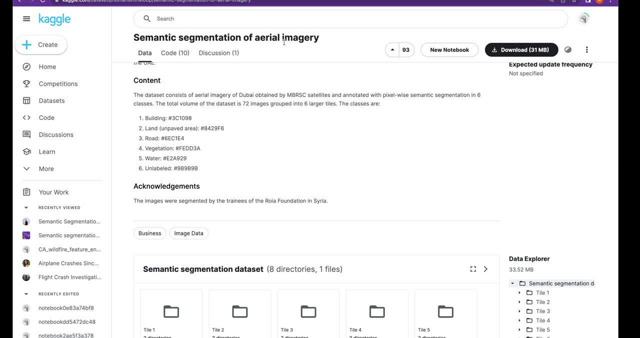 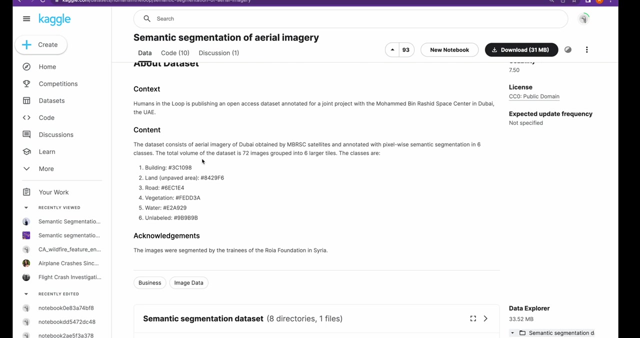 is coming out from this Dubai data set which was released originally in the b UA which was introduced in the area fromasters, those by artifact labels. there are six label, five landmarks and anything else which is not landmarked classified as a unlabeled. so we are going to use this data set with 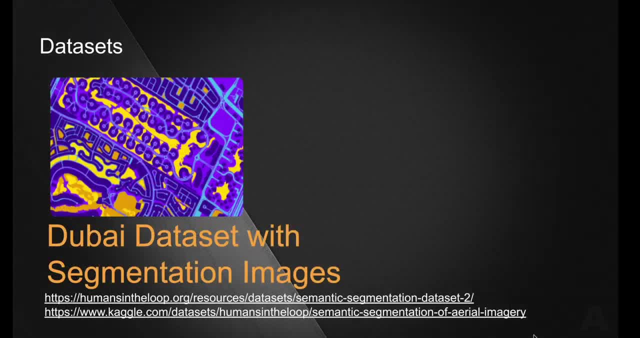 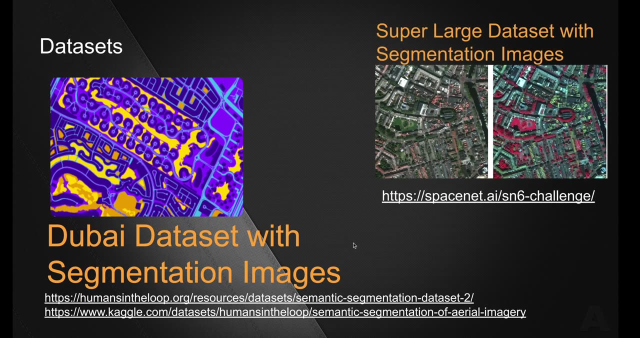 this class description to process further. next, if you would want to use the same code and you would want to apply on a larger data set with a few tweaks here and there, I have another introduction to very large data set which is even much bigger in size, as well as the much bigger in the labels. so 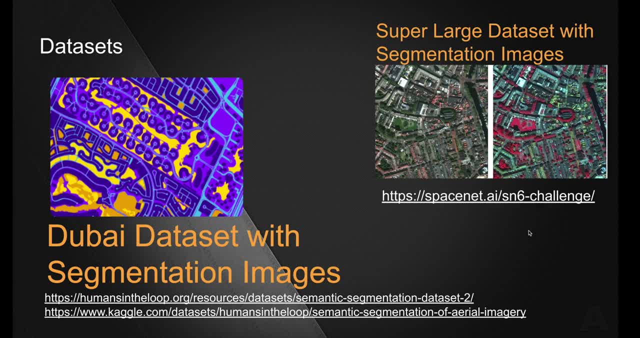 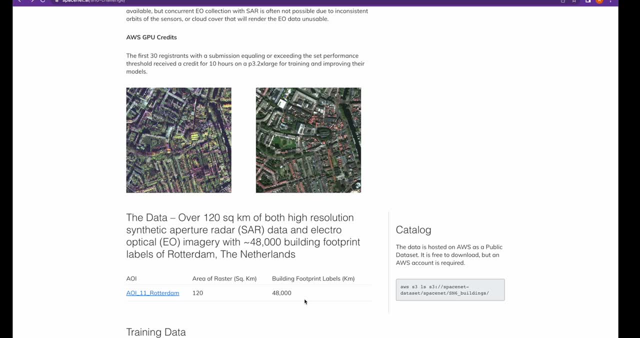 this is space net dot AI as an x6 challenge website where you could get the data and, as you could see, that the initial data set is actually designed, or the taken from about 120 square kilometer, which has about 48,000 building footprints from the Rotterdam, the Netherlands. so looking into this, 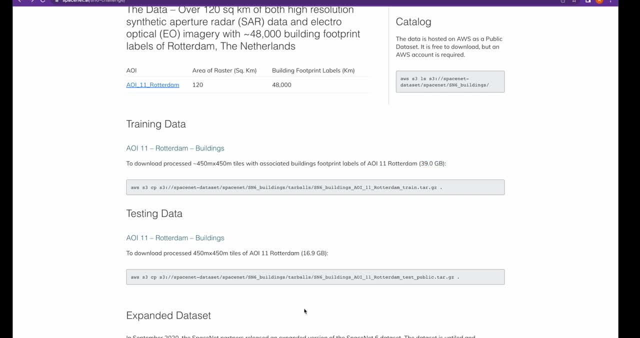 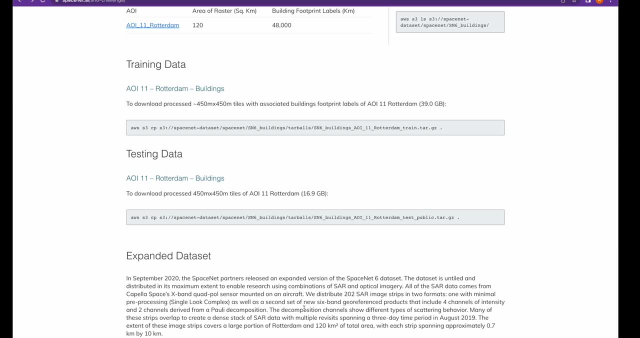 data set. we are going to use this data set, which is even much bigger in size, as you could see, this is about 39 gig, but if you would have the patience to really go ahead and try the learning which you are going to get from this tutorial, you 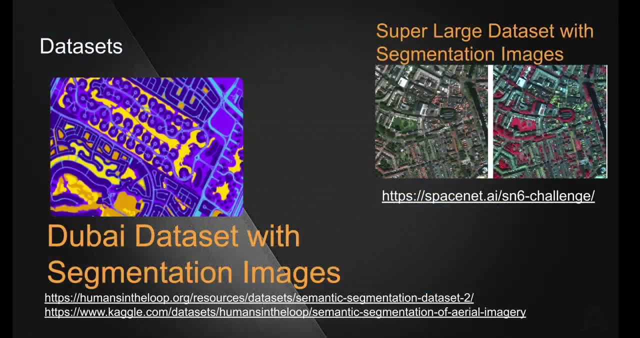 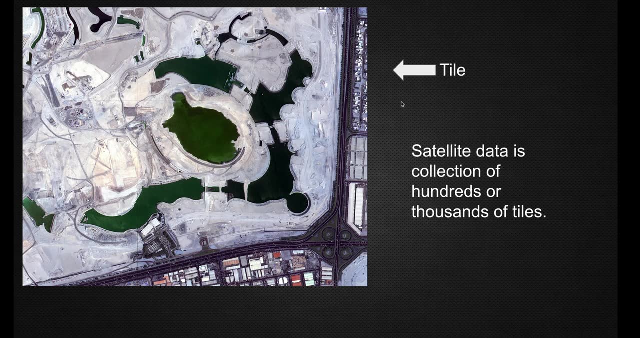 can definitely apply it. now let's spend a little more time and learn more about how the data set is going to be processed by us. in our deep learning model, we have already learned the satellite data is taken and split into the tile, so each set, the input data set is. 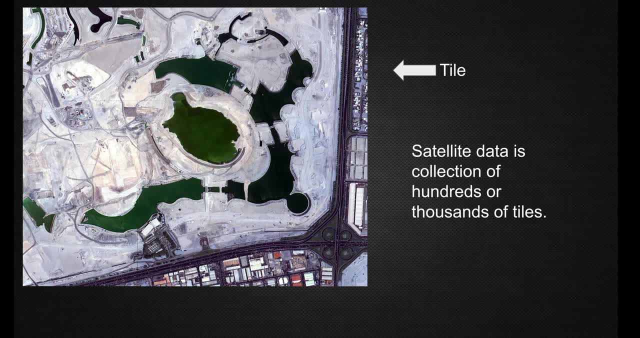 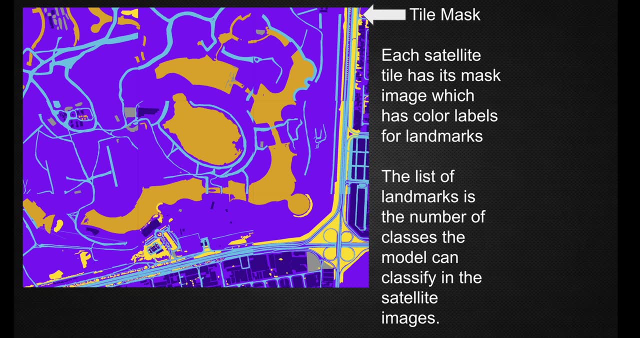 set will be a collection of hundreds of or thousands of these tiles. for the respective tile, there will be the tile mask. so, depending on your tile sizes, there must be a mask for it, and the the landmarks are also specifically laid out in the mask based on their specific color. so, depending on how complex your input data set is, 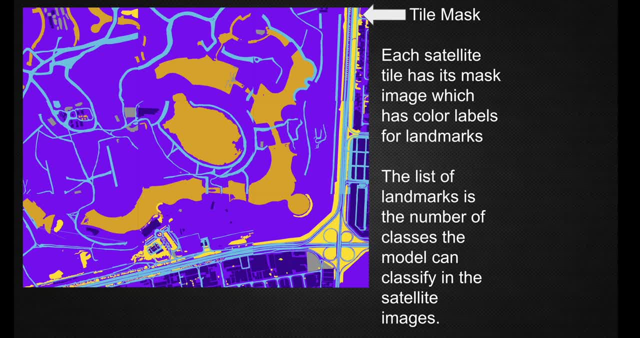 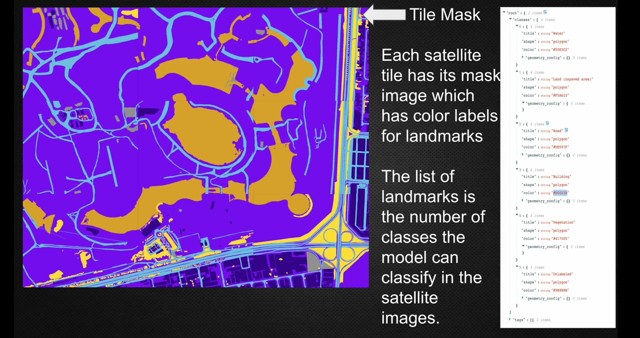 the list of labels is also going to be to complement the mask. that is very important aspect of mask for the given tile, as you could see here in this JSON for this given image. here are the list of classes this particular mask has and for each particular class you can understand. 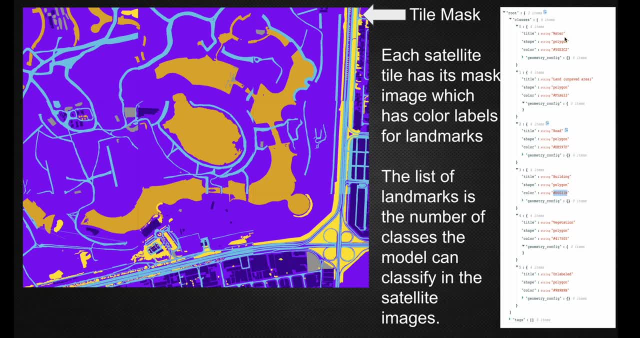 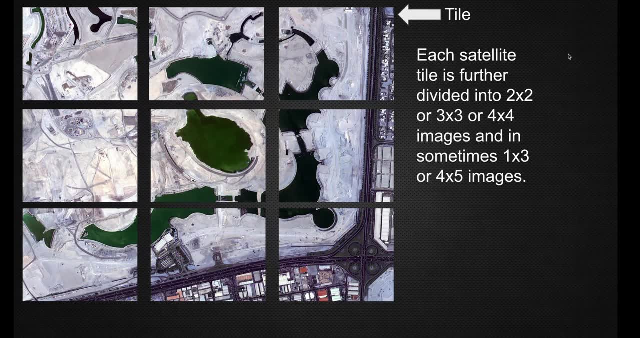 the type, which is a polygon, and for each type label, what is the adjacent color. further, the tile sometimes could be really very large. so the each tile is further divided into two by two, three by three or even four by four images, sometimes because the tile may not be perfect square. 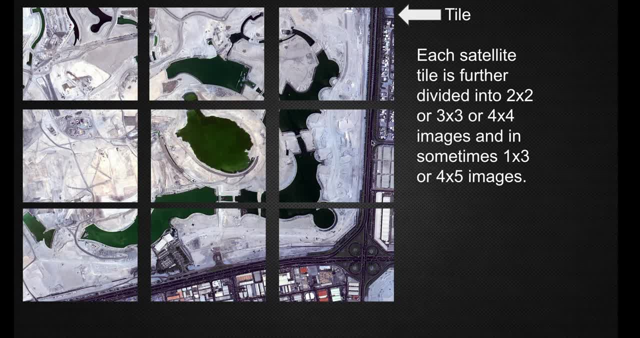 if it is a rectangular, then it is very much possible that the tile image could be in the size of one, two, three, four by five. it could be any size. my point is to share here is that you cannot just assume that the data should be two by two, three by three or four by four. so you, because 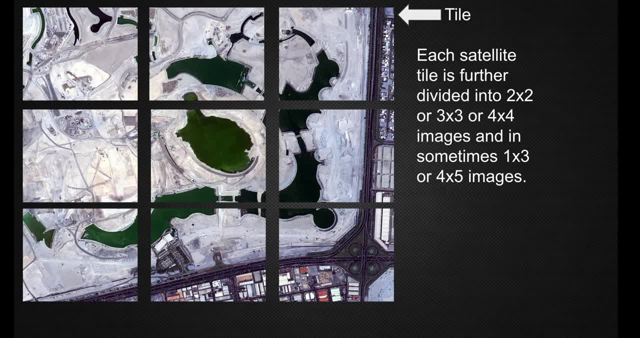 you have to make sure that before you process your data, you make sure that the data is adjusted properly for the individual tile. as it's divided into further images, the masks are also adjusted accordingly. so that's is very important to understand that when we are processing the 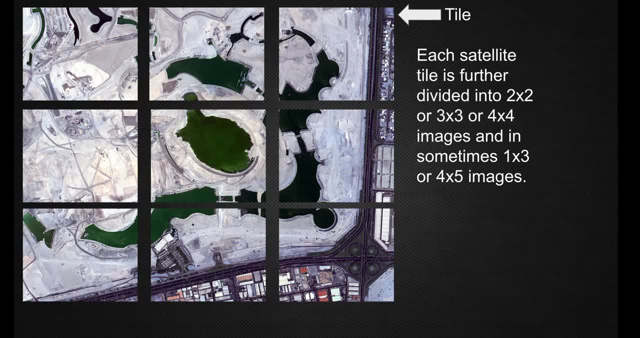 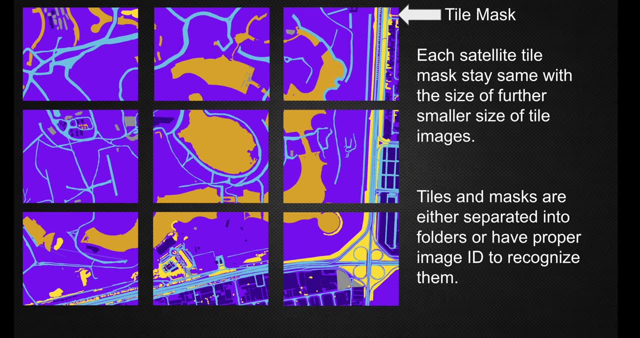 satellite data. you are going to get the tile data, which is a collection of so many images, and the tile mask data is also the collection of images. but that does not change the constitution of your label data, because labels are still the same even when we are splitting the mask image into multiple sub images. next we need to process this. 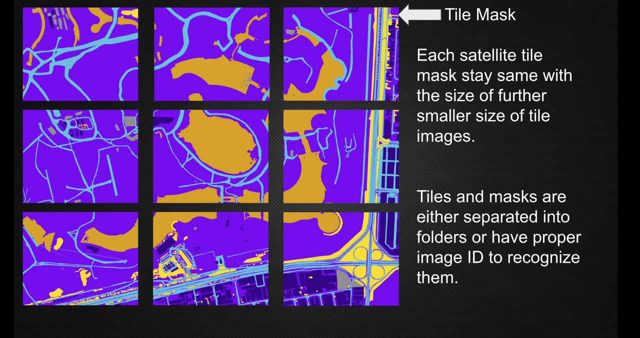 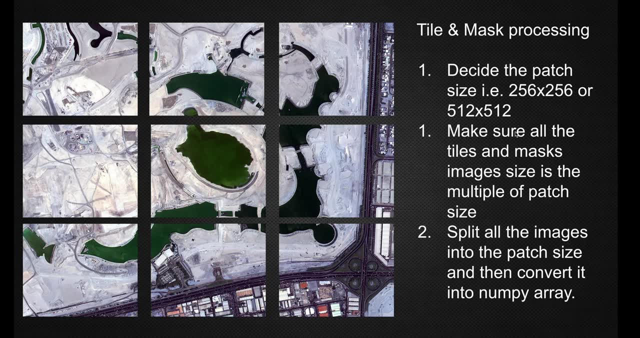 data and when we try to process the input tile data as well as the mask data, we have to make sure that we define that. what is our patch size? so patch size could be 256 by 256 or the 512 by 512, depending on your patch size. you can also understand when you are training how 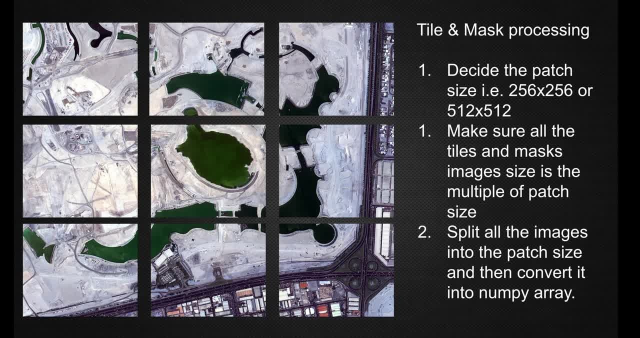 you can adjust your batch size. if you are smaller patches, you can create a larger batch. if your patch size is larger, then you can create a smaller batch. depending on how your resources are there in order to process your input data, then what happens is that very first thing whenever we 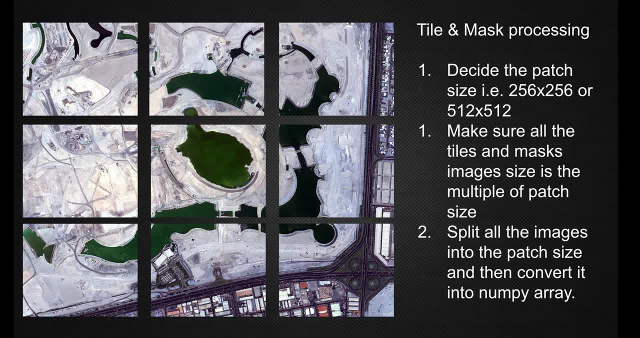 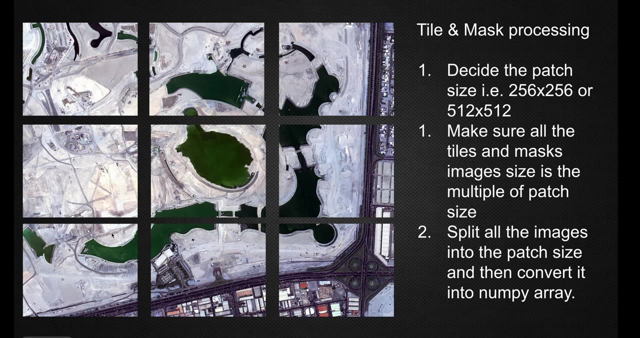 get these images, we actually take these images and we make sure that these images are the size of our patch size. so first we adjust all of these images, reshape them so they are based on our batch size, and then, after we take these images and then we split them even more so that we could. 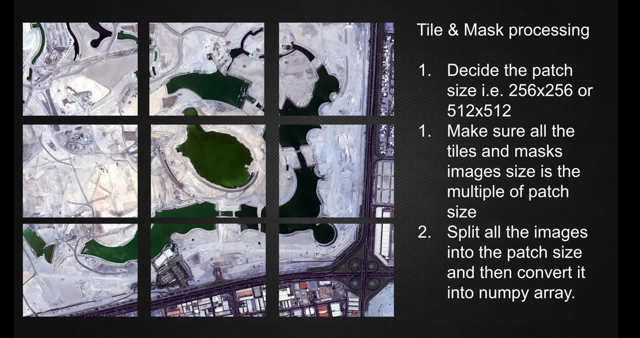 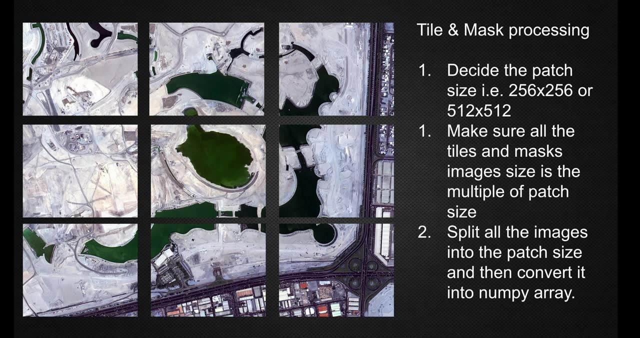 create the patch of every image and every mask image with the size of our patch image and that is what becomes our numpy array data which going to be fed into our machine learning training system. this step is very important and we are going to follow in our workshop. really very 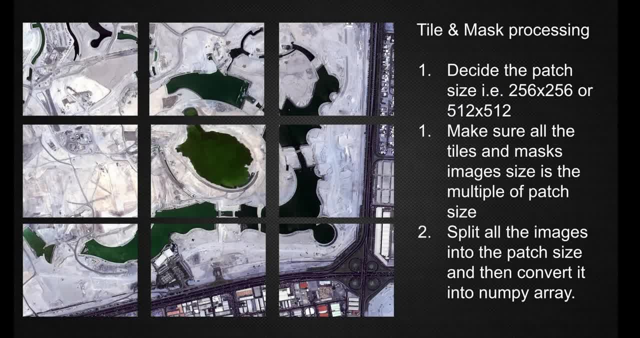 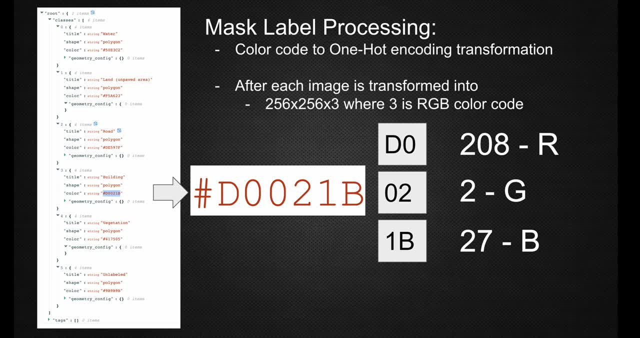 seriously and I will guide you step by step. in the next step, we need to understand the label processing, how we perform the one hot encoding to the labels. so just an example for the given data, this is the label class file, so every label is defined in a hex color. however, if you look, 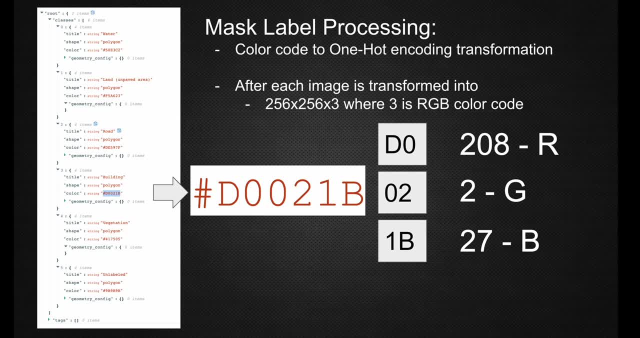 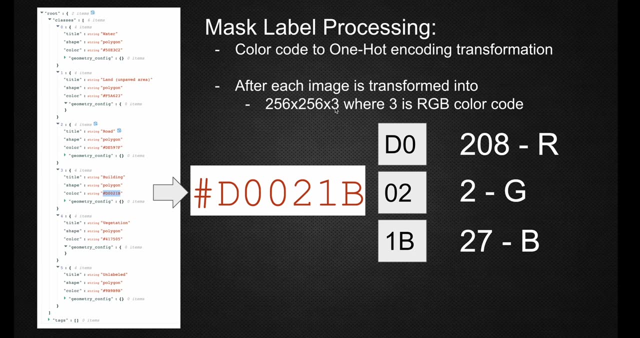 into the images, when we process them through any image library, we get the RGB color. so, for example, when we process them, we always get the height times, width times, the color coding, whether it's a RGB or it's a gray scale. if it's a gray scale, then it becomes one, and or if it's a ygbr, then it's. 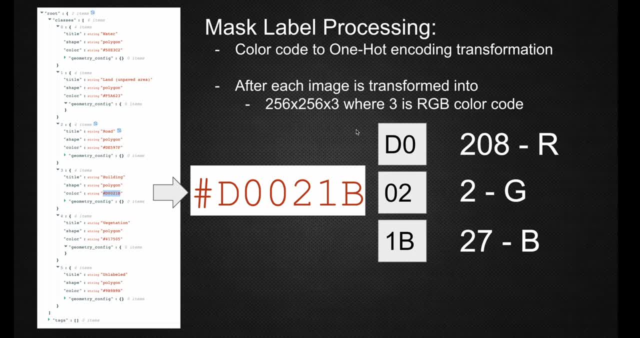 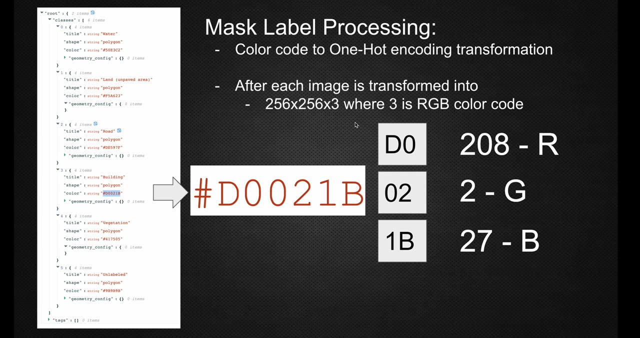 became a very different. so depending on encoding, we have to make sure that labels are properly adjusted. so for a given hex code, we split them into the proper RGB and then, based on RGB, we match the proper label. so we need to also process the label labels from hex all the way to 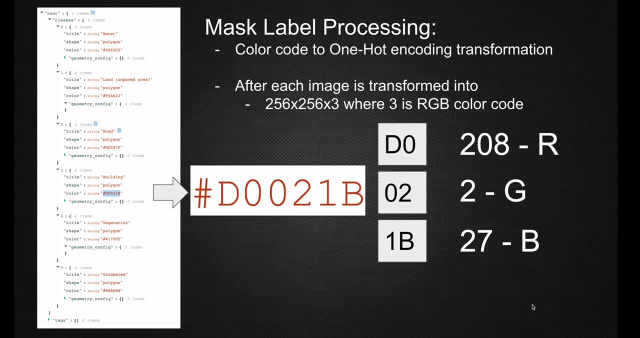 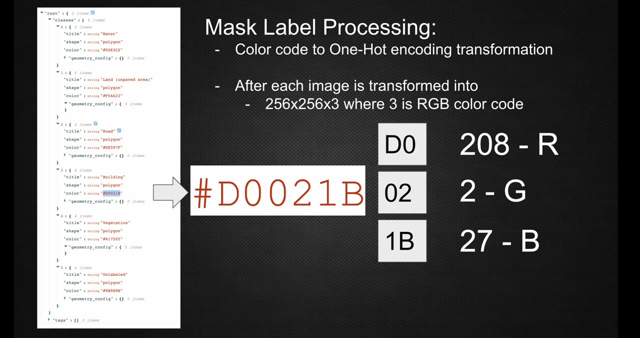 RGB. so that is another part we perform in our satellite imagery data processing so that the labels are recognized correctly based on given data set and their corresponding mask. so I think this introduction should be enough for us to go ahead and we can start coding our data processing. 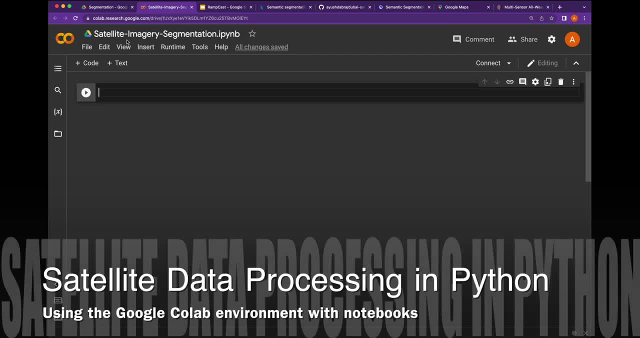 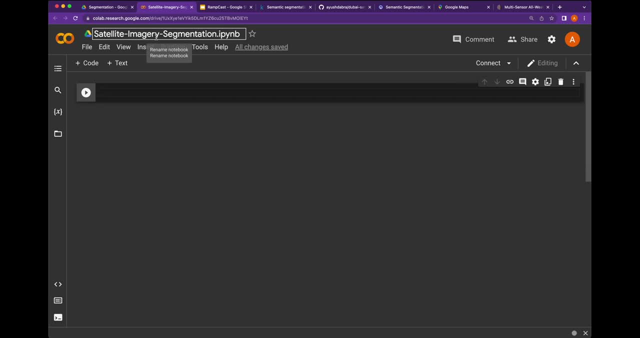 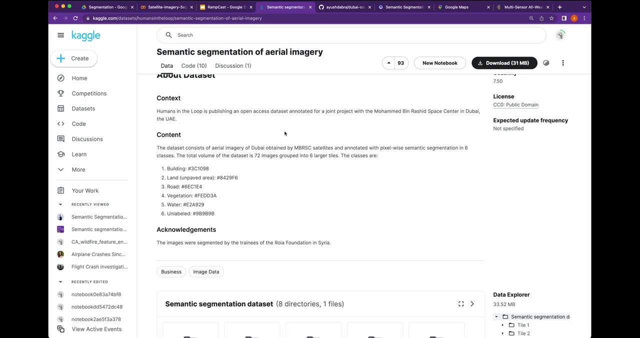 step of this workshop. I have created this colab notebook at Google colab. you can also use the free version of Google colab for this whole workshop and the data set which we have talked about here. I have already downloaded this data set directly from the Kaggle and I have uploaded this data set to 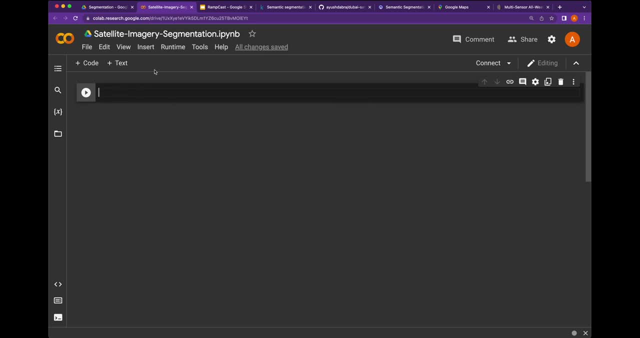 my Google drive, which we are going to connect with this Google colab notebook and access directly. one other option is that if you do not want to connect Google drive, then you can upload the data set whenever your Google colab environment is ready. so first I'm 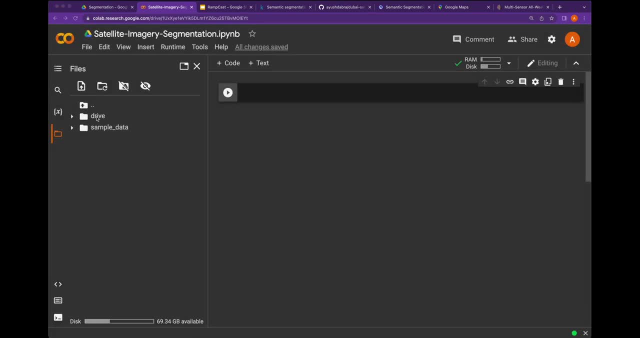 going to connect the Google drive. now the Google drive is connected with this environment, so I will go ahead and I will show you that elements was leh, that this is the place where the satellite data is and the data set is available in this, the way data set. so if you would want to look into the content, 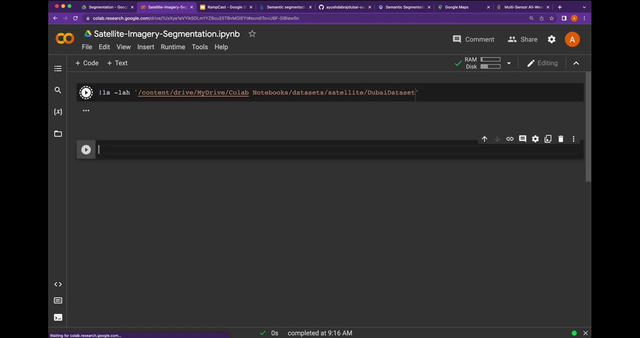 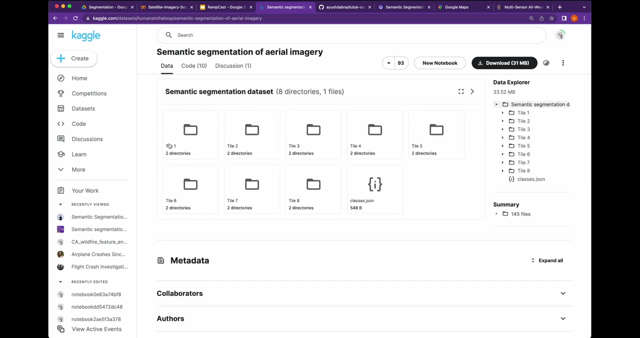 it here and that's where you could see that all the folders are tile one to tile eight and there are the classes respective to this data. so this data set which we have just seen is from tile one to tile eight and each tile is a collection of images and each image, what we are seeing here, 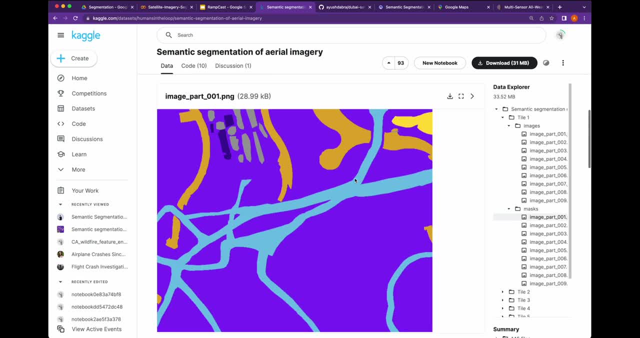 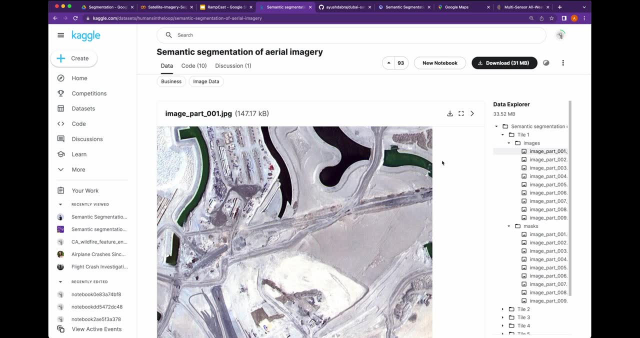 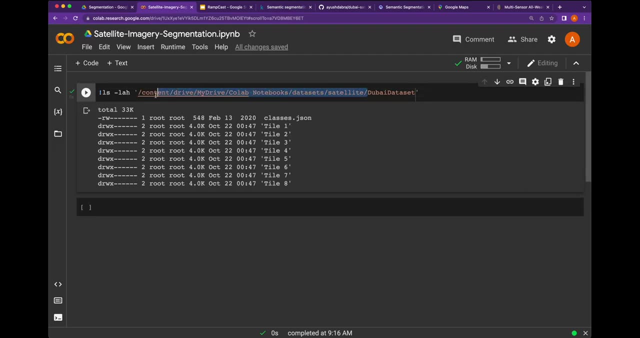 is the respective mask here. so here is the mask for the first image. the source data set for our workshop is quite easy for us to understand. once we understood the foundation of data satellite data set, we are going to create the foundation of our data set, so we will call it data set root. 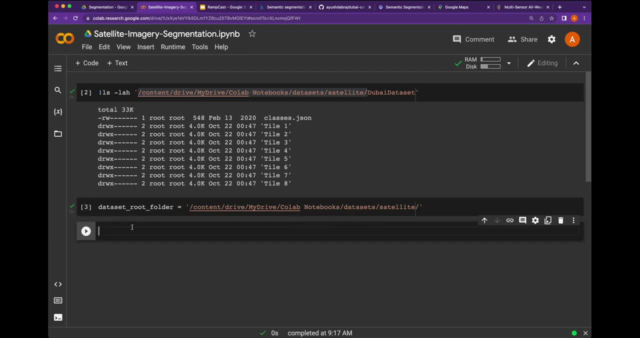 folder is this and we will select the data set name. because the reason i have created this way? because you can use- you can use the data set name and you can use the data set name and you can use multiple data sets when you are using the same jupyter notebook. so data set name will become. 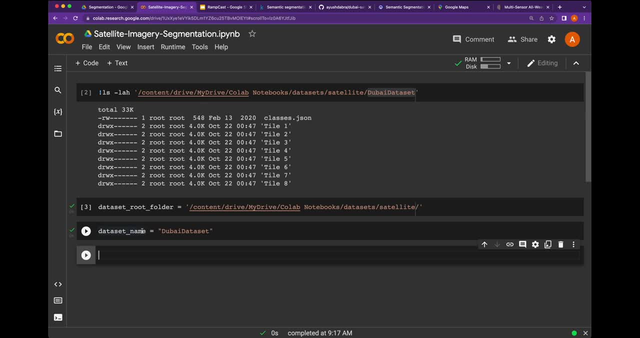 this dubai data set. so these are the two entities which we are going to use for our source data set. now our next step is going to process the images, or and at least learn the images which are available in these folders. so we need to import the os. so i will be using this cell. so import os. 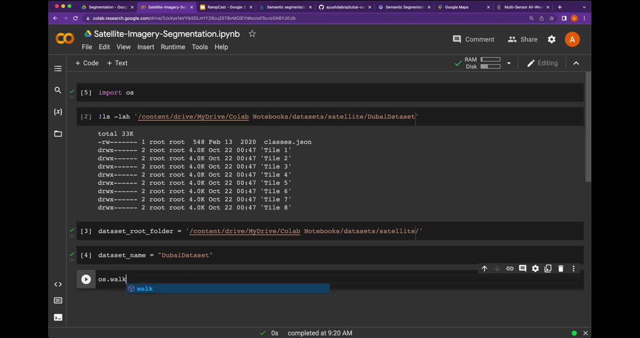 and in the os there is a method called os dot walk. so oswork method helps us to select a particular folder. so our data set root folder and what it does it actually returns us the path, subdirectories and the files. so for path and files in oswalk 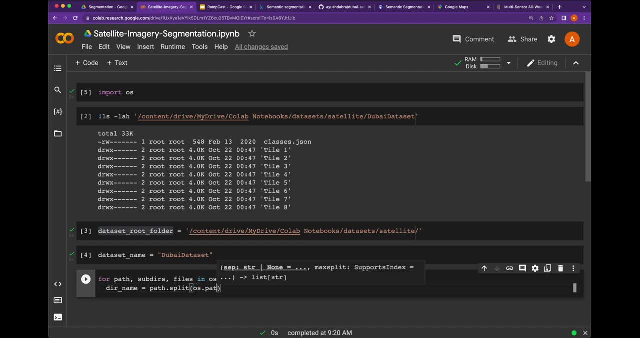 so we can take that path. we can split it. ospath dot separator because separator depend on the ож Wort path and files within 5.0. we can take that path. we can split it. ospath separator because separator. wherever you are using this code, linux or windows machine separator could be different. we are going. 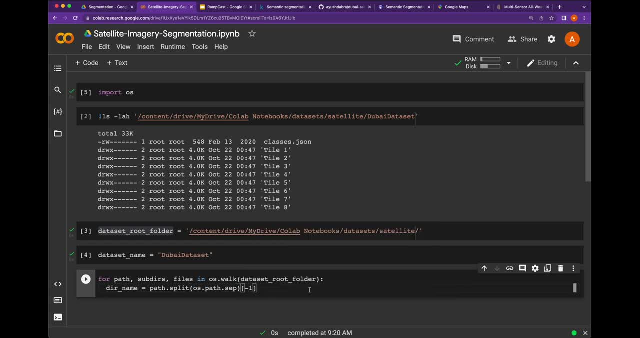 to take the separator and then we are going to use the negative one index. so that is going to give us the directory name. so if you say i would want to know what is the directory name at this point, let's print it and let's run this code. so you see here that within the dubai data set we 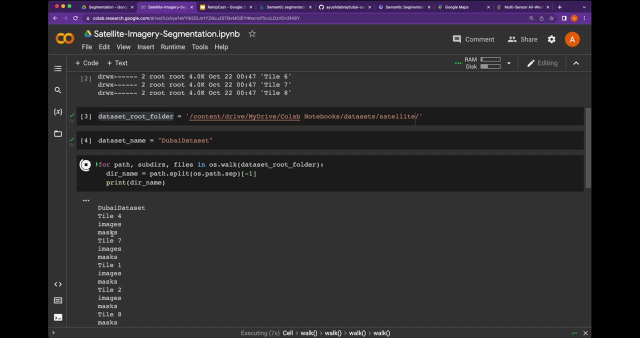 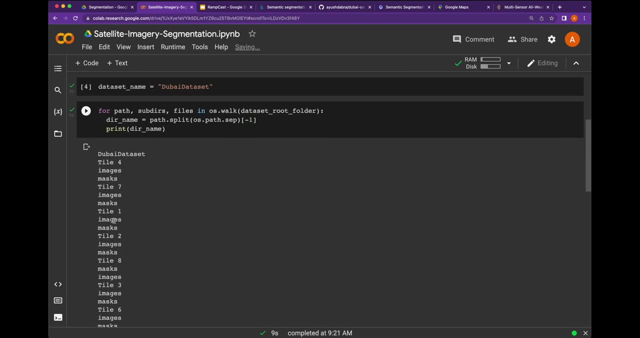 are getting the tiles within the tiles, we are getting the images and mask within the tile. we are also getting the images and masks. so for every folder which we are reading, there are the further images and mask. so very quickly we could figure it out how we can get all the directories which are 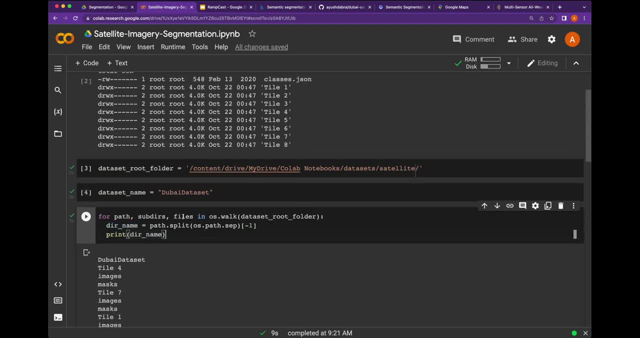 available in this data set. however, we just need to make sure that when we are using our source data set is going to be the dubai data set, so here we could actually use os, dot, path, dot, join and we can actually take this data set name to. 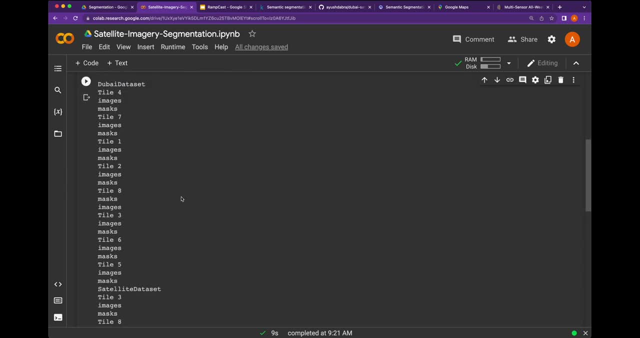 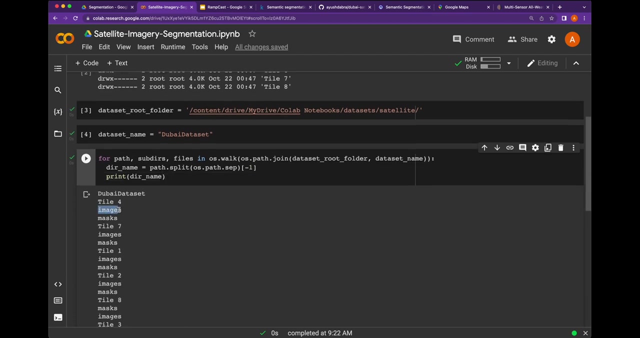 there you go. so now we will not see the other data set, satellite data set, which that is another. now, if we look into our data set, we are only going to get the folders which are available into the dubai data set. now we need to figure it out whether we want to process the images or we want. 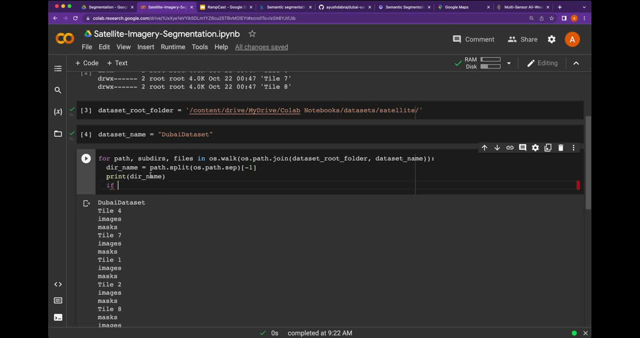 to process the mask. so here you could say: if the directory name is images, then you could process all the images. if you would want to process mask, then you can process the mask. so here now you can say all images. so images will become your os dot list directory and you can pass the directory name. 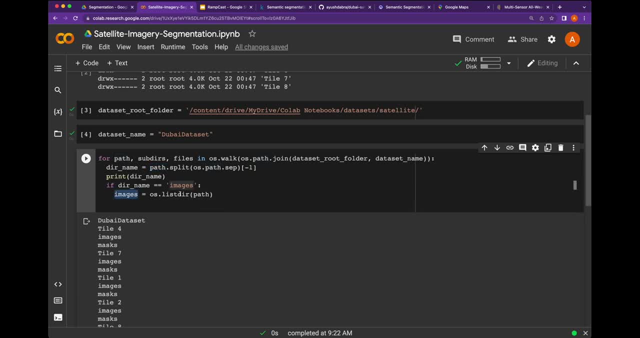 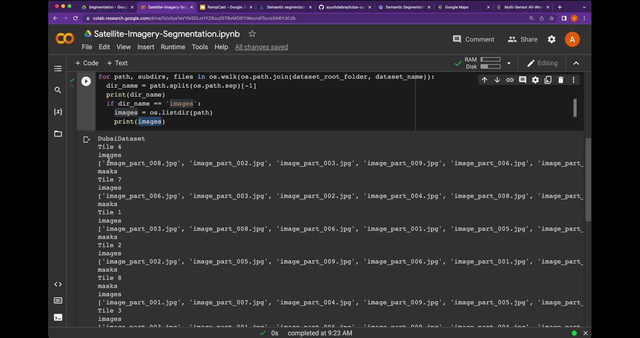 which is the path here. and at this point, images is a list. let me just give you. it may not be the good thing, but at least you can get an idea that images is an array. so, for the way, data set in the tile for a directory. we found the images folder in the directory. we found the images folder in the 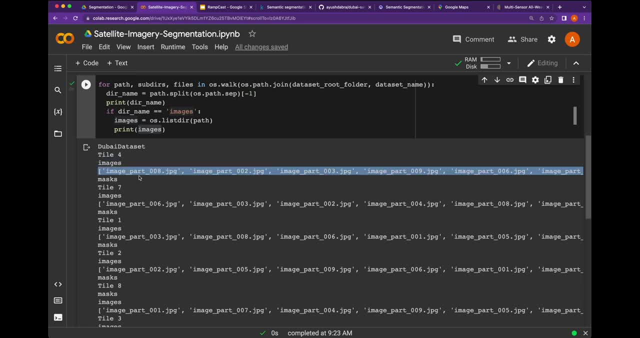 the. within the images folder here are all the images we are not processing the masks. then in the images folder, here are all the images for the tile, one folder for the images folders. we here are the images. so if we do not print this part, that should give you very quick idea that all the 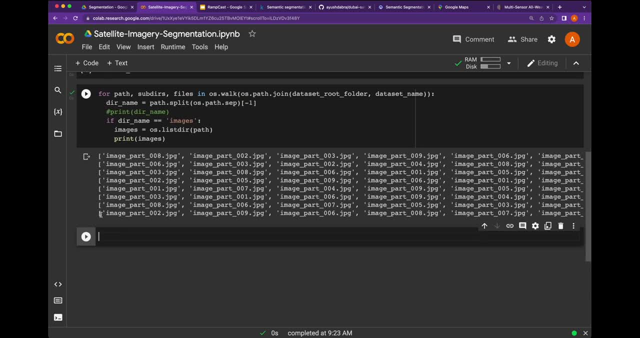 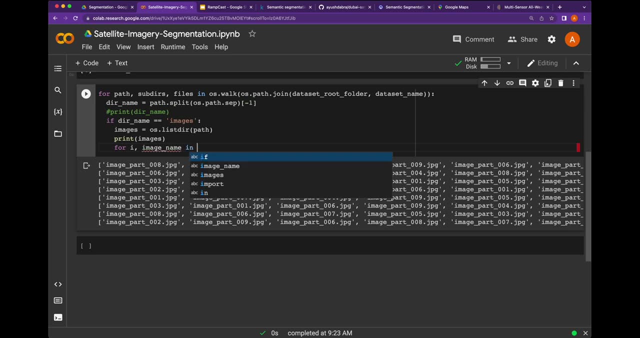 images in individual directory we have found. now we could enumerate them so we could say, for i image name in, and now here you can enumerate these images. so you could say i would like to take these images, but i would like to enumerate them and here, if you say, i would like to print. 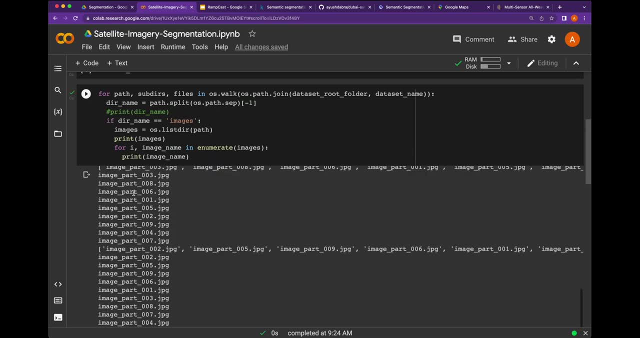 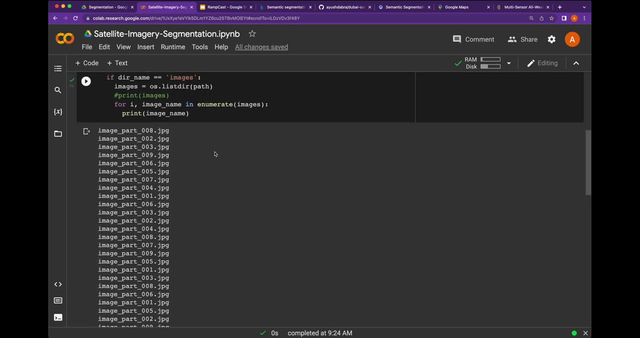 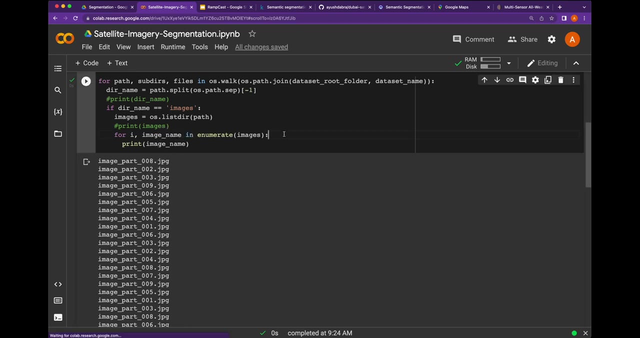 the image name. let's see now you you can get an idea that we are getting all the images individual. we do not need to see this message, and now you are getting the list of all images similar to that. if you would want to make sure that the images must be the jpeg images, then you. 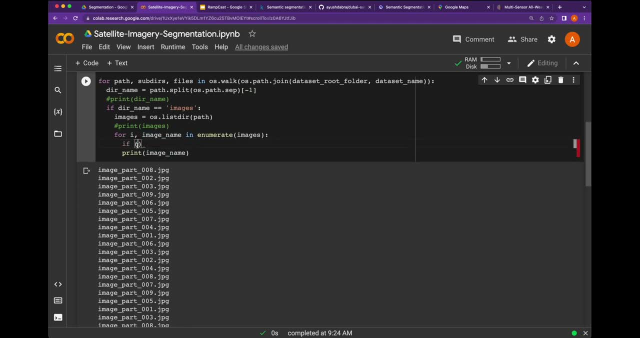 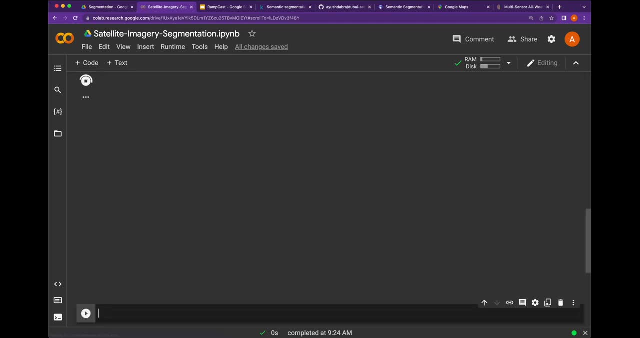 can process them. also, you could say if this image name ends with, and then you can provide your extension, so you could say jpeg, only then print the image, and that's where your images are there. however, if you will choose the directory as a masks, you will not get any images because your 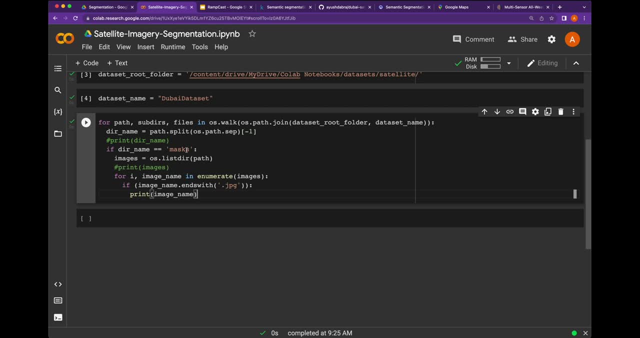 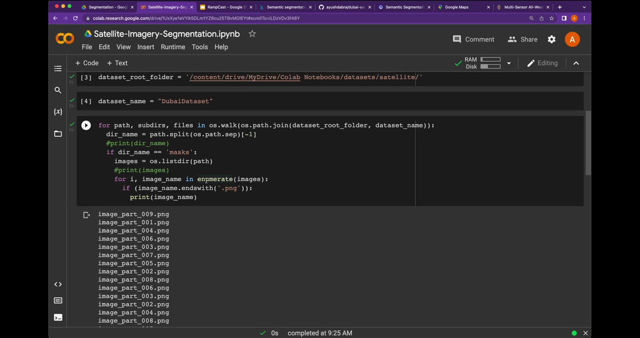 chat is dot jpeg so all the masks images are the pngs. if you change that to png you will get all the mask images. so you can get a very good idea that your source directory is the jpeg directory. so you can see that all the mask images are the png images. so if you change the disk data, 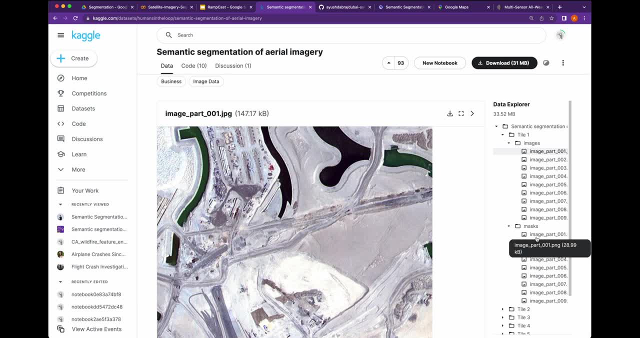 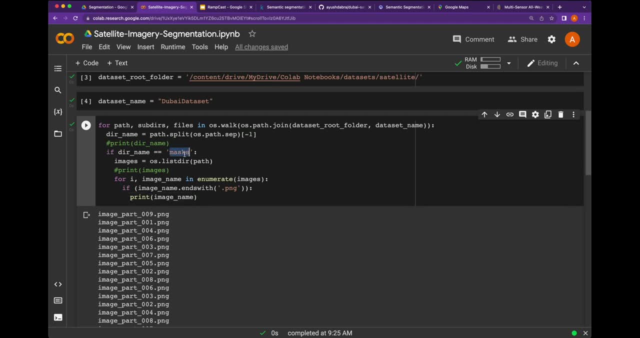 which is actually here. so the these images are, as you could see on the hover, is they are the jpeg image. the mask images are the png image. so this is how you will be able to access all of your images, whether you would want to process mask or you would want to process the jpeg, so i will. 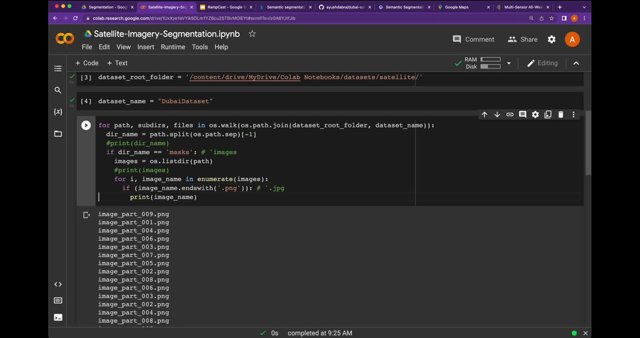 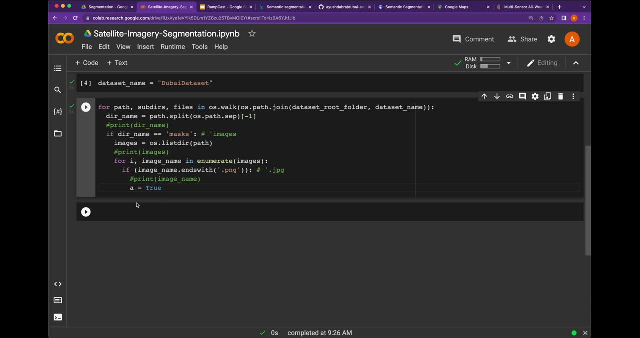 comment this area, i will say you can also use the images here and here you can also use the dot. see the output. i just want to make sure that it's easier for us to work with notebook. now, in the next step, i will show you how we are going to read these images. for reading these images, we are going 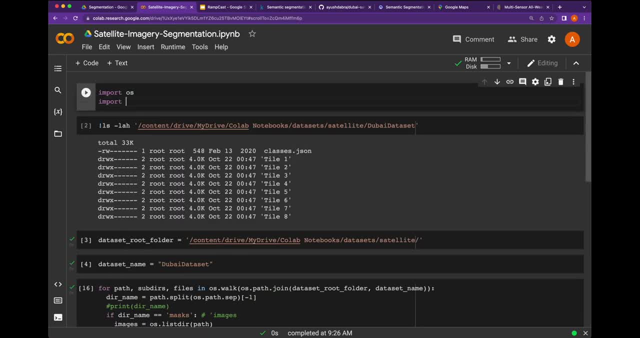 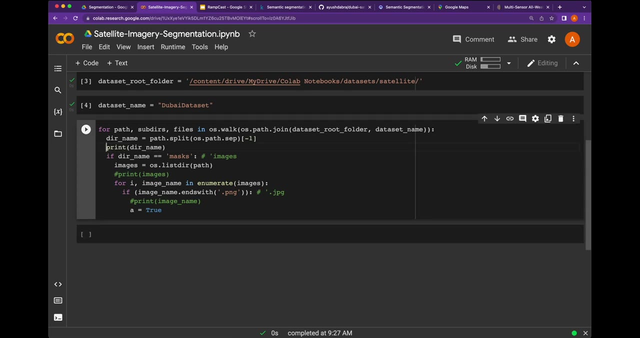 to use the opencv, so i will import here. i will say import cv2. and because we are using the google collab environment, so cv2 is already installed here, so we are importing the cv2. now we are going to read the images from the given folder. so if you look into the directory name and remember this, 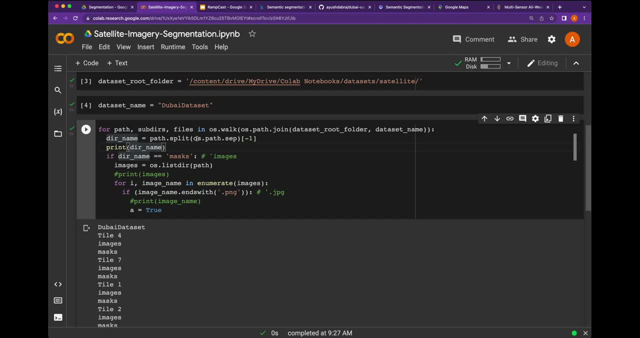 this was the directory name. however, the path which we have split completely, so, depending on whatever this folder is, the directory names are basically the tile for images mask, so we need to have that included in our path. so, for example, this path, if you will try to print the path here, 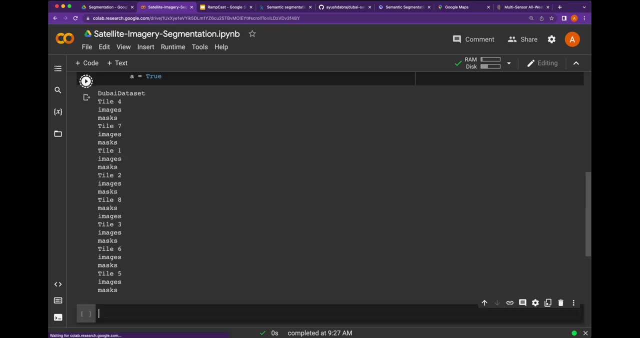 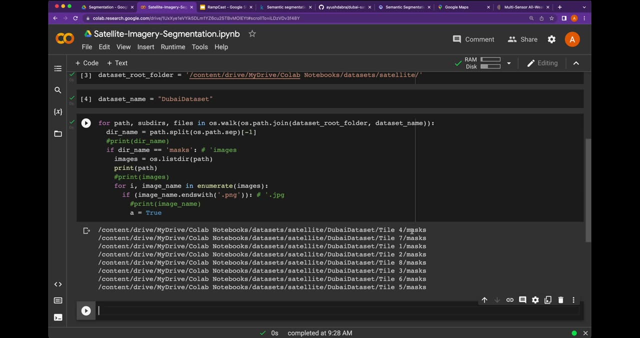 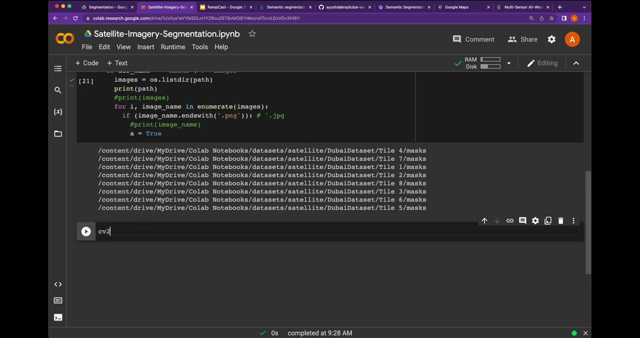 you will get. so let me comment this. and here you are getting the proper path for the, each folder which has the either mask or the images. so we are going to use this notation in order to process our data. okay, so let's use this opencv to read the image. so cv2 dot im read. so im read is our method, which is going to. 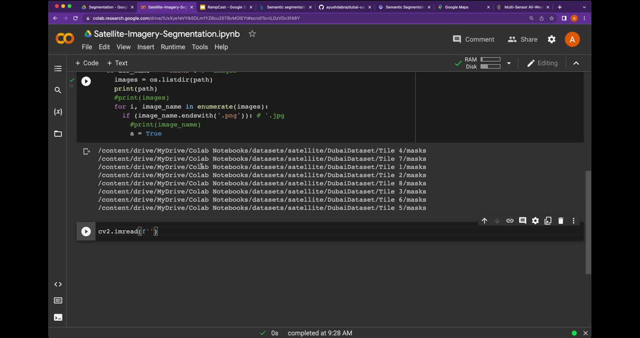 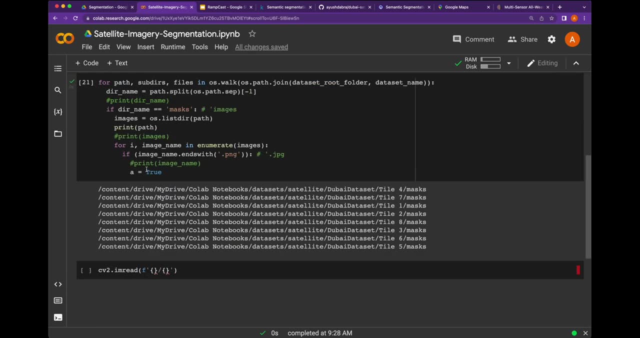 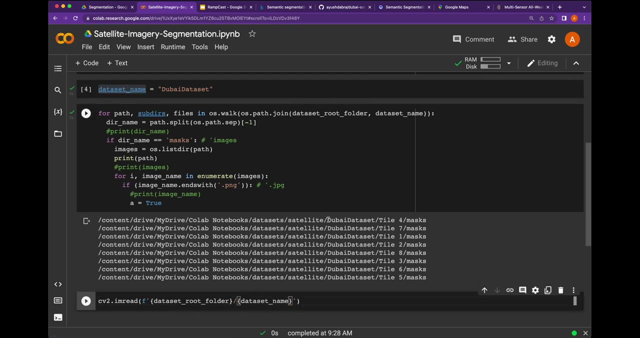 read and then here we are going to provide the path. so path will be the first. i will show you how you could create. so your path is basically the root folder, then your data set name. that's where your data set name. now you are going to say that where you are. 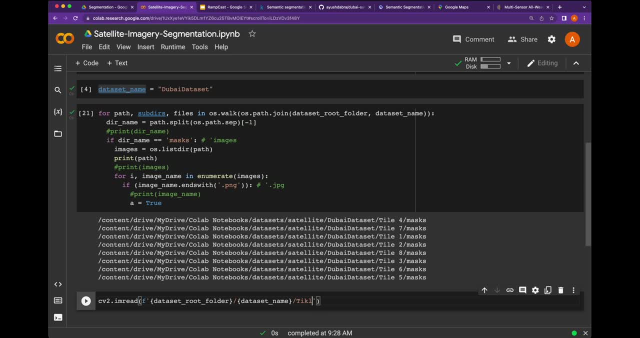 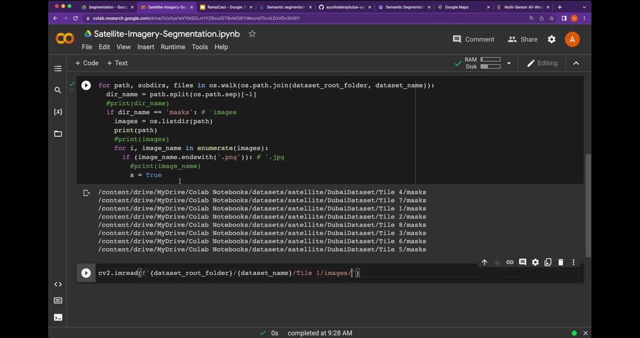 going to read the tile, so we could say, oh, let's start with the tile one. then we need to provide the images or mask, whatever is our. so that's where the images is going to come, and at this point we could actually say that what image we want. so we have already seen that. 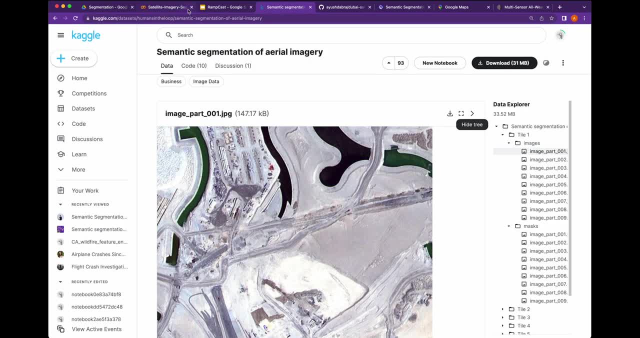 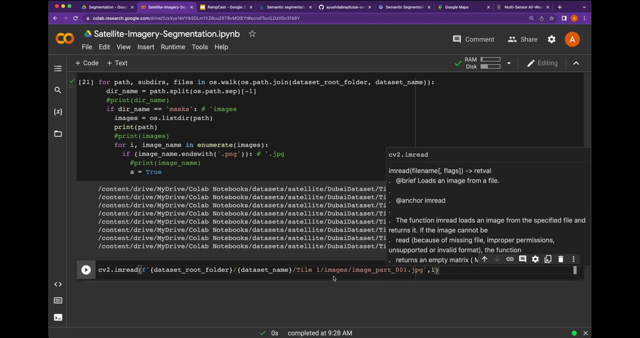 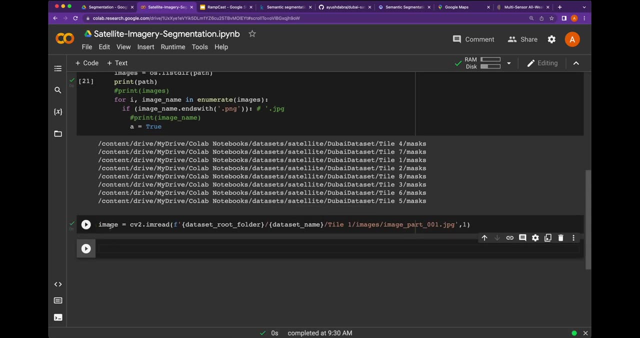 our images are the image part, then zero, zero one image part. zero, zero one dot jpeg. that's our image, comma one. so that's the image read and then we are going to read this image as a image equals. so now we have read this very first image and this image is what we have. and if we just try to, 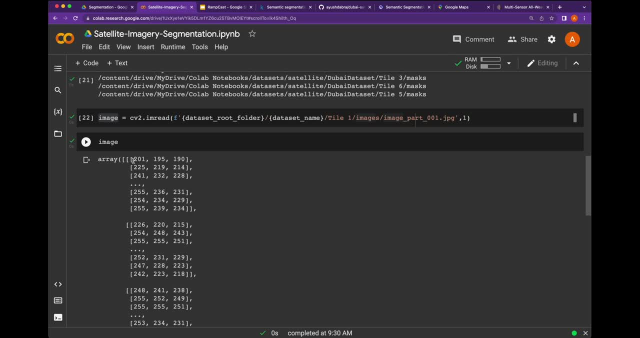 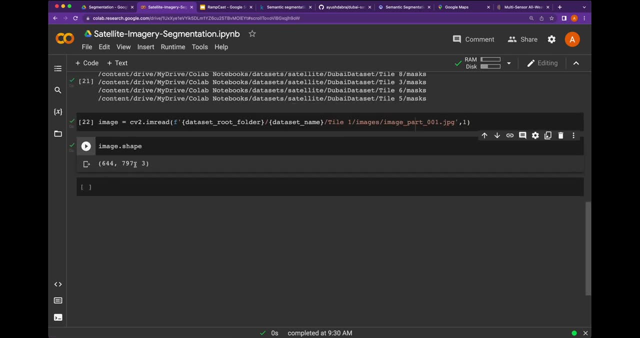 see what the image is. the image is a n dimensional array. we can check the shape. shape will tell you that the image: height, width and the color type, whether it's a grayscale or it's the rgb. this information is very important for us to go ahead and process the our. 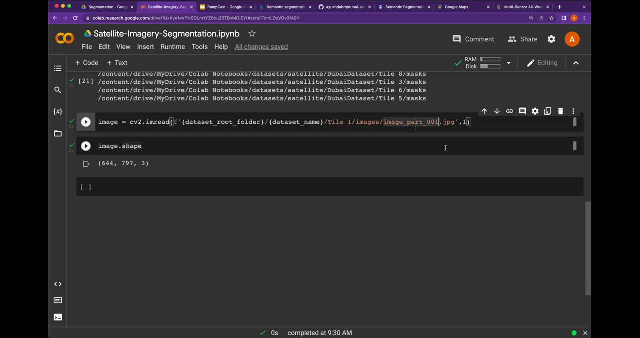 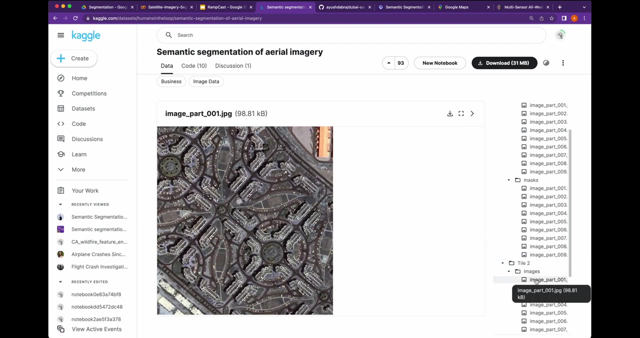 images. so, as you could see, that if we change this image to, for example, image tile1 and if we use the tile2 imagetile1 image shape change so you can get an idea that all these images are the different shapes in different folder. so we need to make sure that all of these images 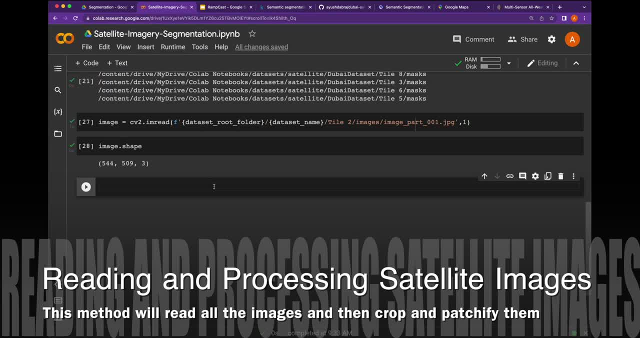 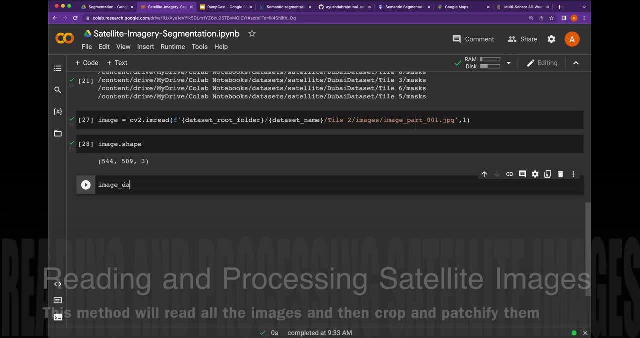 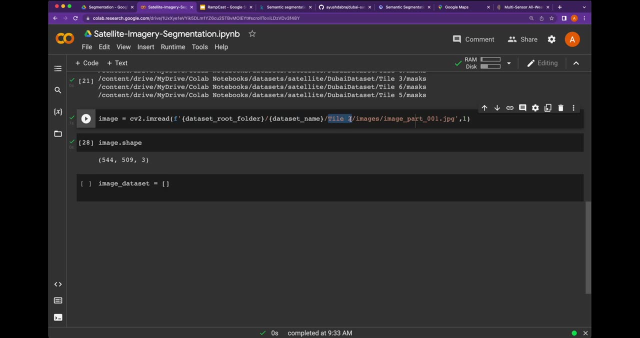 has to be uniformed. okay, so let's go ahead and start working our code where we can process all of these images. so first we need the image data set. so that's our image data set set array. as our data set is divided into the tiles folder, so we need to make sure that tile 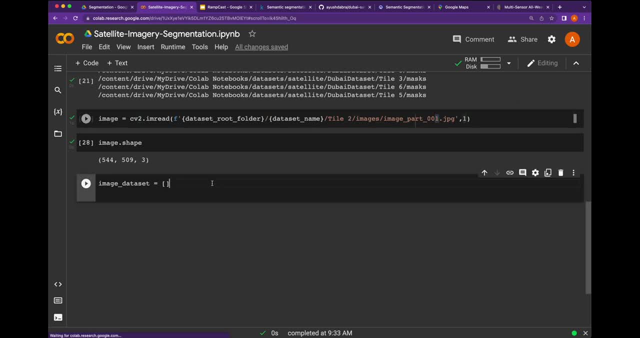 because, remember, tile has the id and image has the id. so we could say for tile id in range of tiles. so we have seen that our tiles are from one to eight. so we could say from range one to eight, and then for image, id in range one to twenty, because we have seen that how many images are. 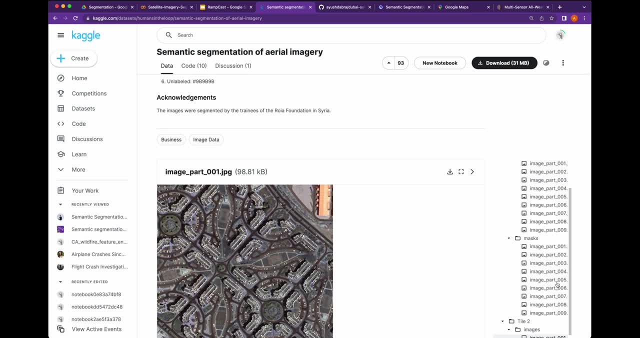 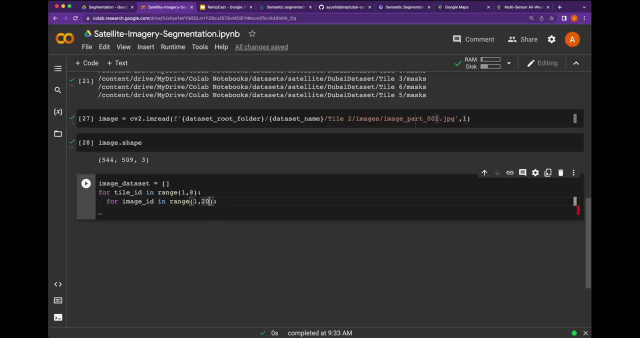 so that way we could figure it out, we could process all, almost all the images and their individual folder. so you can even say 202, because we will validate if image is there or not. now we are going to use this method, which really process our images, so here we will change. 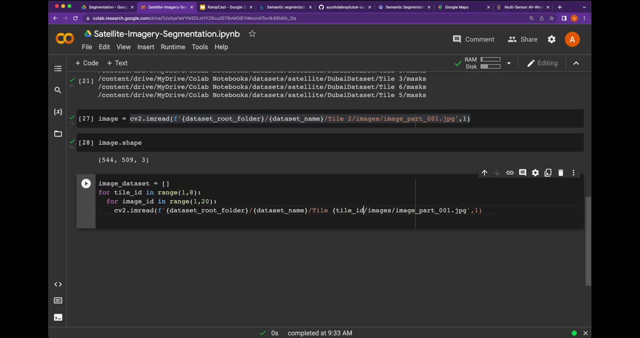 the tile number to the tile id and we will also change the image id with this number, and here we are reading the jpeg. so we could also actually set, because same method is going to use the mask as well as the images, so we can make sure that this is also changed. so here we could actually use. 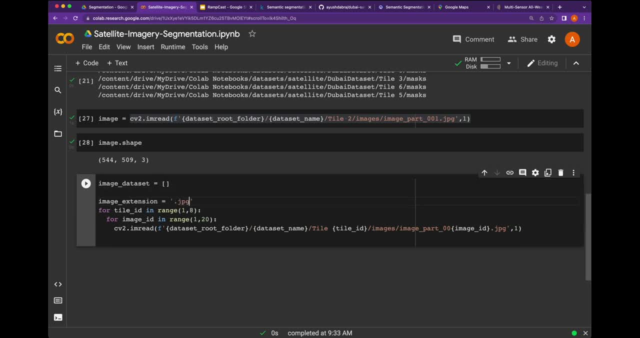 image extension is actually dot jpeg, and replace this here and remove the dot from here, because where the dot is already there. so this is how we are going to read the images. so everything what we have read is become the image here, and then we could actually print the image dot shape. so all the 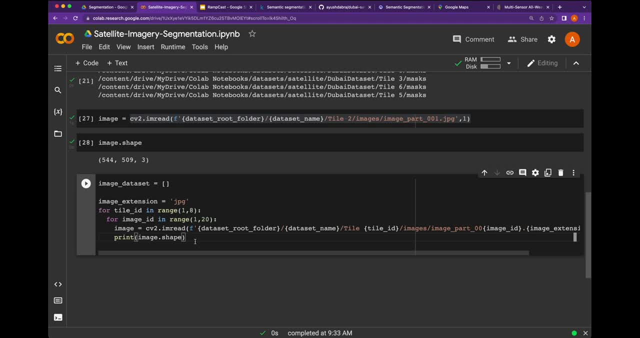 jpeg images which we are reading. we are going to get the image shape. however, we need to make sure that this image is not none, because it is very much possible that range go high and then file will not be able to read. we could say if image is not ever going to be saved. 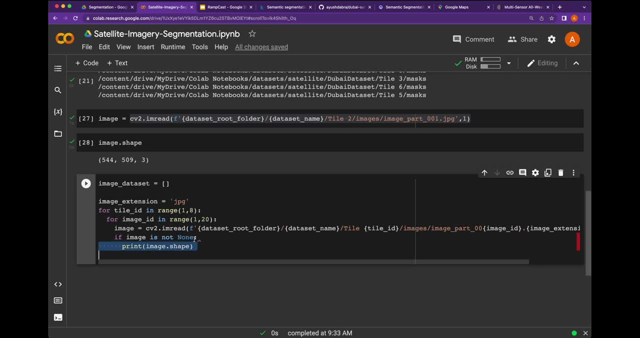 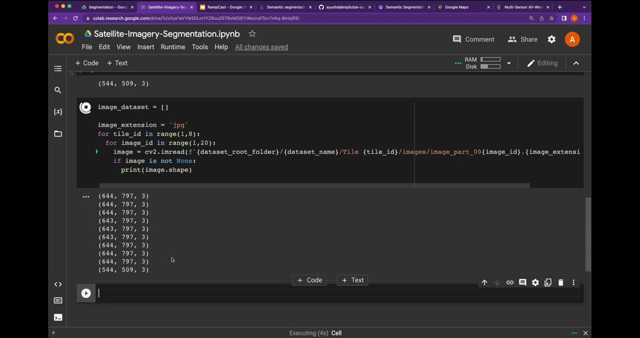 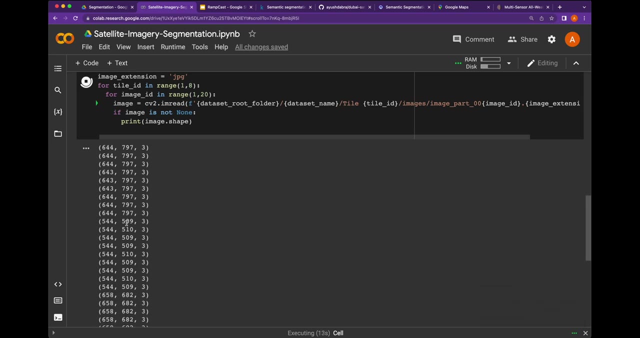 if image isienenet for a table and then file will not be able to read, we could say: if image is not not none, let's print it. you run this code, you are going to get all these images which we are reading from different places and you can get an idea that for each tile, the images, all the image. 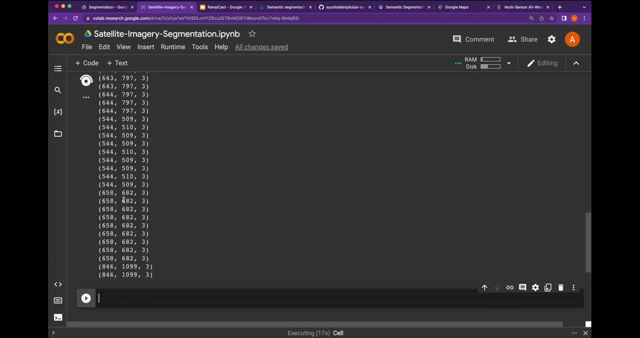 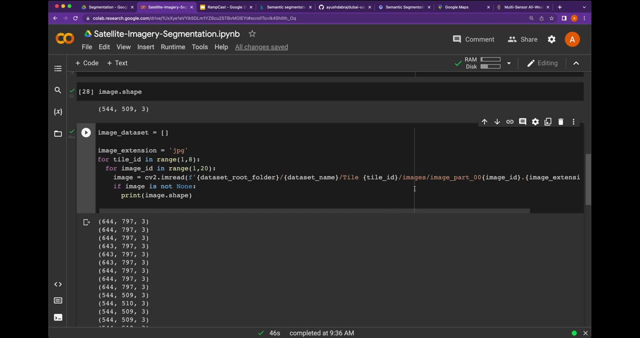 in that particular tile are same. however, the individual tile, the images, are different. now we have seen the images. if we would want to make sure that this images is also- whether it's some mask or images, so we could also say image type is equal to masks and later it can also be used as. 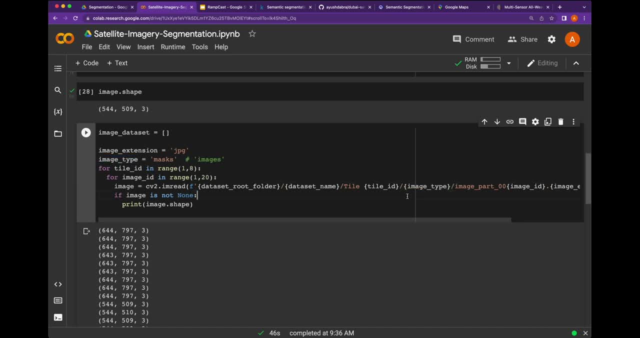 images. and now we could use image type here, because the image part between the images and between the mask is does not really change, so this part will still going to be the same. so, and here it can also be the png. so if you would want to check the mask, we will also going to see. 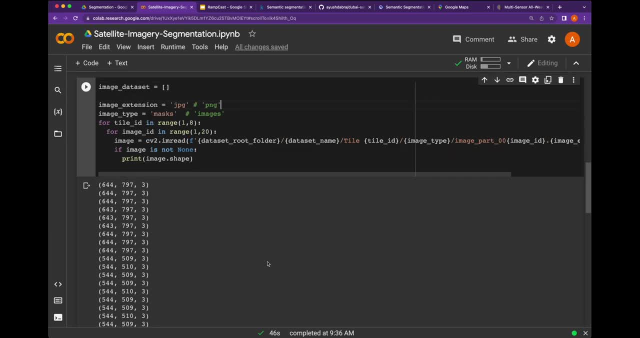 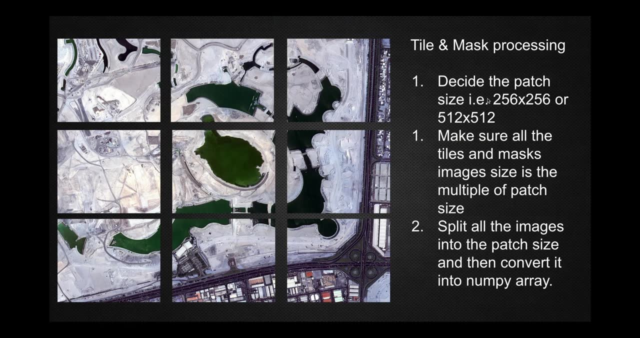 that everything is going to be the same. now it's time for us to understand the patching of our image. so remember, we talk about that. we need to decide the patch and then we need to make sure that we could. all the images are the multiple of the patch size. so that is what we are going to. 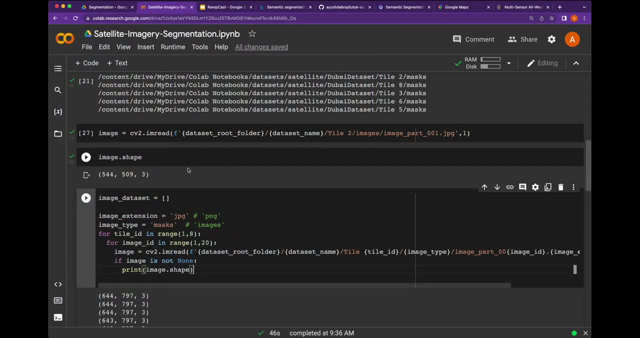 apply in our source data. so one thing: i just wanted to show you that right here, we are going to apply the patch size. so we are going to apply the patch size. so now you see that the image which we are reading here is five, four, four by five, four, nine. so we need 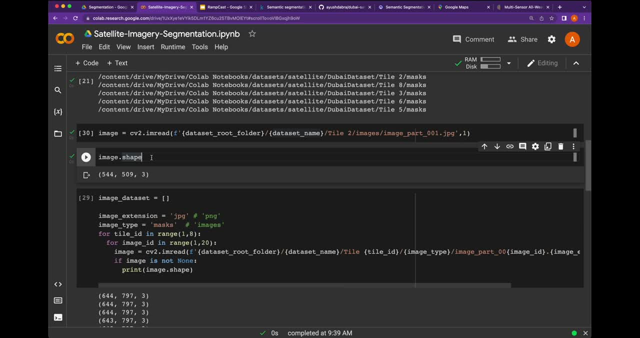 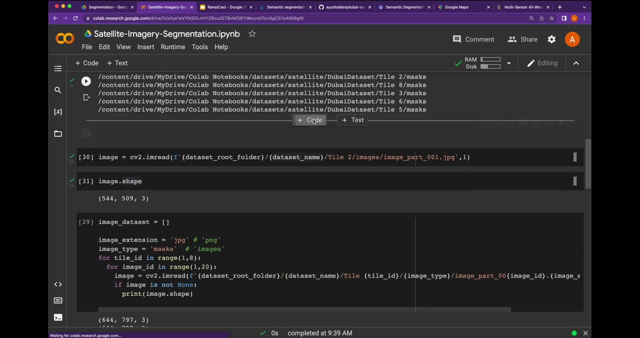 to make sure that this image shape is going to be the multiple of our patch image. so let's define our patch size. so our image patch size is 256. that is our patch size. now we can take this image, which is our five four, four, by five four, four, which is very different: the multiple. 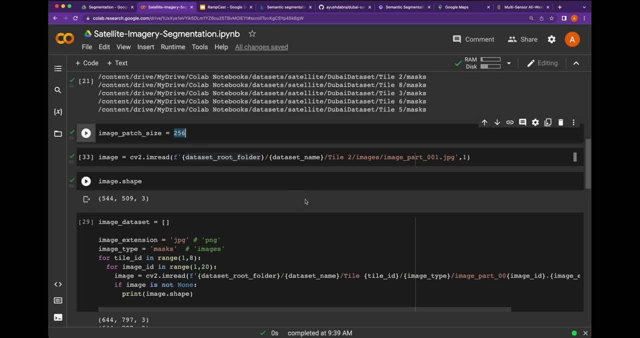 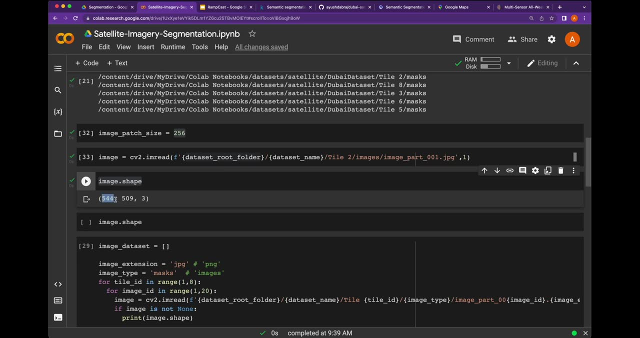 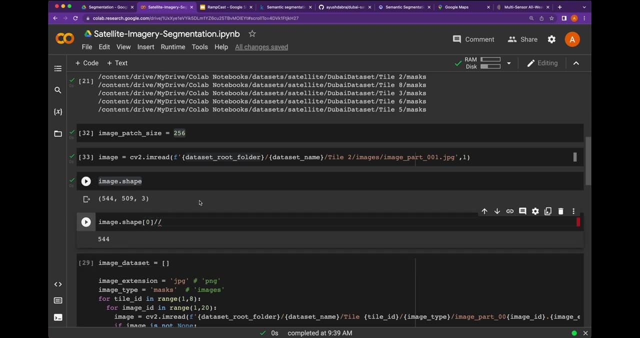 of 256. so in order to perform the patching, we can generate this quick method. so here we take this image shape which has image shape of zero. you can get the five, four, four value. you can actually mod it with our patch size. so our patch size is 256. it will tell you that the in the multiples 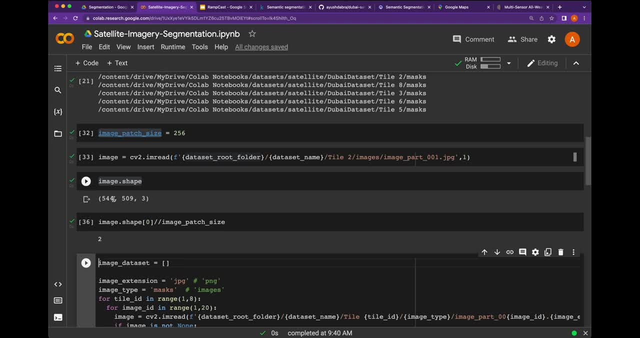 it's only two times 256 times 256, which is 512. and third will not be applied. so we can get an idea that how we can make sure the patch size work. then we can take this whole result and we can multiply this whole thing with the patch size. so we will get that in this case. 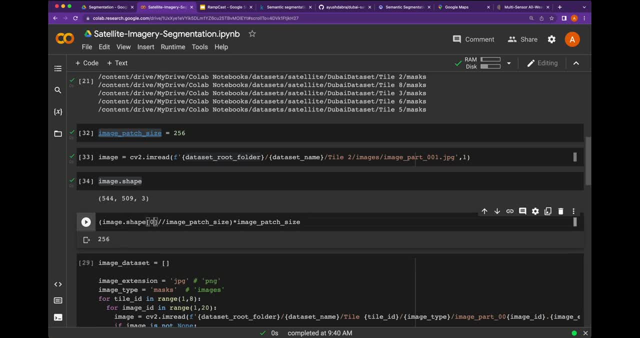 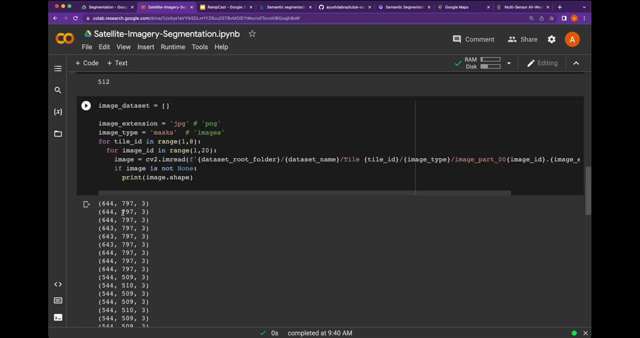 the multiple will be 256. in in this case of 0, the multiple will be 512, so all the images will have the multiple of image patch size and the multiple will be 512, so the multiple of image patch size what we are looking for. so the x will be this value and y will be this value, so we could. 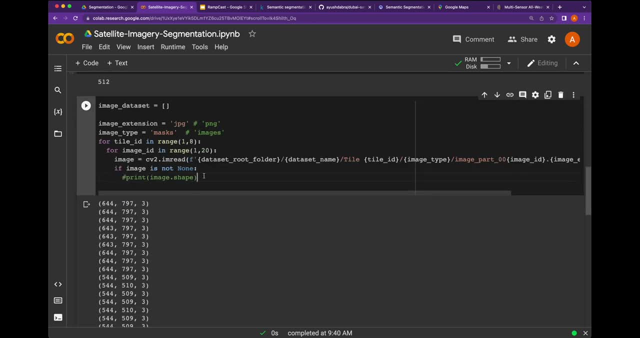 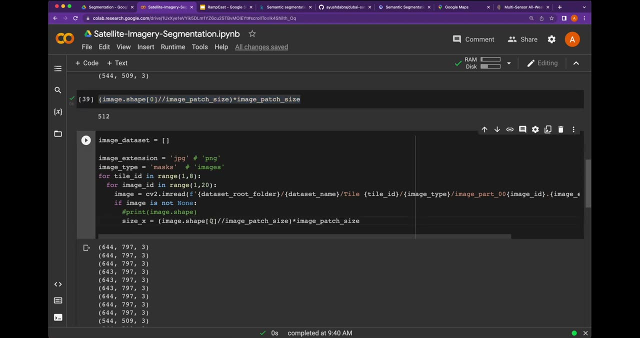 actually define that here. we could say: the size of x is- we take this whole value and we need to make sure this is one, and the size of y is the zero value and patch size. so this is how we are going to get the x and y for each of these values. so we are going to take this whole value and we 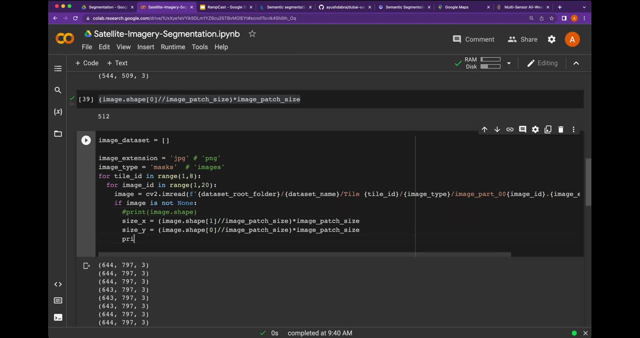 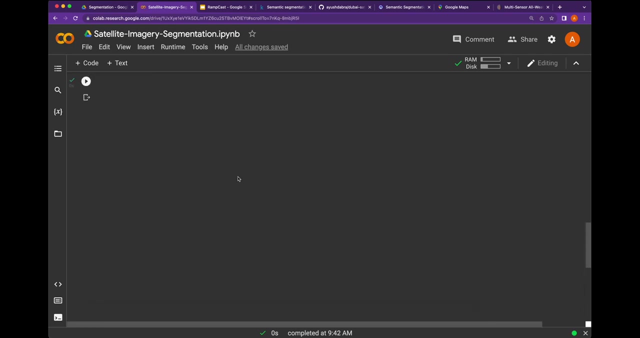 can take print, and here you could say format: size x, size y, and at the same time, if you would want to print the image shape, you could actually print the image shape also, so you have better idea that how the adjustment is going to happen. let's run this code. so we are reading the mask, so we need to make 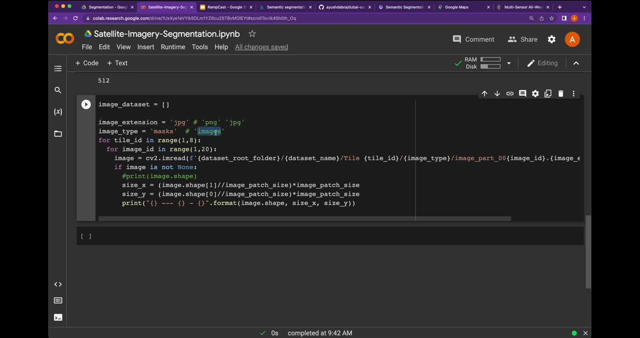 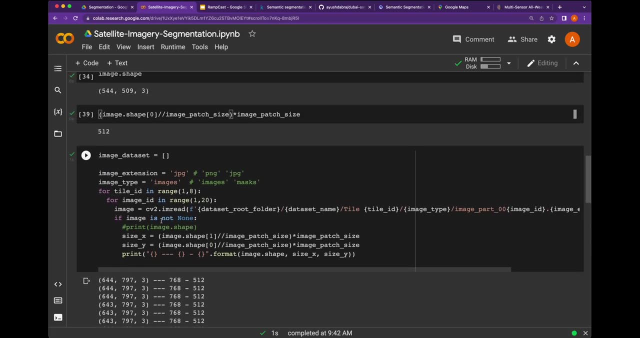 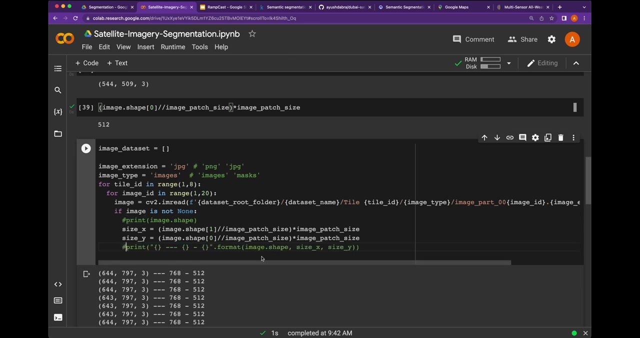 sure that the value is png, so let's make sure this is the images and jpeg. you could see that how these values are being adjusted in the multiples of 256 by 256. let's comment this line. go next. now we are going to convert this image, which we have actually, if 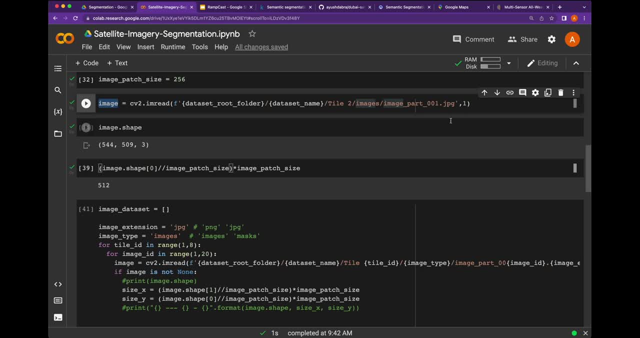 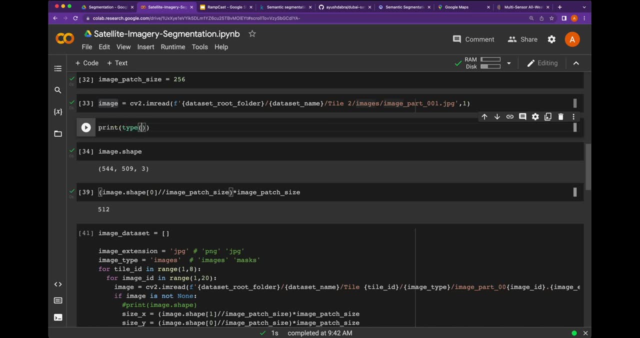 you would want to really understand what is this image when we are reading. you can actually come here and you can say: this is the image which we are reading. so we can actually come here and we can say: give me the type of this image. you can say: print the type of image. you can get an idea. 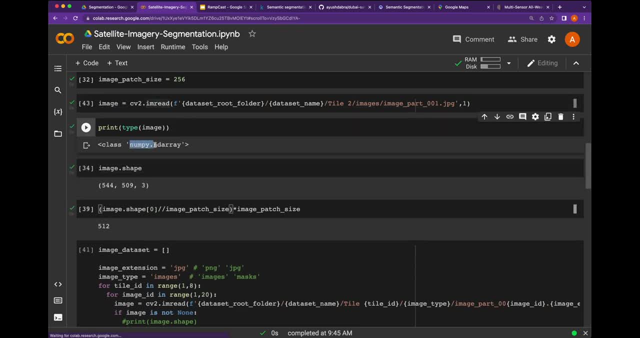 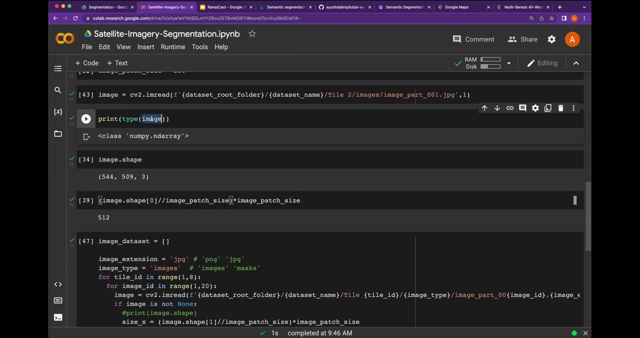 let me read it. so this is the numpy nd array. whenever this im read is reading this image. this is the numpy nd array, as you could see that this image is actually the numpy image, so we need to convert this image to the image type so we can use the image library, which is from the 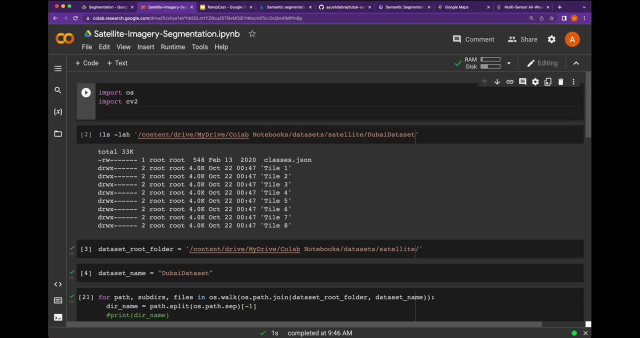 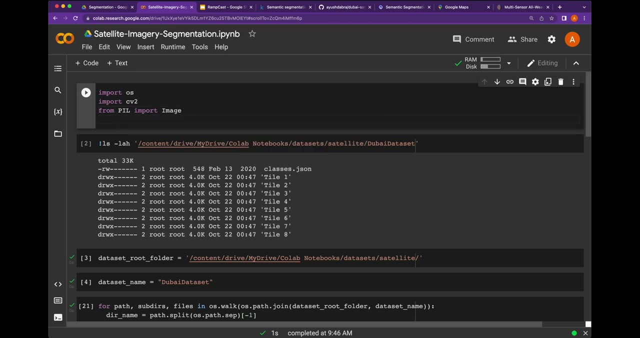 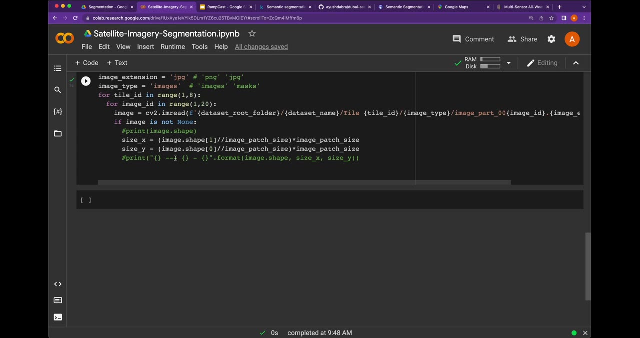 philoh. so let's use the philoh library here. so from pil import image, and when we are importing image we can also say import numpy as np, because sooner later we need to use the numpy too. we could say so here. i just wanted to show you what is the process we are trying to do here. so 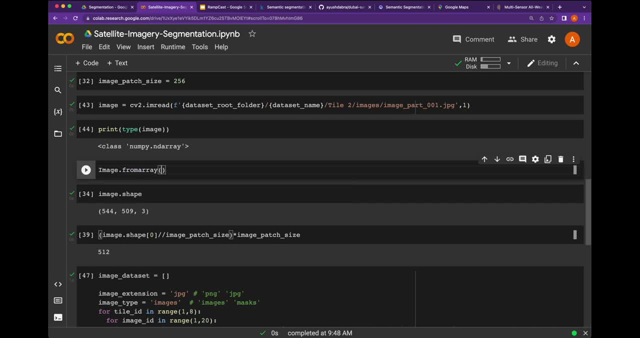 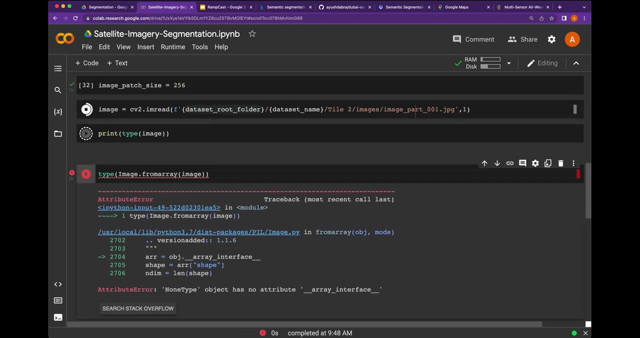 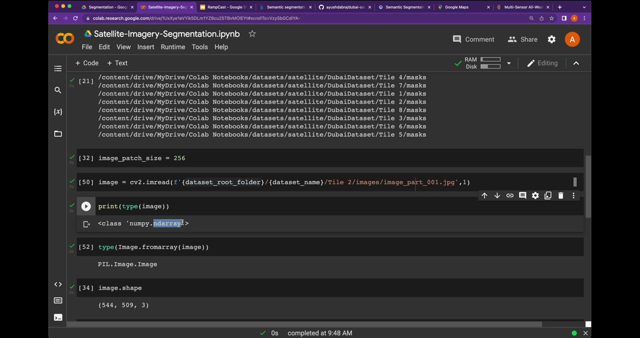 we can say image dot from array and we can take this image. If we take this image and we can say what will be the type of this output, Let me run this code first Down here. So this will become the image. so which image? which was the nd array? now, 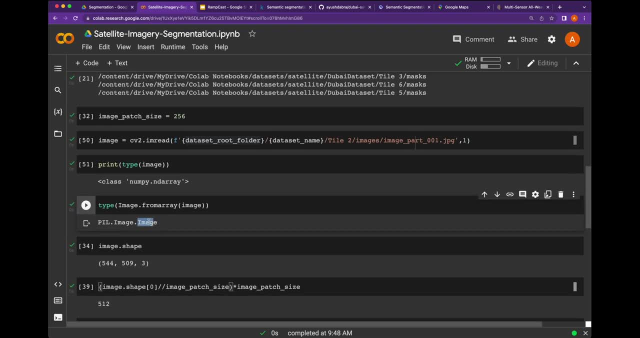 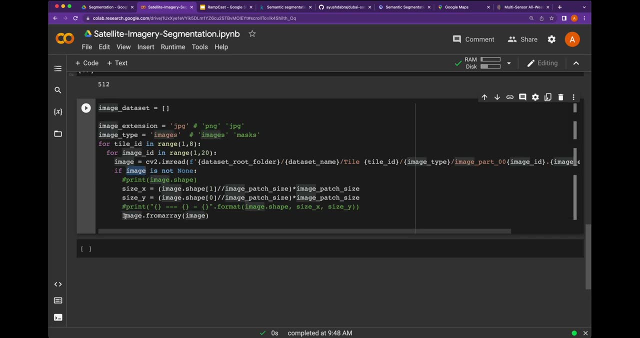 It's became the image type, because now you could process this image whatever size you would want to change it. So we are going to take this code here and we will convert that back to image. So now our image from the array became back to image. now, at this point, 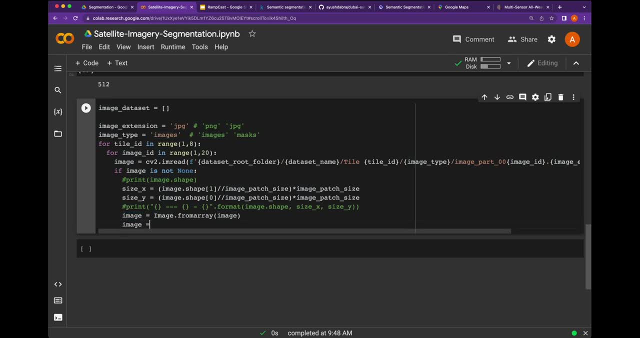 we could actually crop the image. so we could say: the result image is going to image dot crop, and Here we could provide the size which we are looking into. so 0 comma, 0 comma, We can say what is our size X and what is our size Y. That's what we want to. 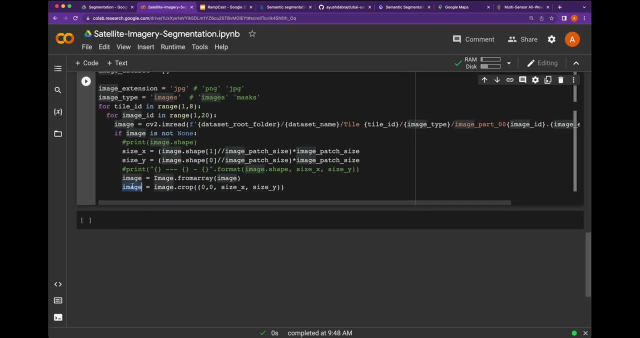 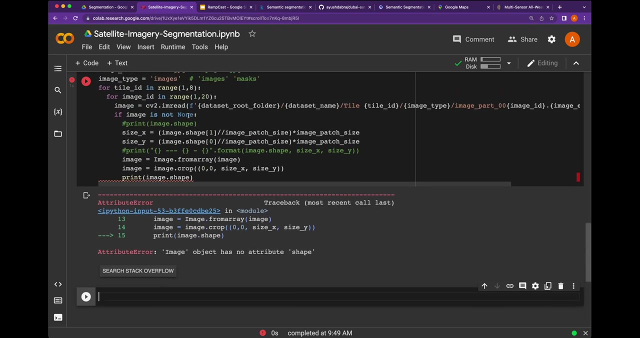 Crop it and at this point if you would actually get this shape of image, That's. Let me Show you. there is a trick. so if we try to come here and say what is the image shape, you are going to Get an error because the image is no longer the array, because array has the shape, not the image object. 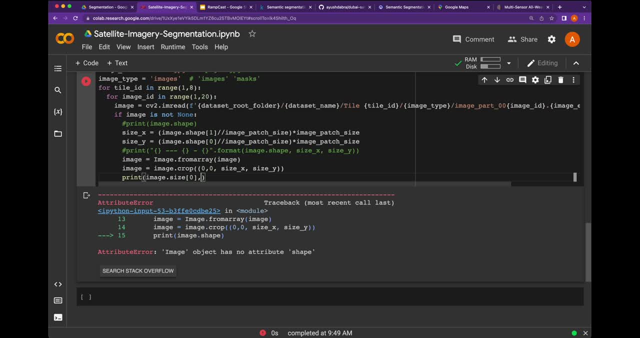 So actually you could use the image size 0 and the image size 1, because image size 0 and 1 is going to tell you the image size. so you could say The output is going to be format here. You could say: you want to print. 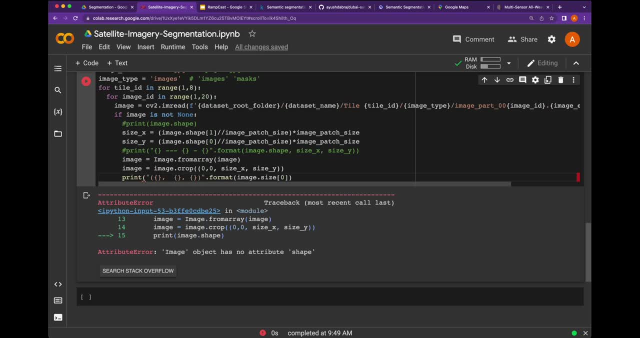 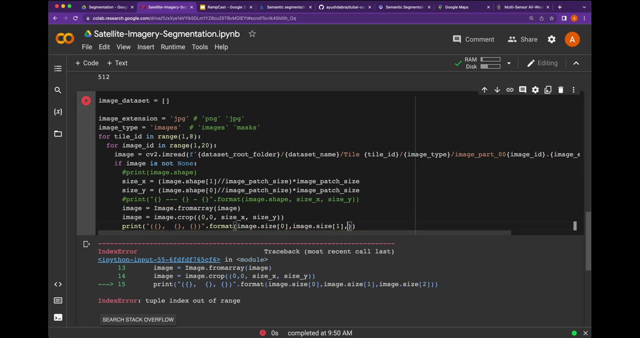 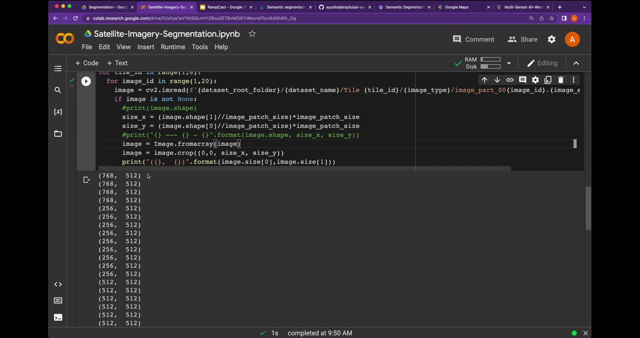 first comma, second comma, third, and here it's going to be the image size of 0, 1 and the 2. Okay, there are two parentheses. Take so the output of this image object has these two values, 0 and 1, and now we can get an. 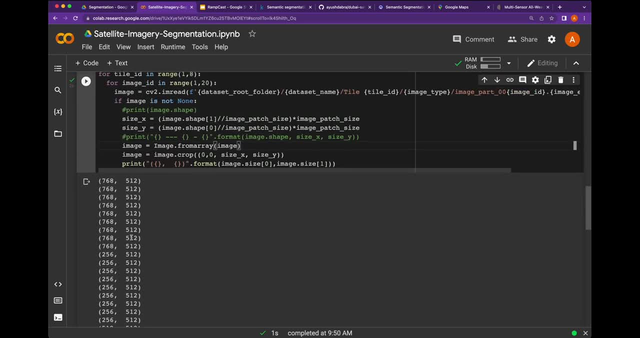 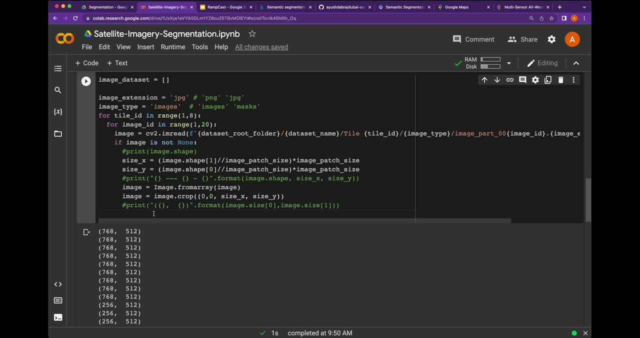 Idea that all of our images are cropped based on multiple of our image patch size. So the cropping has been done. after the image has been cropped, now We need to go back and make sure that all of these images- So we need to patch them, based on the multiple of 256 by 256, what which is our batch size. 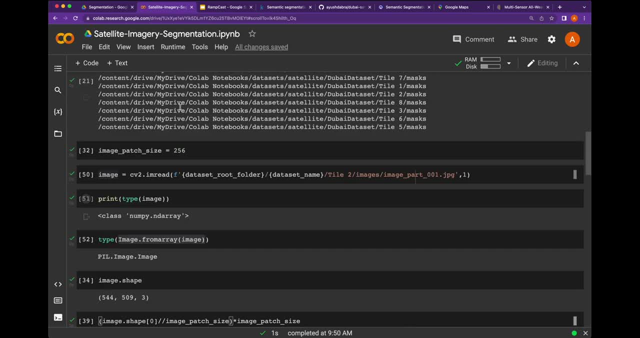 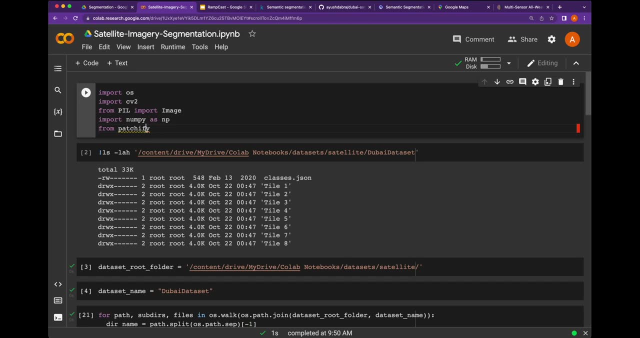 So we are going to use a library called the patch. if I, Let's come back here. We can say: from patch if I import, so patch if I is Not there, so we can go ahead and we can install it. pip install patch, if I. okay, this is installed now. 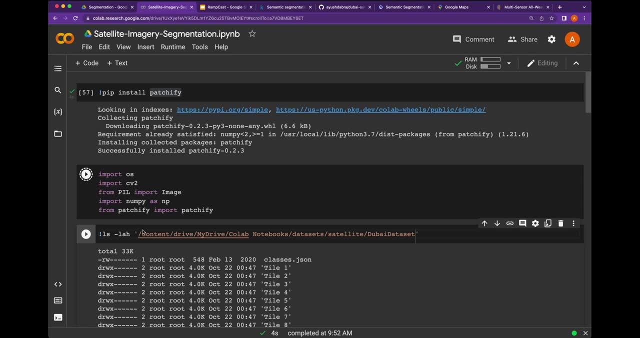 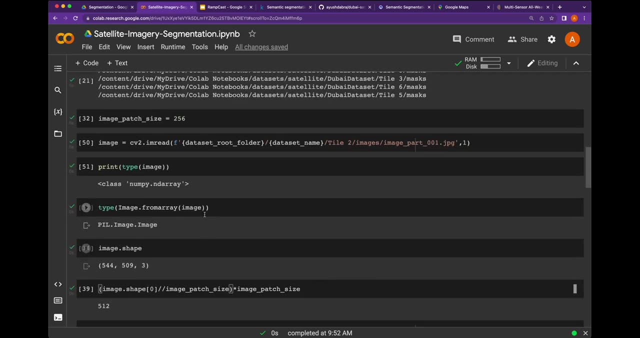 We do not have this warning Import patch if I, so now we can have access to patch. if I, let's take a look what this patch if I does. So remember, this is what our image, which we are reading, so I can actually show you the patch if occasions. 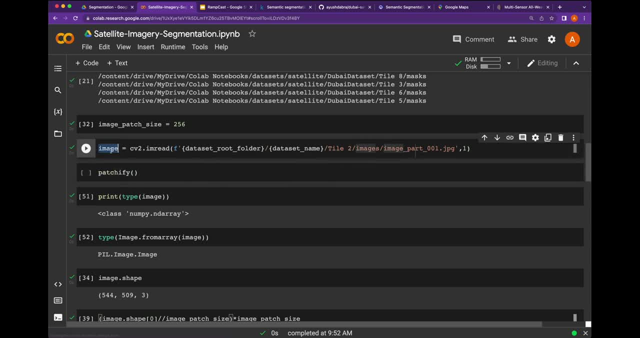 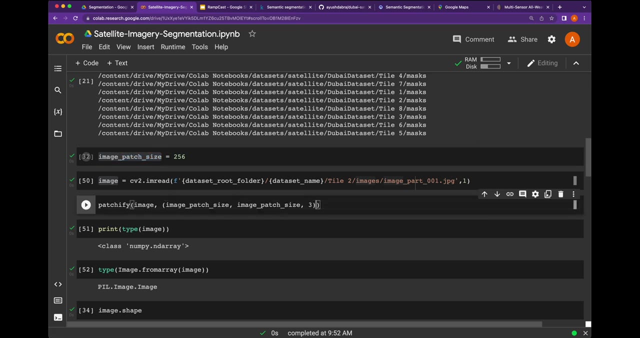 So the patch, if I it takes the image, so you can take this image and you can patch it So you could provide whatever your image patch size You would want to use. so our image patch size is going to be The image patch size X, image patch size wise, and the color, so three colors. 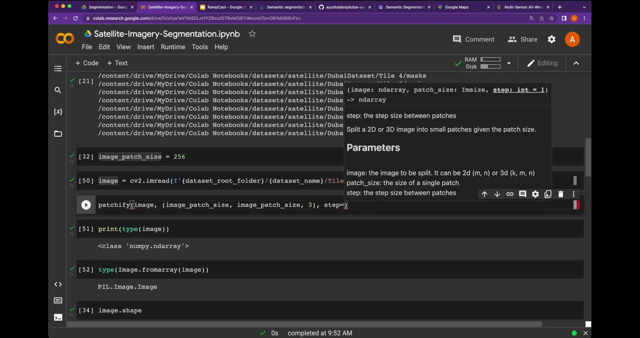 So the steps is going to be these steps, if the step will be the same as image patch size, So the create the patches of size 256 and that we call them image patches. so let's Image patches. so let's read the image: create the image patches. 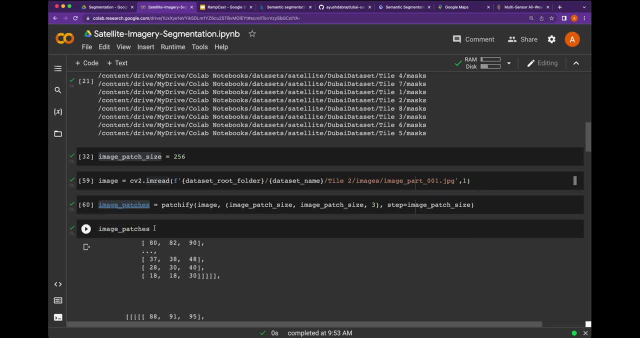 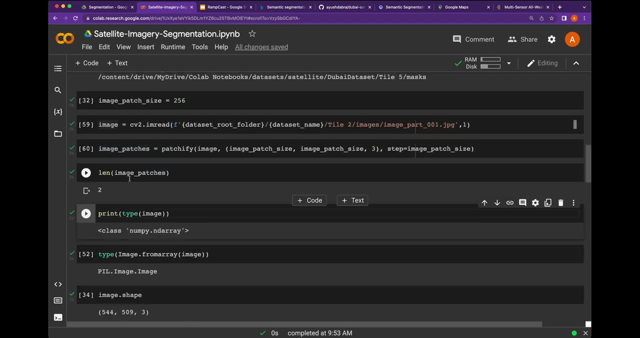 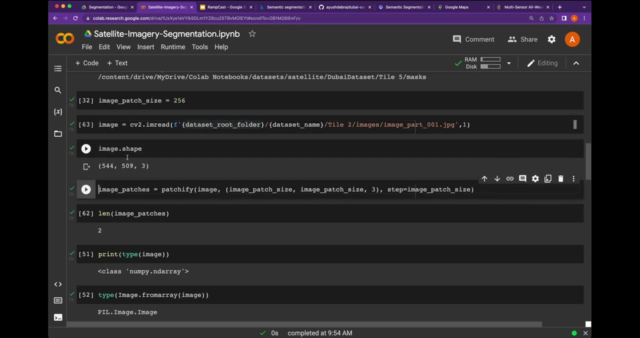 and if you look into the Image patches here, that is basically the various images of different patches, And if we say what is the length of patch, the two patches. so, based on this image shape, let's read: This image shape is 544 by 509. So once we have cropped this image properly, 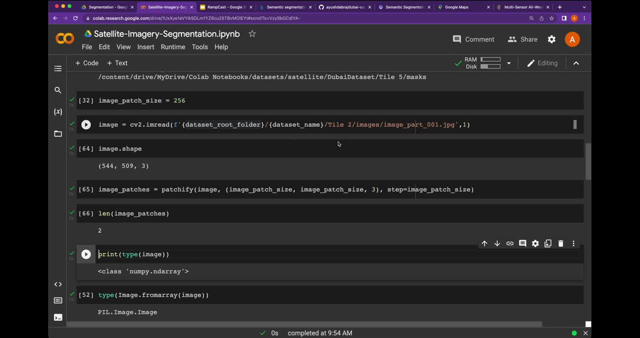 The patches is going to have the two image. if you will change for this to something else, then you will get the different number of patches. So this is the patch if acation code which we are going to use and At this point the image input image is actually the numpy array. 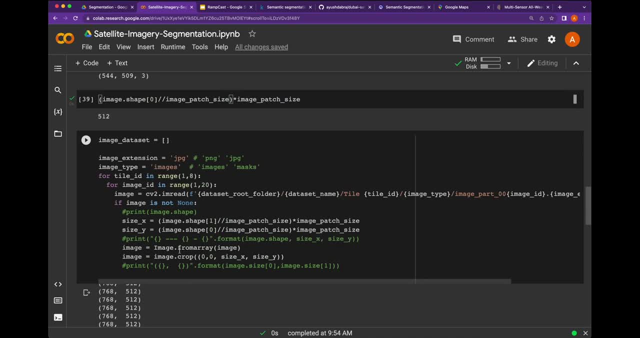 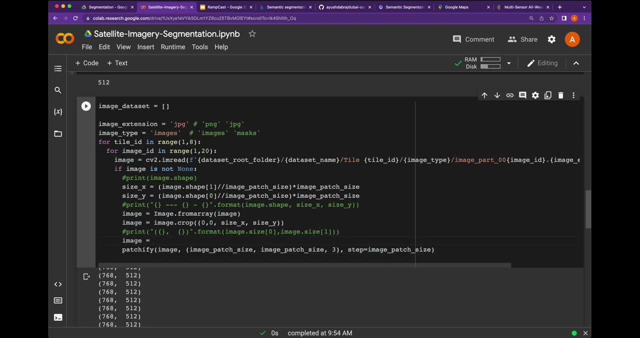 So it takes the numpy array- because that is what's C V to read. So if we come back here and if we would want to apply the patch, We need to make sure that this input image is back to numpy array. So we need to convert this to numpy array. 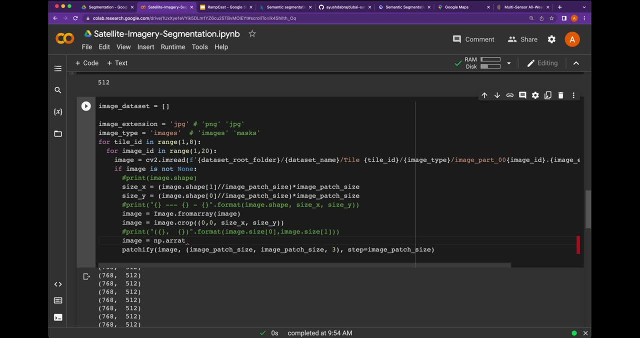 So that's where we will do NP dot array and We are going to put the image back here. So here we took image convert back to Image type which is below image type. we could crop it and putting back to numpy array, And now that will be going to be used as the input for patch if acation, and here we could generate all. 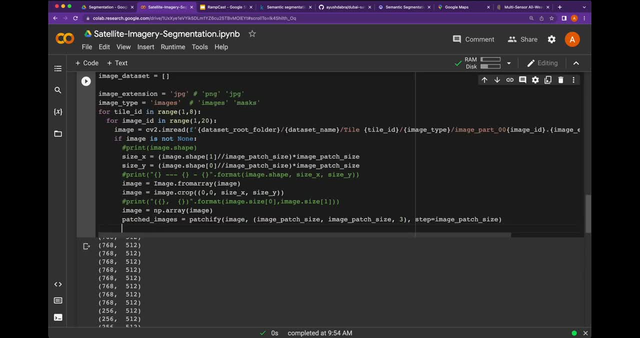 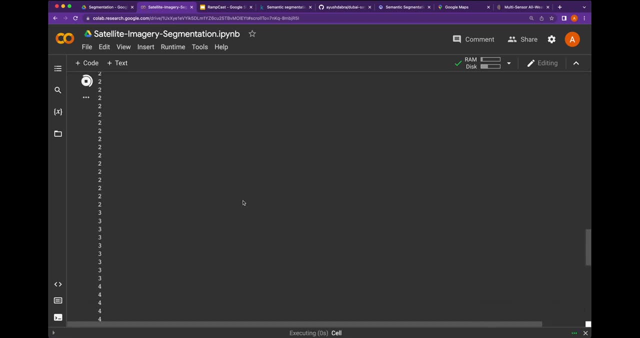 Patch images. That's where we get the patch, if I know. if you say, print the length of patched images from this code, Now you are going to get an idea that how many patched images are Generated based on each input. so here: 8 patch images 3. patched images 4. 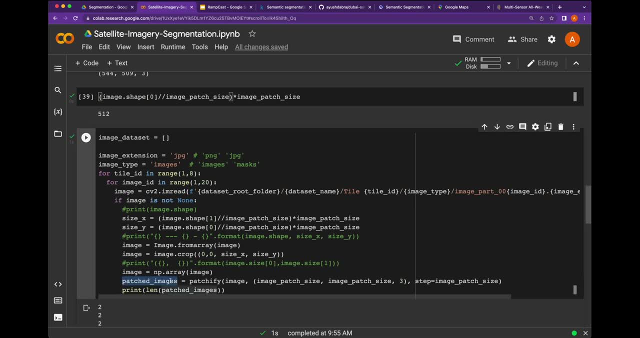 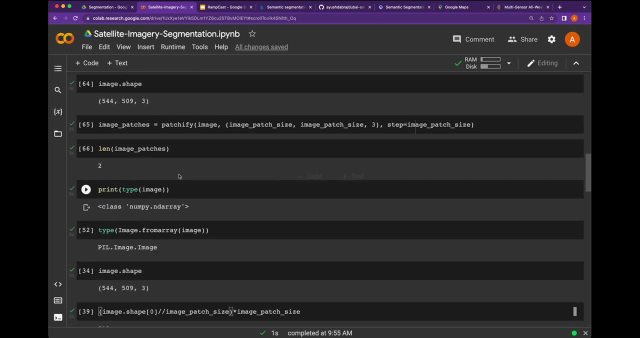 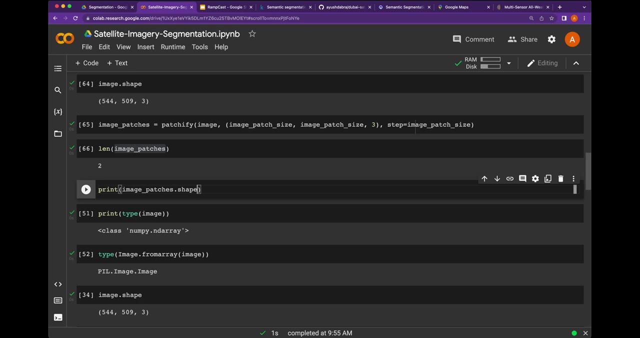 So you can get an idea how this patch, image or a is working. Not only that: if you, if you could print the patched image is size, you can get the patch, the image. So let me show you here That. here is your Image patch. and if you would want to print image patch dot shape, let me read the image first. So there are. 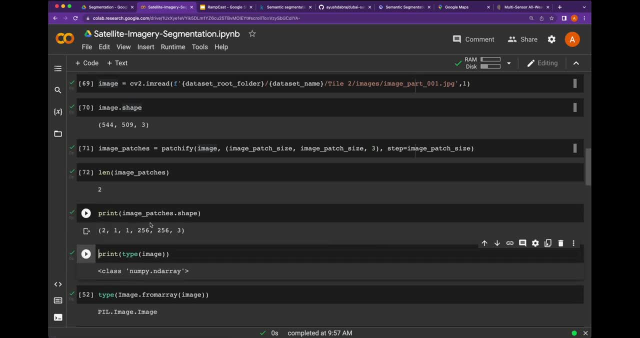 two patches shapeي shape. you can get 2 of 1, 1, 256, 256. so this is the batch image, so you can get an idea that this is the shape. and if you would say what is the shape of 0? this? what is the shape of 1 is 1. 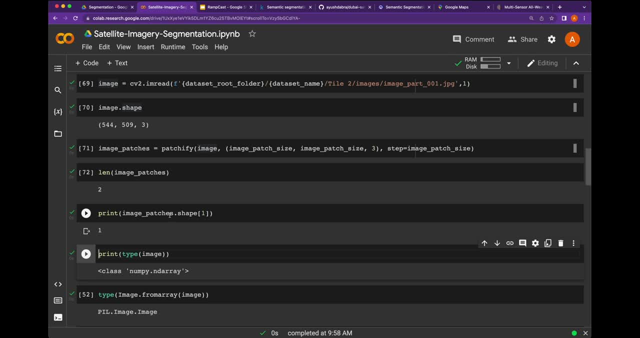 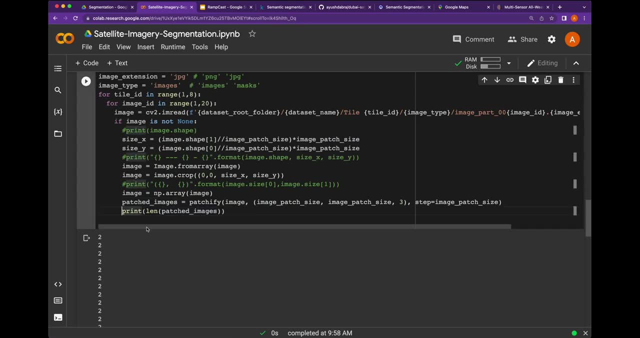 so, for all the images we have in the patches we need to enumerate, for the patch 0 shape and patch 1 shape. let's come back here, comment this line and we can say, for i in range of patched images, dot shape 0 and for j in range of patched images. this everything. however, we are going to use the 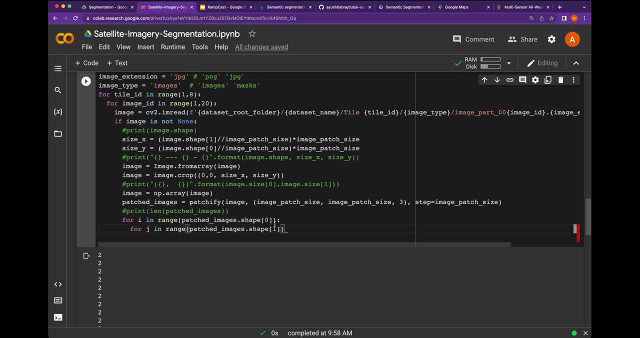 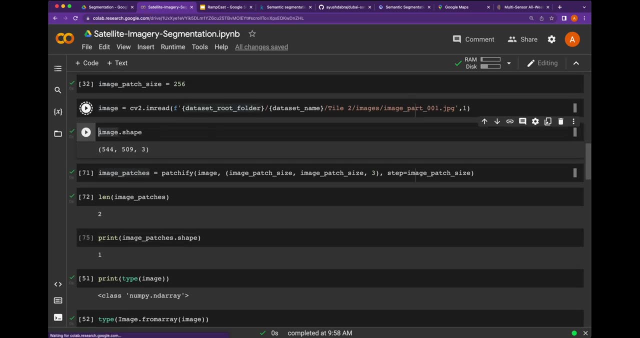 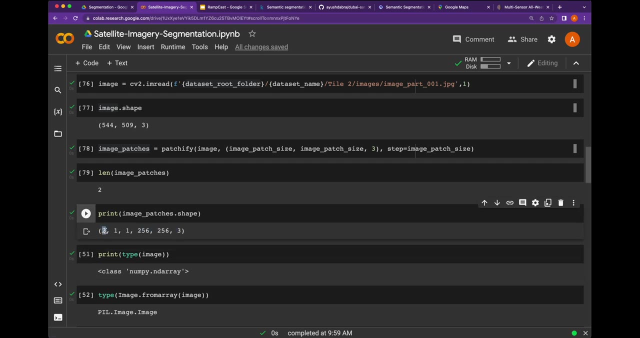 1, and that's where we will be able to get the patched images out. remember when we were processing here shape? let me read: so you see, we want to get this image out, so we need to get from this this triangle, and then that's where we are going to get these images. then we will remove this one out and that's how. 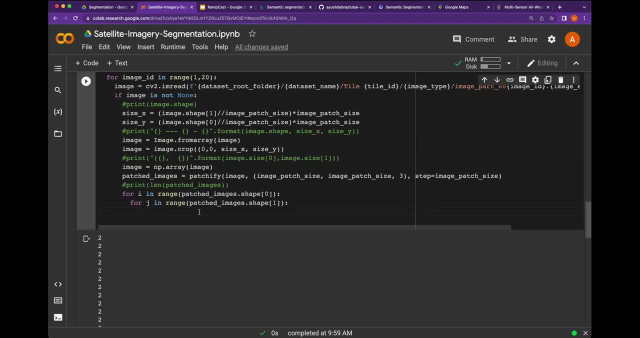 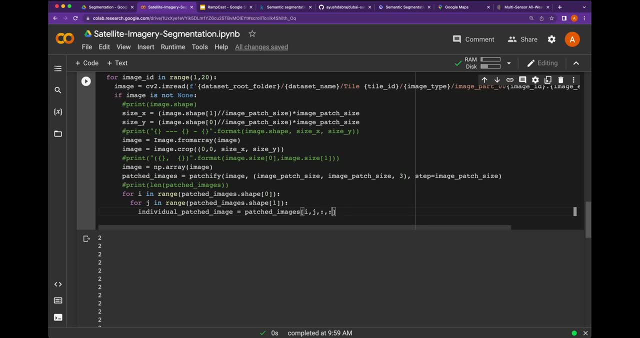 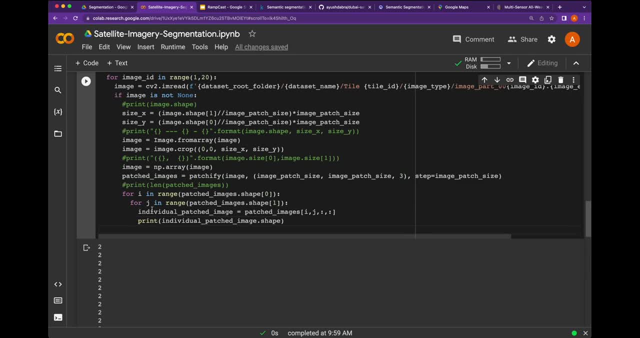 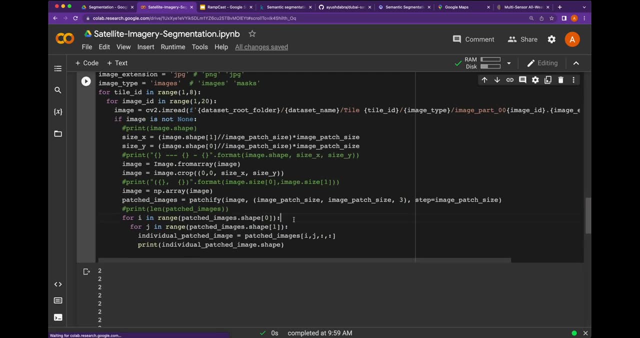 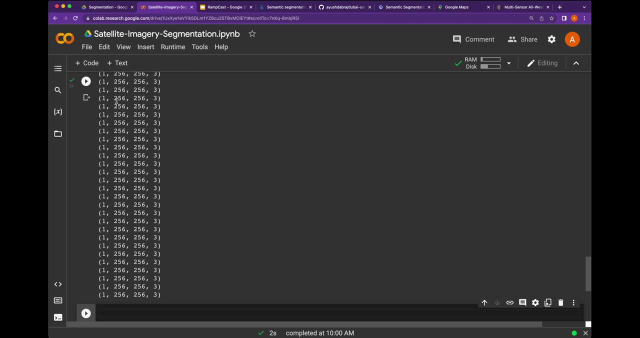 patch image and if we take this individual patch image and we can get the shape of it, that's what you are going to get, what you are getting out from that output. we supposed to get this output from each image. as you could see, everything is same. getting all of these images of size one of two, five, six, two, five, six and three. so one thing you. 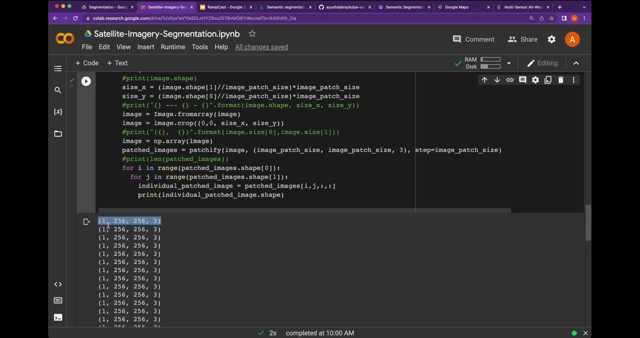 figured it out that this image is actually transformed into the array of one colon, then image size. so now we need to actually perform the min max scalar. let's take a look from sk learn or the scikit-learn library. there is a method called min max scalar. so using min max scalar, we are 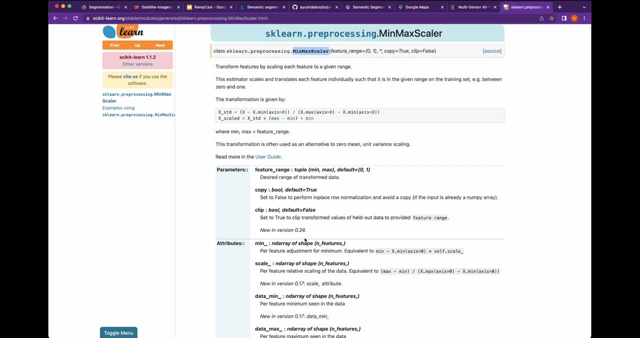 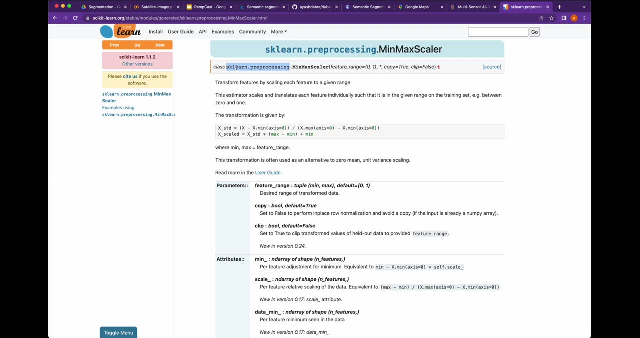 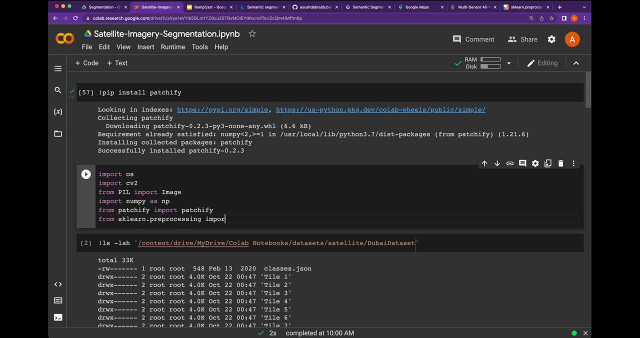 going to convert every pixel value between 0 and 1.. so it's a normalization of our input data. so we are going to import this min max scalar method from the sklearn preprocessing. let's go top: from sklearn preprocessing, import min max scalar and we can also actually take the standard scalar. 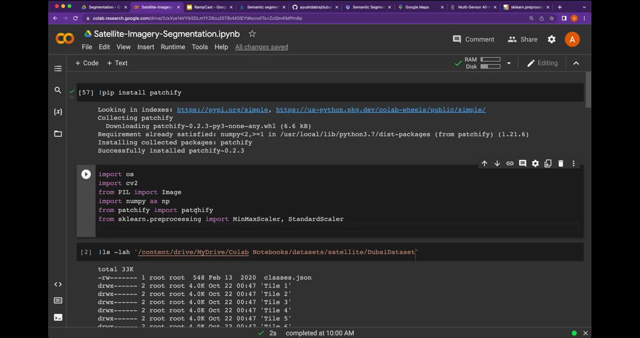 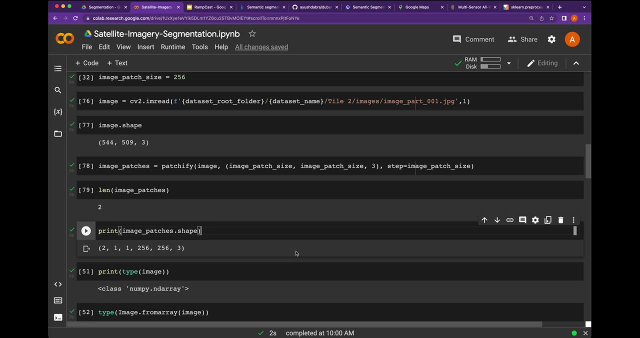 so we have these two scalars available, available with the scikit-learn preprocessing and if we take this min max scalar and we process our image here. so first let me keep it here. now we are here, so our image size is this, so we will take this image. 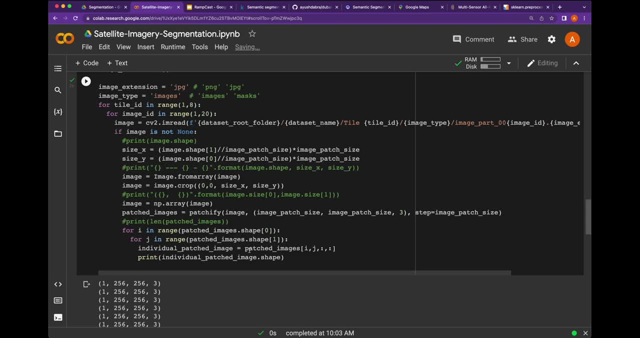 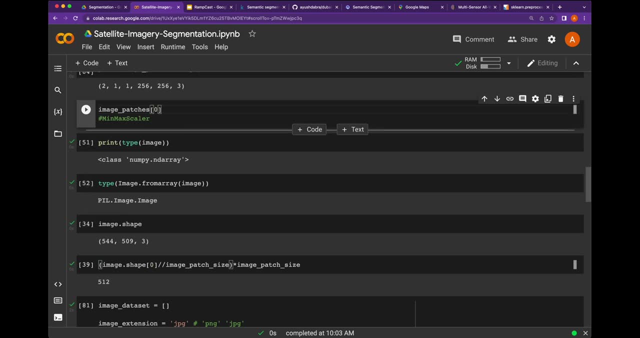 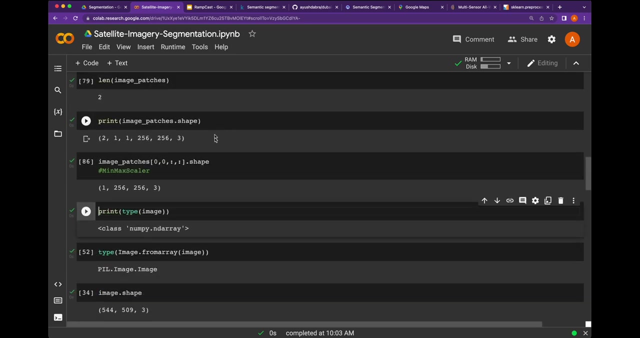 patch and remember, we have already take the patch image of zero, zero, colon, colon. so we can take here zero, comma, zero, comma, colon, comma, colon. and that is the image we have taken and if you look into the shape of it you are getting the one of 256, 256, of three, so okay, and then this will: 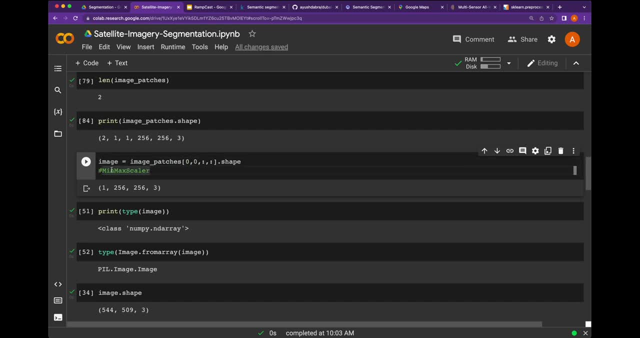 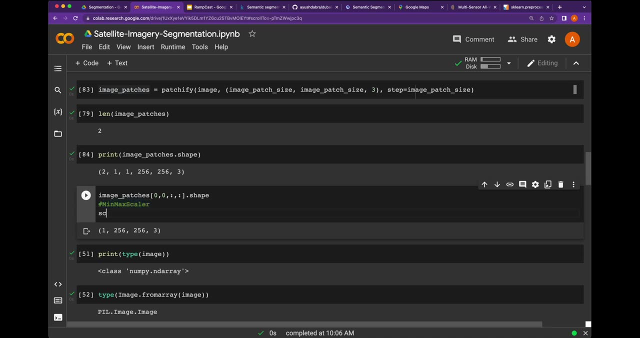 become our temp image. so let's take, this is our image, we just call it image x. now we need to process. so let's define the min max scalar first, so we could say: a scalar, or we just call it min max scalar is min max scalar, so we defined it. then we need to perform the 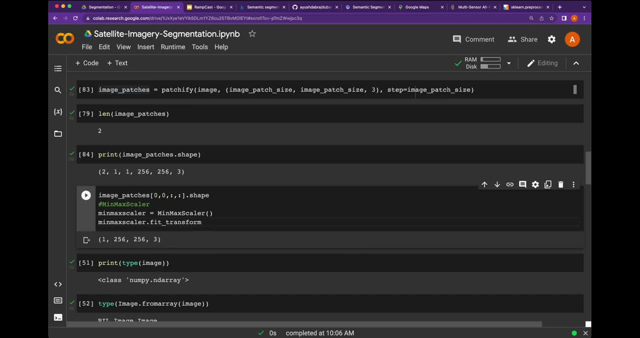 min max scalar dot, fit transform. and this fit transform is going to take the whatever the image we have as input. so we need to set up the image here so we could say: this is our image of x, image x, so this image x we need to pass here, then we need to reshape it, and this reshaping is going to be: 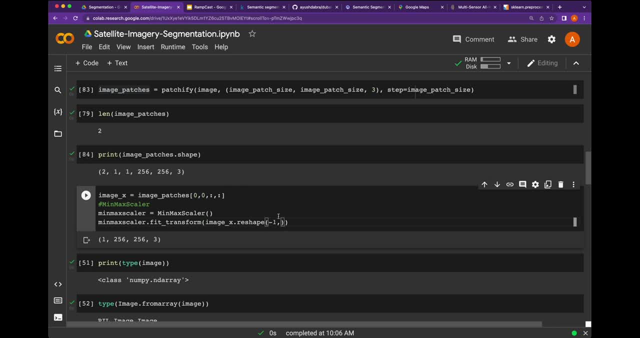 done through the negative one, because we are moving one left, then we are taking this image of whatever this available shape is of negative one dot. then we, once we have this, we could actually reshape it based on whatever the image we have, this of available shape, because that shape has to be. 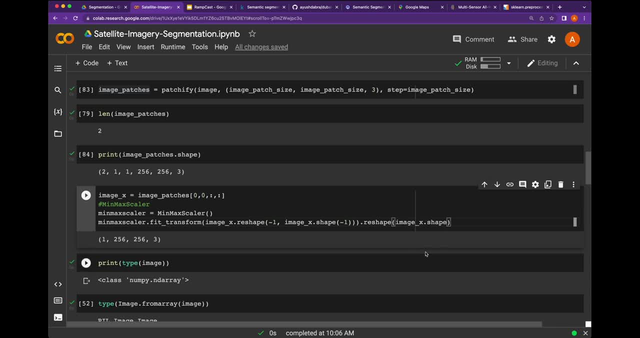 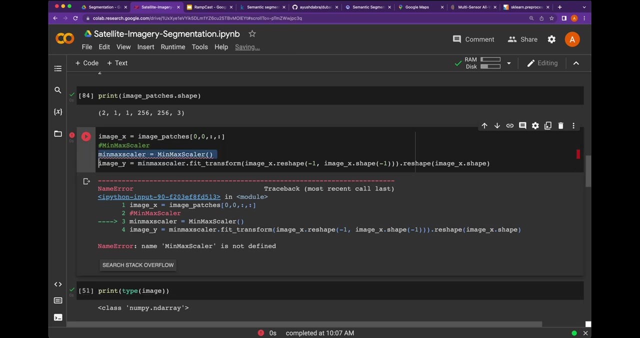 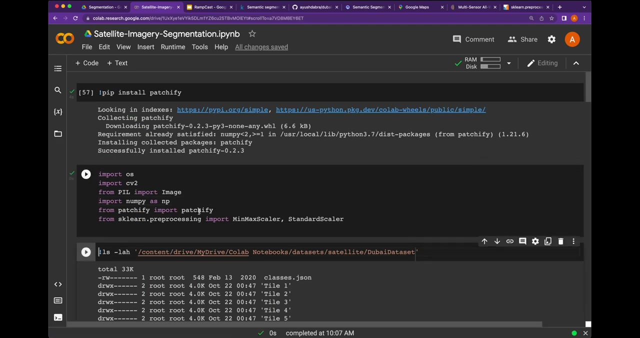 already been changed now shape. so if we run and then we call it image y, let's run it. let me take this and define it first here. so min max scalar. let me call this first, then make sure the min max scalar is defined. now it's okay. 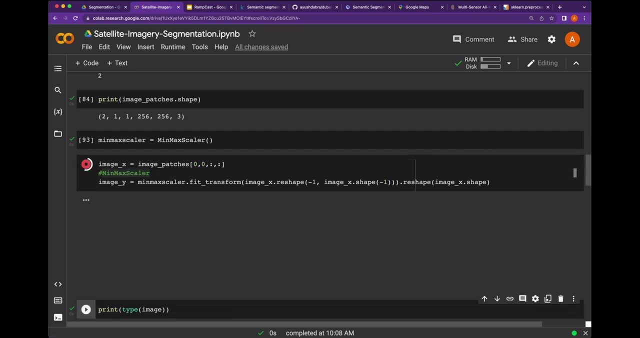 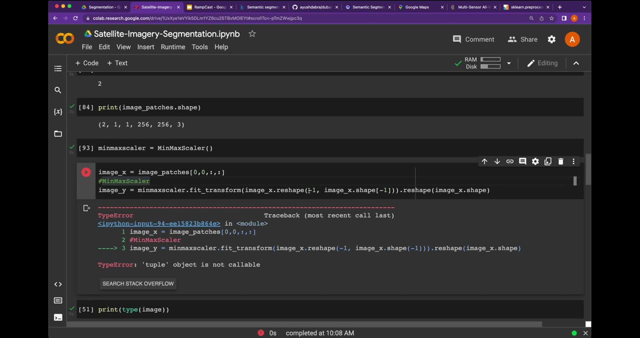 so min max scalar is defined. now we could make this call. it should be the array. now, that's my mistake here. that's why we got this error. rest, it should be okay. so reshape is going to take the two values and then shape two. well, okay, image y: now it's perfect. so now we can take this image y. 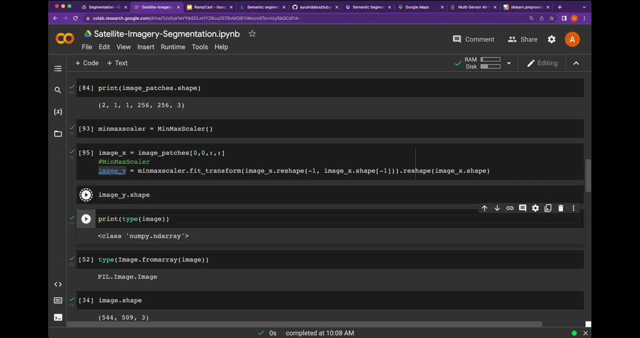 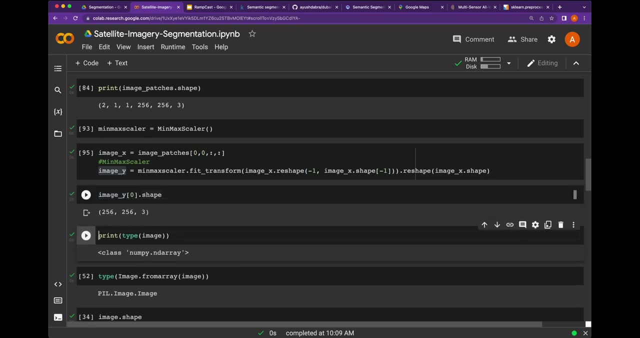 and we could actually see the what is the image y shape? now we take this image y and just only use the first part, and that's what we are going to get this image. so once you get this image y, we need to just take the first of this like the very first index value, and then 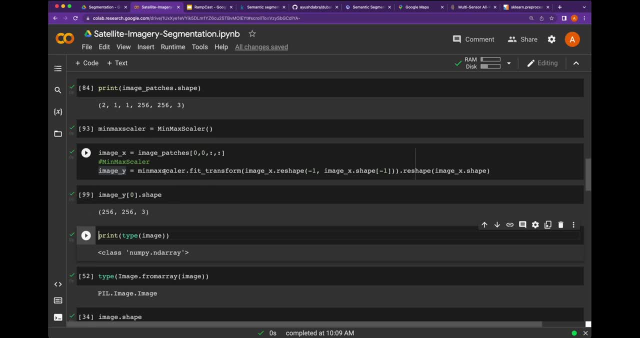 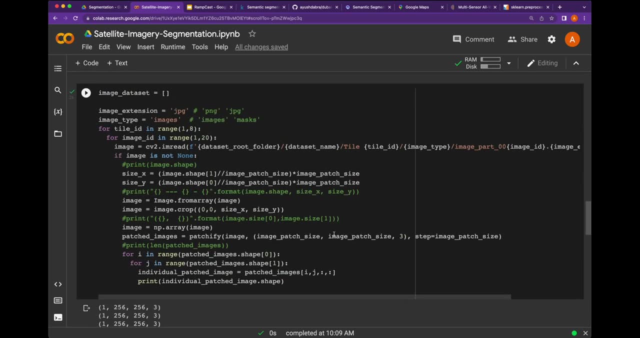 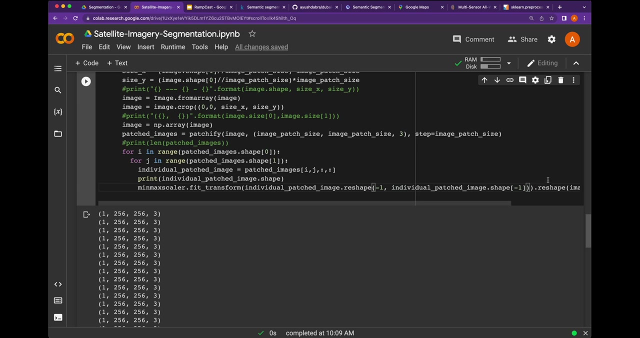 when we select this, that's what gives us the image. so we have performed the min max scalar on our code. so we take this whole code apply in our method here. so we take this whole code apply in our method here. replace this with this image, this image. 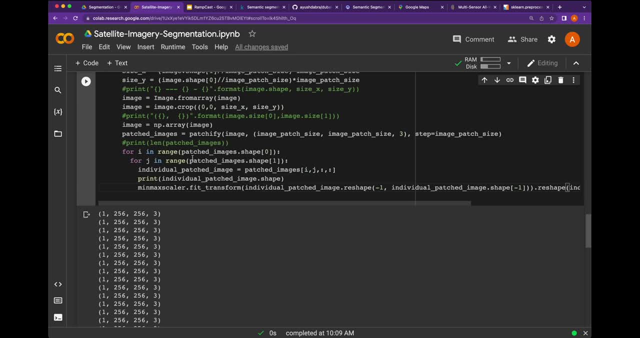 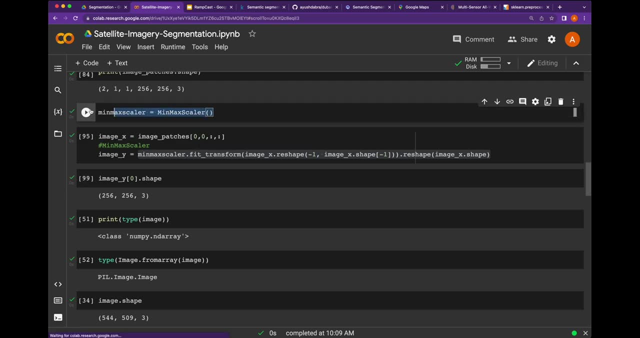 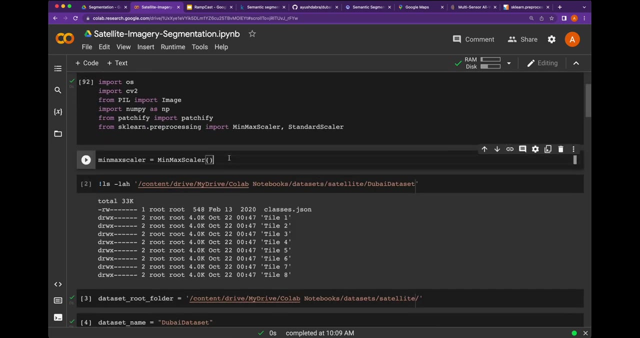 replace this with this image, this image, this image. so the individual visual patched image has been used here and we need to make sure that this method, we take this from here and we make sure that this method is at the very top, so you run this, you run this, so that's what makes it important there. so we will not use this method. 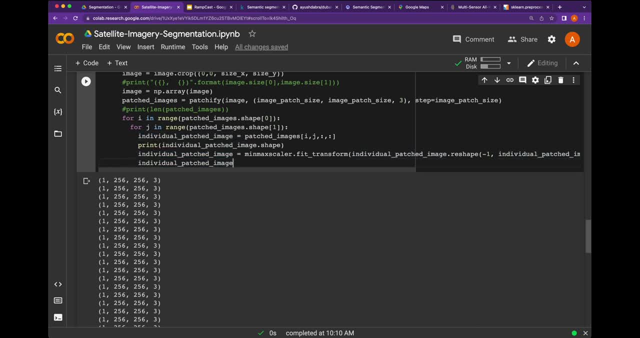 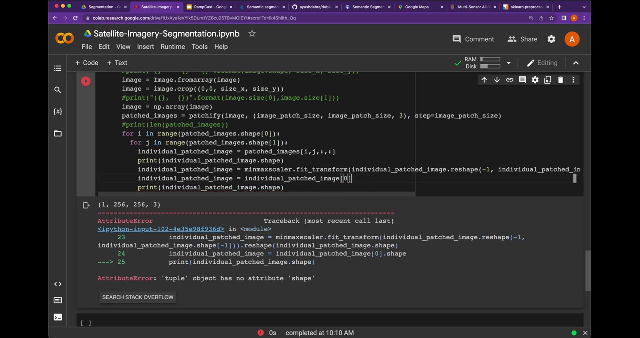 not forget, and that's where we get this image. and then we can say: this image is equal to zero of its shape and that's what gives us the perfect 256 by 256 size of image. we can say: print this image and its shape. oh sorry, this is removed. now it's perfect. so here we are, getting one of this then, after minimax. 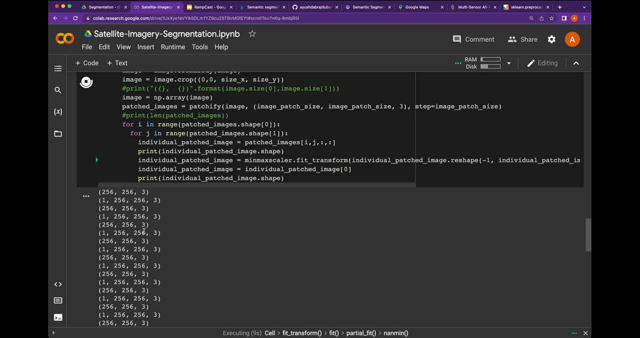 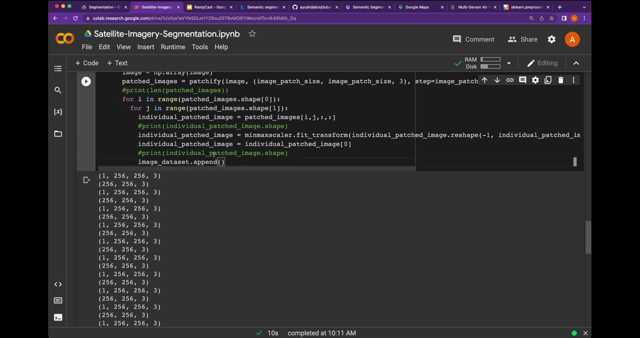 scalar, we are getting the image of 256 by 256 by 3, so let's comment this, let's comment this, and then this is the final value which we are going to store in our input image data set dot append. because this is an array and we are going to put this image here, let's run this code every image. 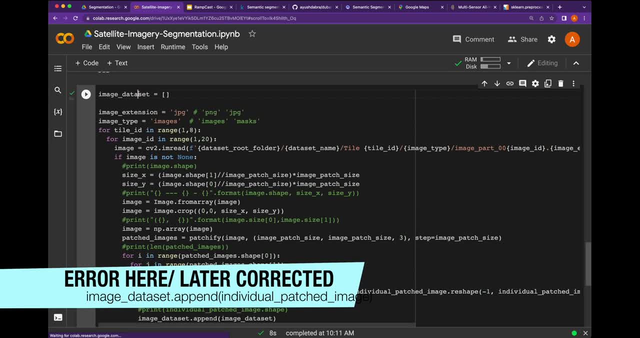 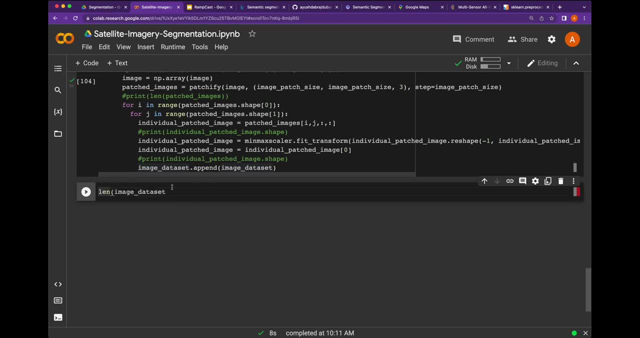 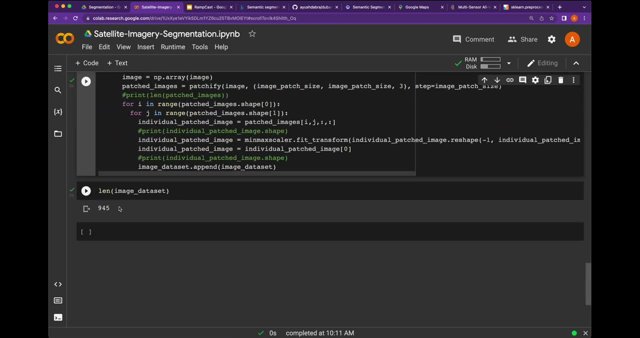 being processed and filled into this image data set. now we take this image data set, we say the length of the image data set. it's going to have all of these images stored into here. so here we started with zero. now we have 945 images stored in this image data set, exact what we have done for image. now we 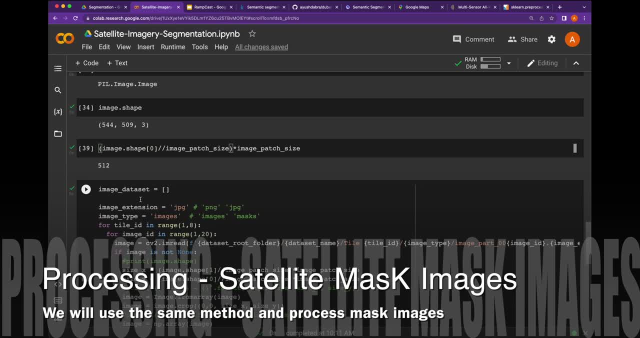 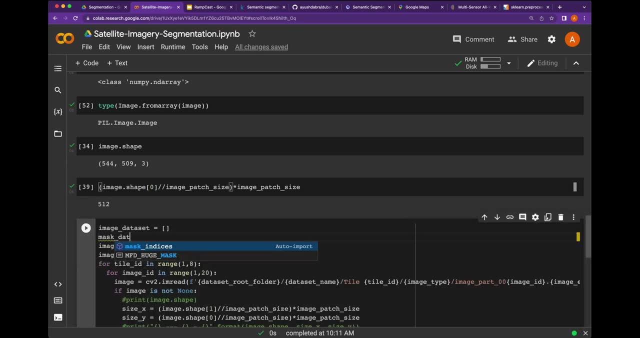 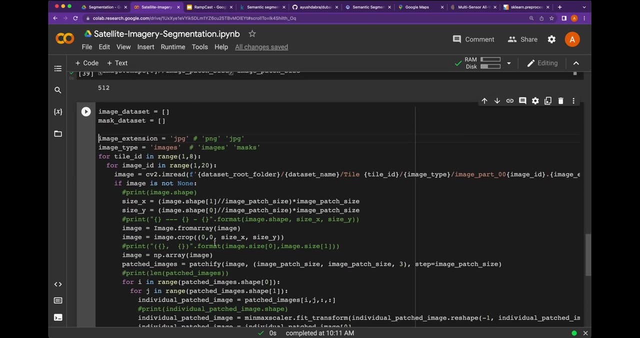 have to do exact same thing for our masks images. so now we are going to create a new data set- mask data set- and we are going to create a new data set. we are going to perform the same code, but we are going to make few changes here, so we are going to. 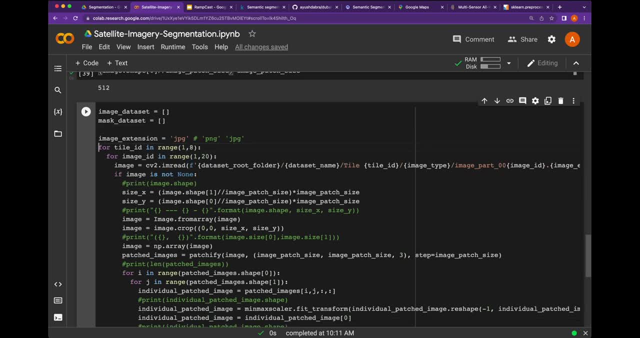 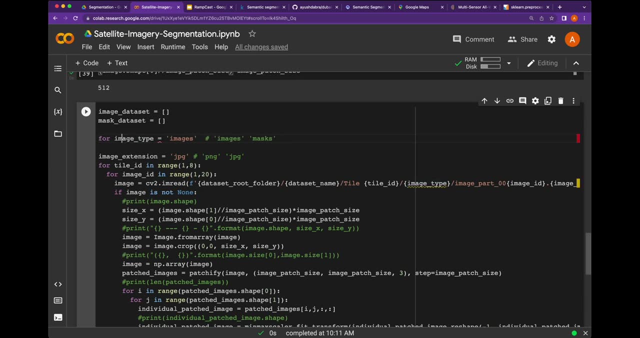 create the image types first. so this image type is going to be processed in a way that, for image image type in, we need to make sure that we have an array of images and masks, so that's why we will process both of them. we are going to write very lifted Apple com. 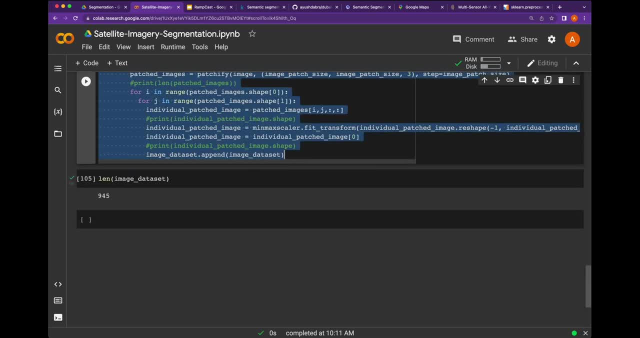 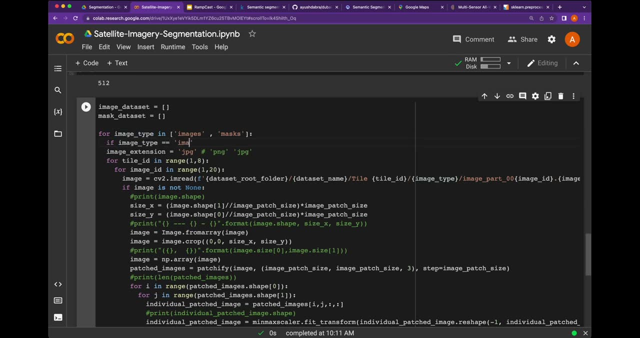 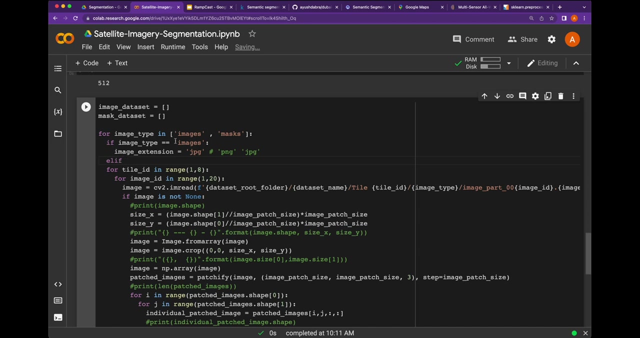 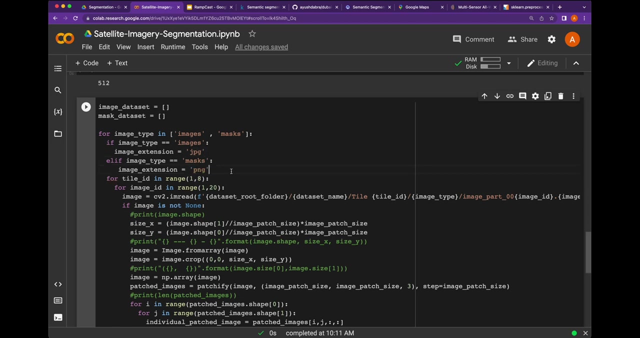 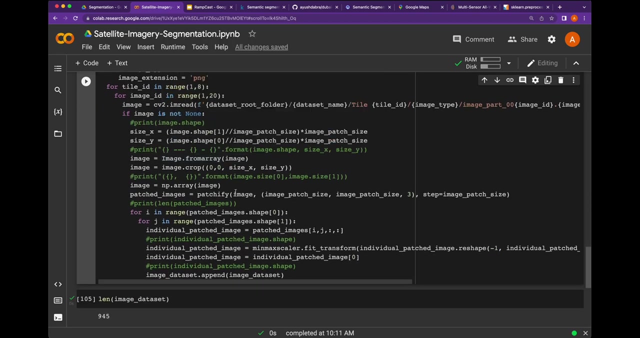 project sql. we are going to write a OMR OFF will. OK guys. data set, full data set. OK, now we could say if image type is images, then the image extension is going to be this properly and just just a very quick even. it's a wrong, but if you would want to, 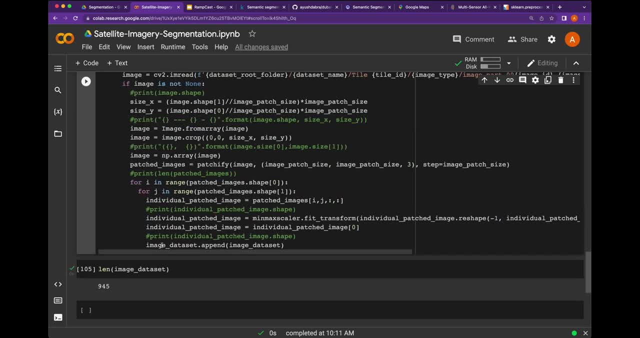 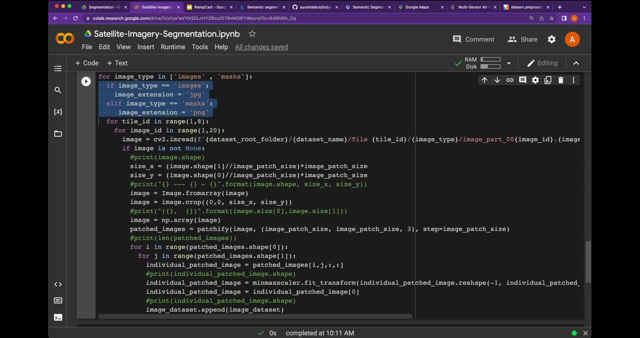 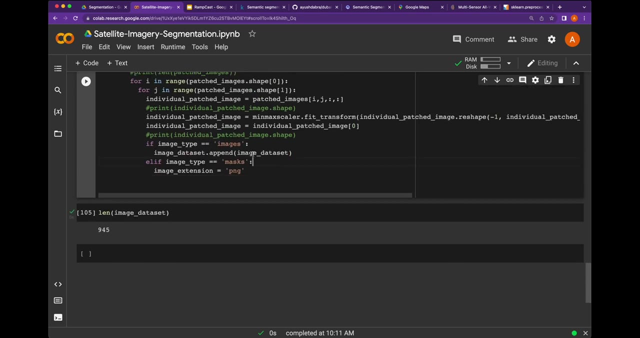 make sure that whatever we are processing has to be stored correctly. we just really need to make sure that we just make a simple check here too, at the very last ego, what we have done, that if this is the case- and this is the case- so this will be the mask data set. actually, this is not correct, but I'm just trying to. 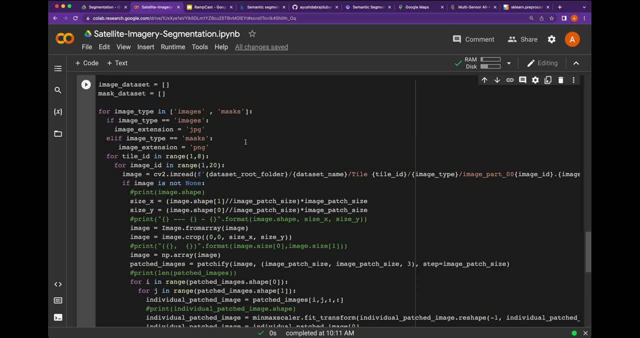 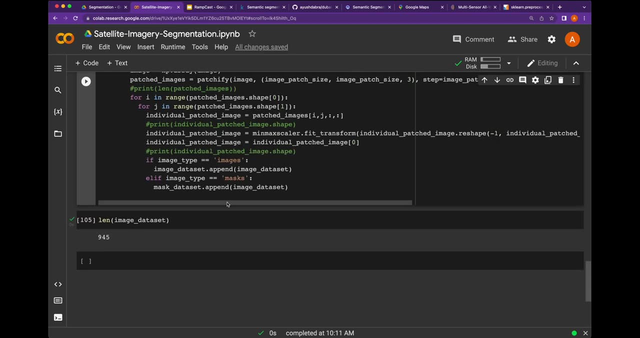 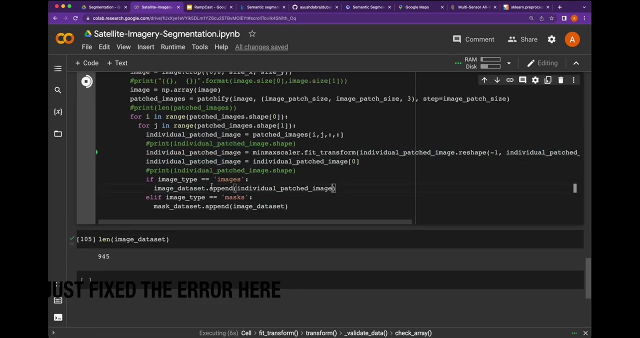 show you that how we are going to make few changes inside here, but at least this code is designed to read the images first, then mask first and then read the proper JPEG or the PNG and then store everything into individual data set. let's run this code or this is very bad code, so we need to put an append here. 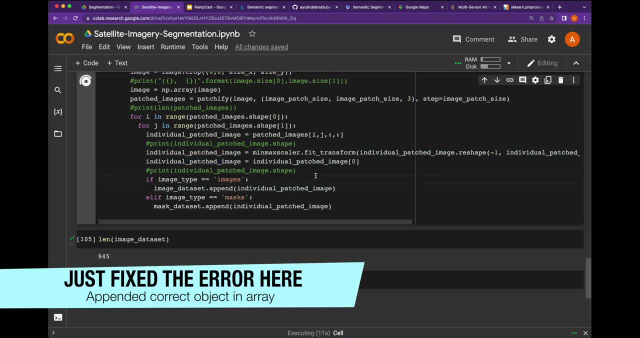 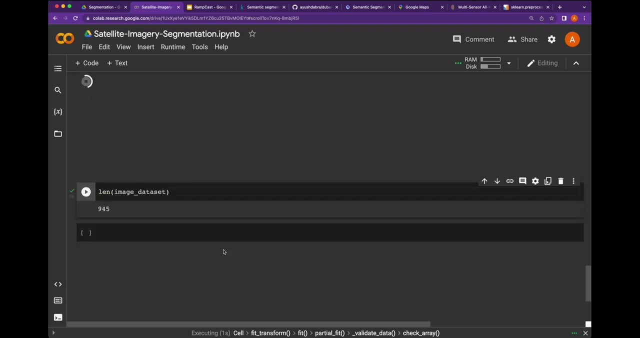 and we need to change this to append here whatever the patched image is. let's stop it, let's rerun this code again. and while this code is, we could actually use the same. we could say: the print of image data set and the print, the size of mask data set. that is done. if you look into the length, you could. 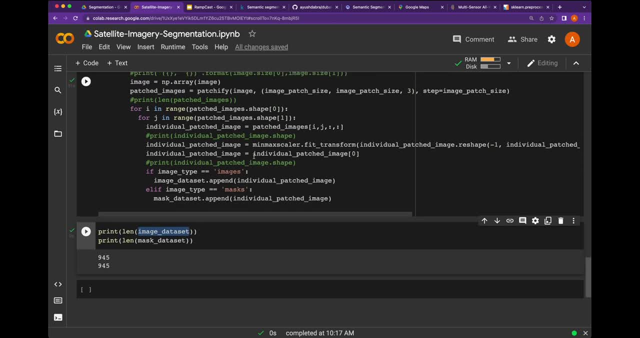 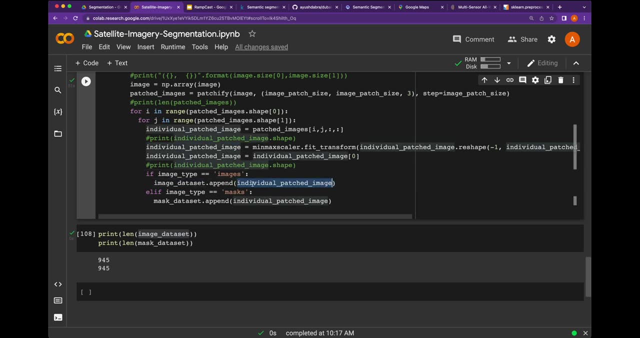 see that both data sets are having the 945 and 945 images. so make sure. one change: I have just added it because this individual image has to go inside the array. initially there was a bug, so at least we have got done. now we need to make sure that we make few changes. 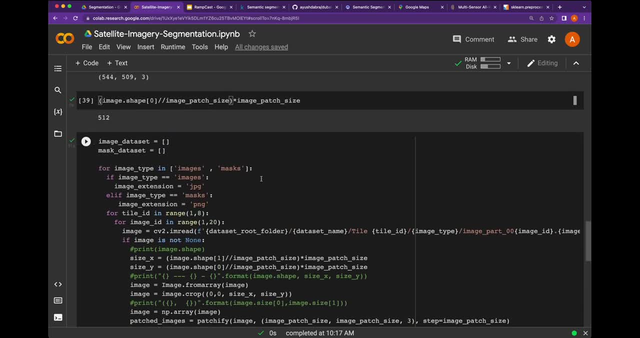 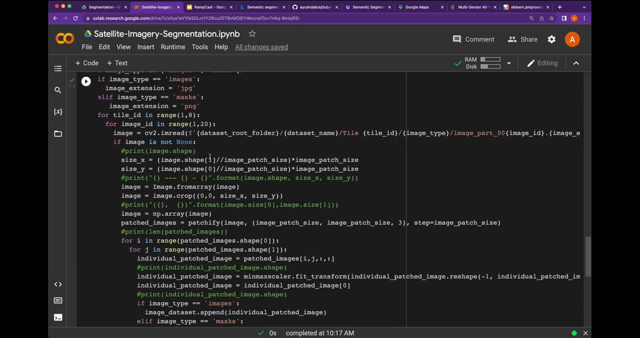 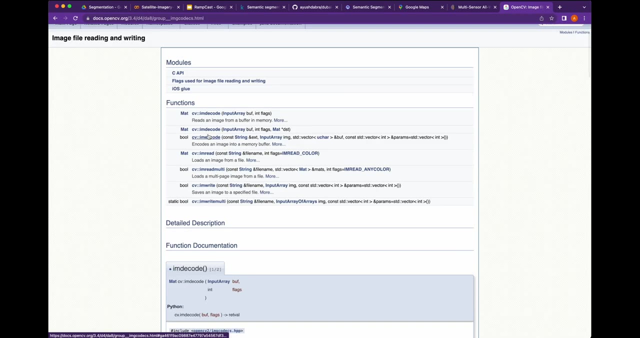 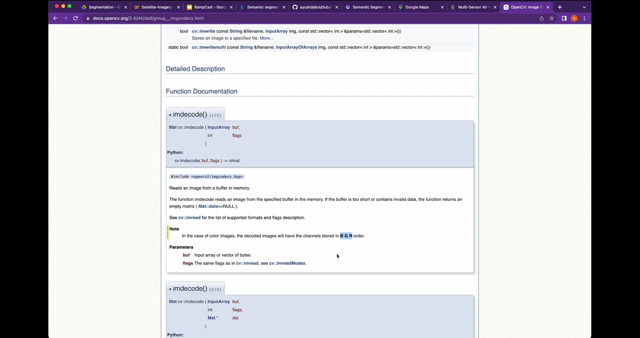 whenever we are going to process the mask, the very first change we need to do is that the way we are going to process these masks. so let's look into the CV to I am read method. so the open CV documentation say that whenever you are going to use the I am read method, the image is going to be decoded as a BGR. however, the image 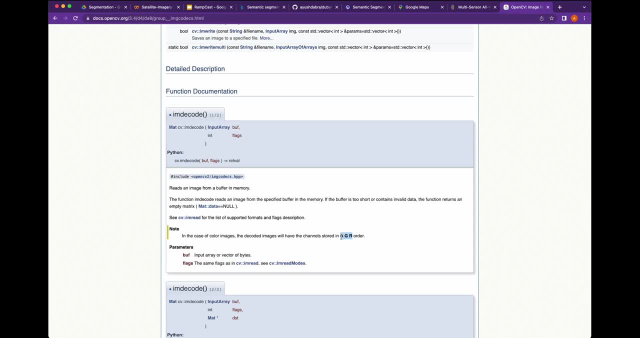 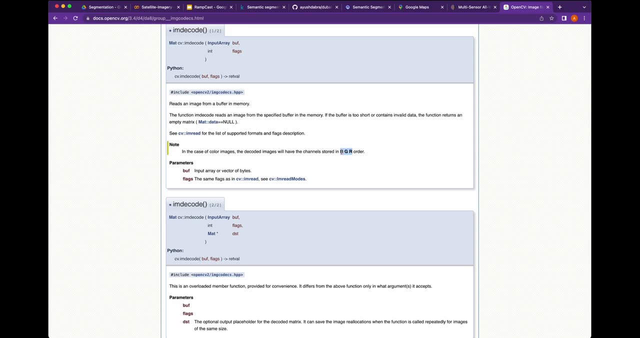 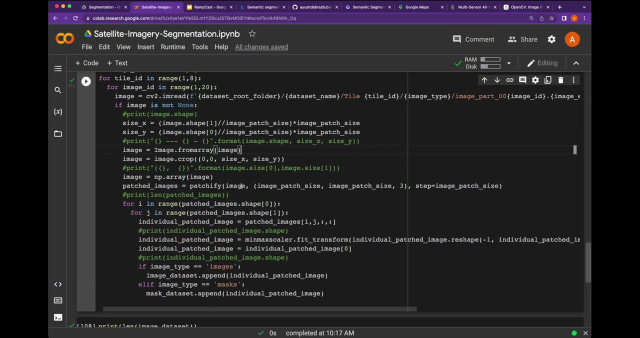 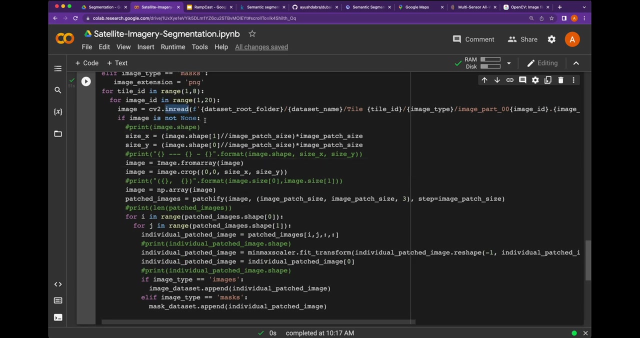 which you have is stored is in the order of RGB. so whenever you are going to process the images for your mask, we have to make sure that their order is set based on RGB, not the BGR. so whenever we are going to process these images, we need to make sure that after reading these images, the images have read correctly. it means we need to make sure that this image is being read correctly in the order and that iscase the implementation will not be good. and again, this checkedika, the current format, the new objections- has passed by the type that I want to: ميällіon تعالى, supَلعَدْعَدْعَدِبَس כלُ dovğisch. 65 behaves with export bg rufiı fol. 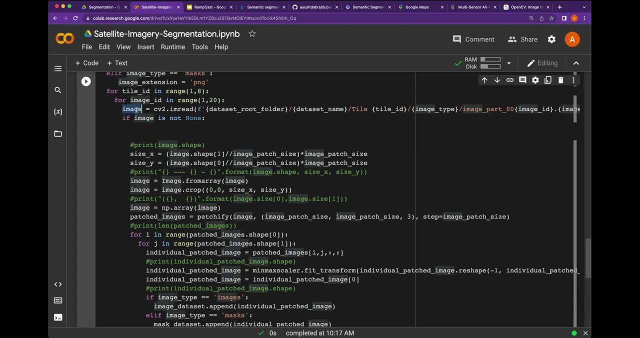 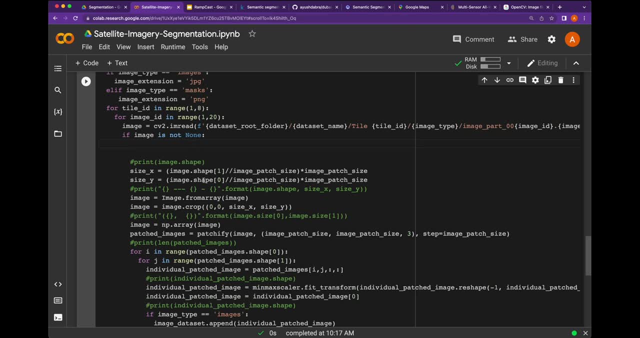 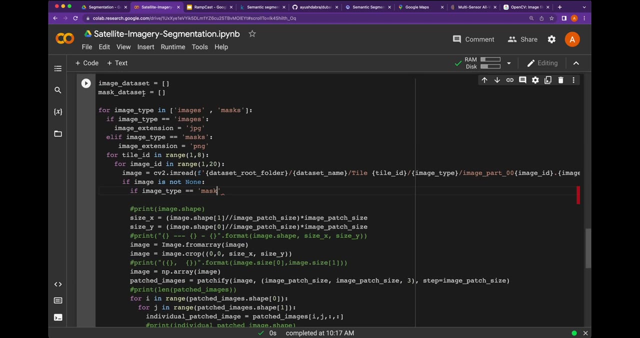 it means we need to make sure that this image is actually being set properly into the RGB order, not the BGR order, so we could say: if image type is equal to mask, because that's what image type is equal to mask. we need to make sure that. 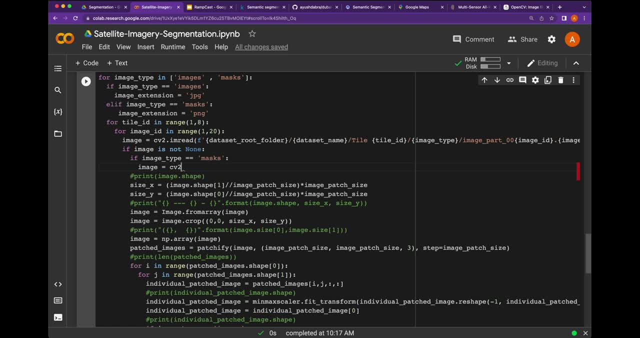 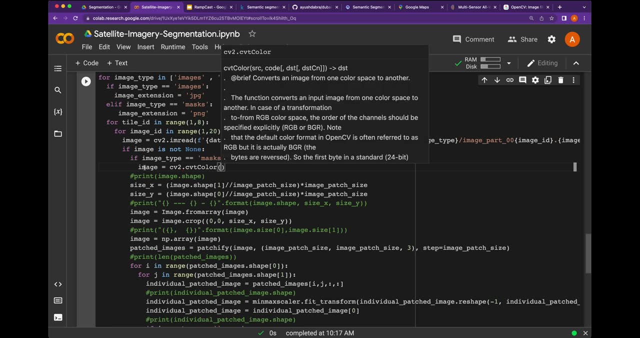 this image is equal to CV 2 and then we have to change the color. so CVT color is a method where you could say that you would want to take this input image and you need to change its color to CV 2, CVT, CV 2 types. so what is our original color? 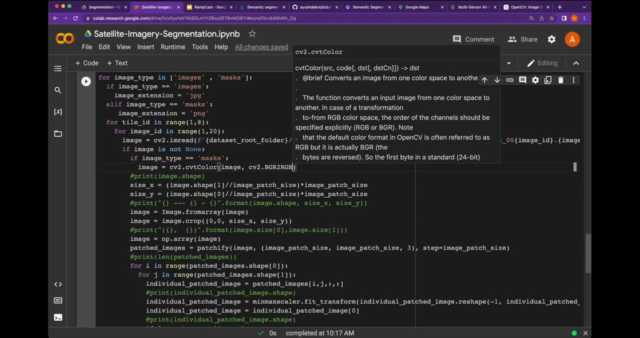 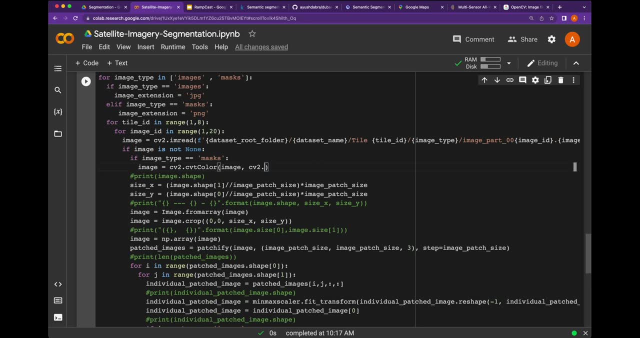 is BGR to RGB. so that is the color type we would want to change and this is actually the color. if you see, here we can actually say color, it will give BGR to RGB. so this way, our image has been changed from BGR to RGB because we have 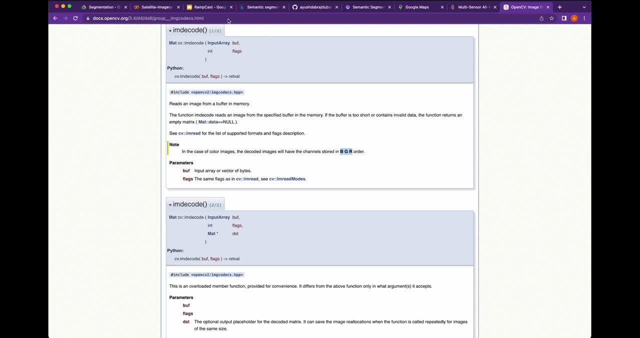 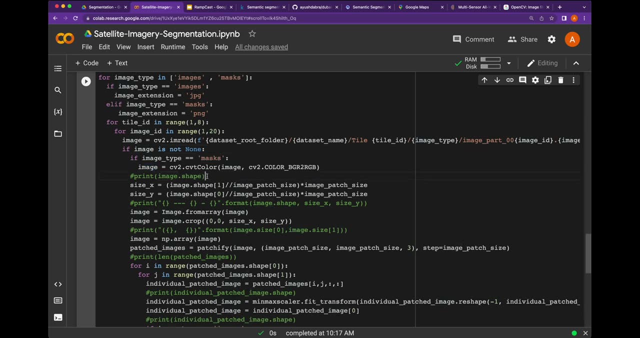 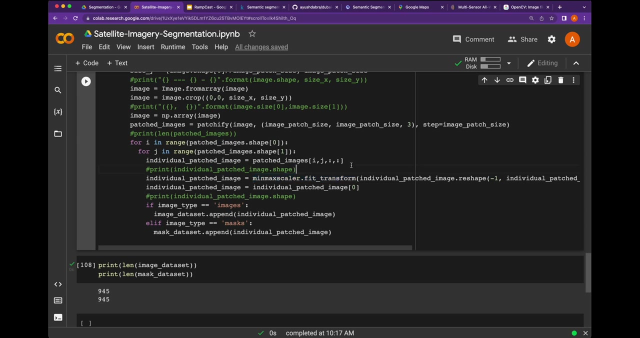 validated, that input is read for the BGR and then we are doing that only for masks image. that's a one big change we need to perform. second, we need to change this because we do not need to do the transfer, because the mask image are not, because we are only performing the transform for the input. 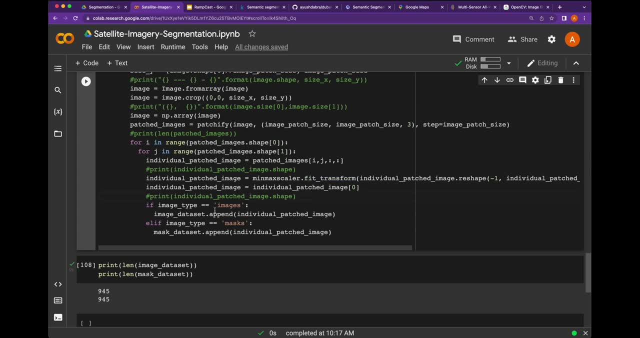 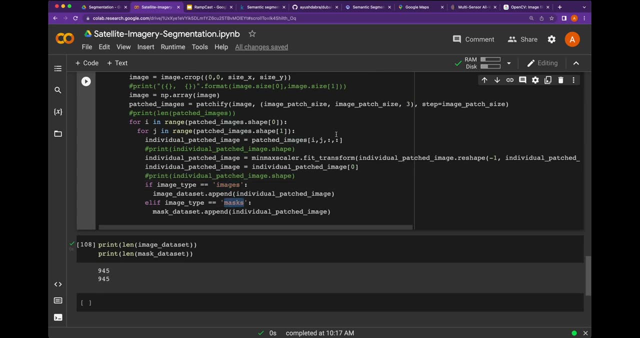 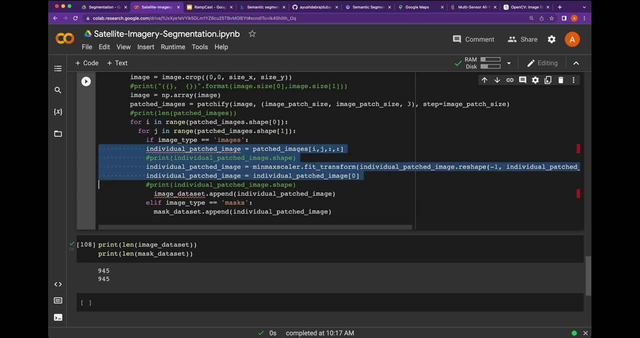 images, not for masks. so we need to change this code which we are trying to process for individual images or the mask. so I will take this whole code from here for now and I will put that is inside this images area. so it means we need to write a new code. 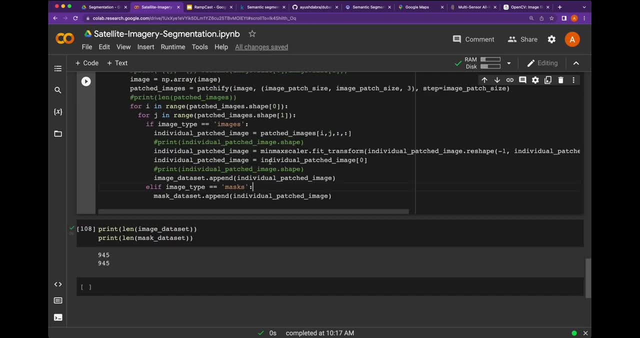 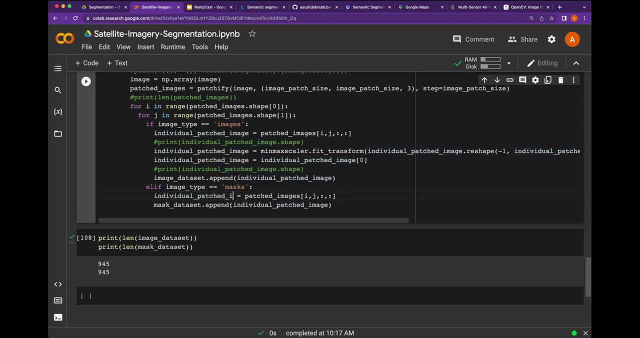 in order to process the mask images. so first thing we need to generate the mask so we could say: individual patched mask is going to take the same patched image, which we have done, and then get the patched mask. at this point the patch mask is basically the size of 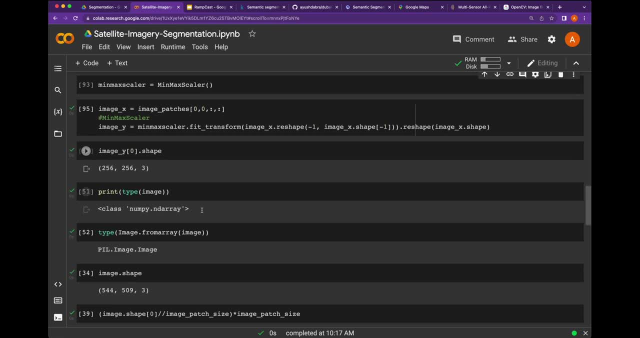 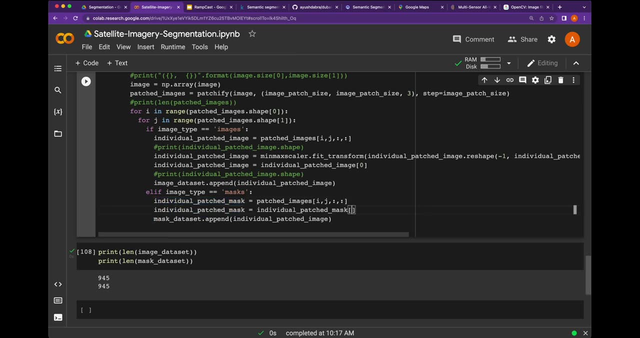 one of this, so we need to get only the image out, so you could say that individual patch mask is equal to the first one. and now we need to mask. data set must have stored this mask image. that's all we really need to do. we really do not need to perform this part, so that's why we have individual 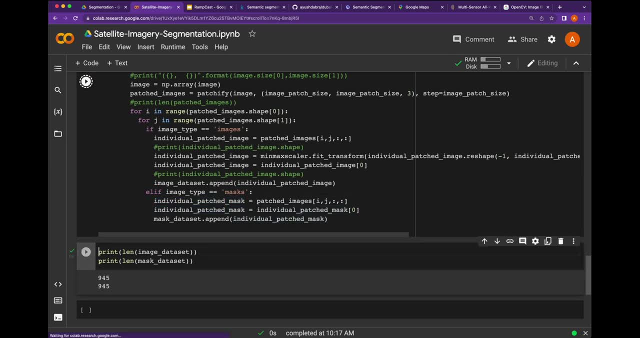 patch mask images, so now we can run this whole code that is going to generate the same size of image as well as the mask data set. however, the images inside individual of these data sets are masked image in the rgb format and in the individual image, which are the original as it is. now we can check the size. 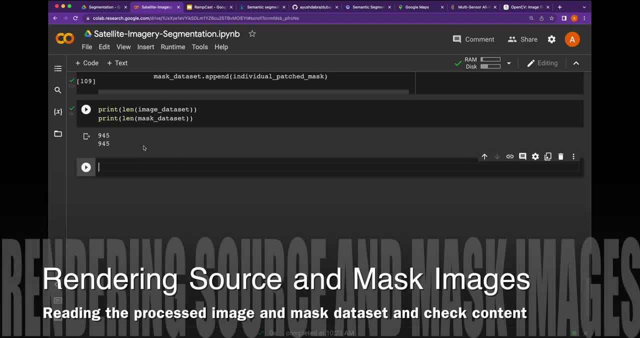 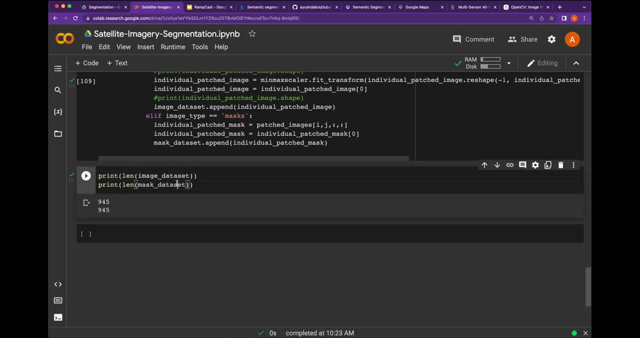 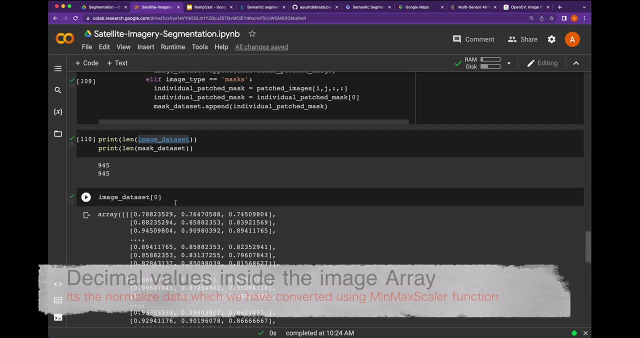 they both are 945 945, but now we need to validate that. can we make sure the images which we have stored in both of these data sets are the correct one? let's take a single image in image data set, which is, so here is what the individual image inside the image data set look like, if you will. 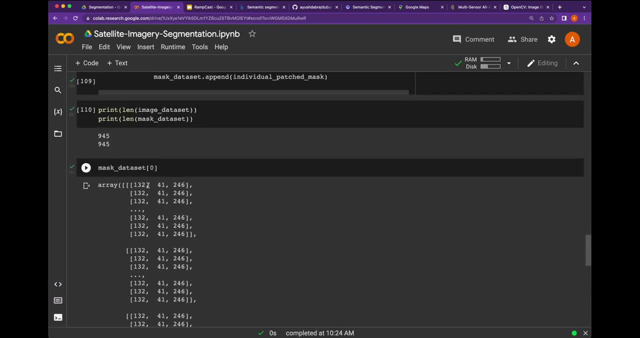 want to check for mask data set. that is what you are seeing into the mask data set. so now, if you would want to take this image and convert that to numpy array, if we just take and say np dot array and convert the mask image, so this became the numpy array. same thing. if you will try to do this for the 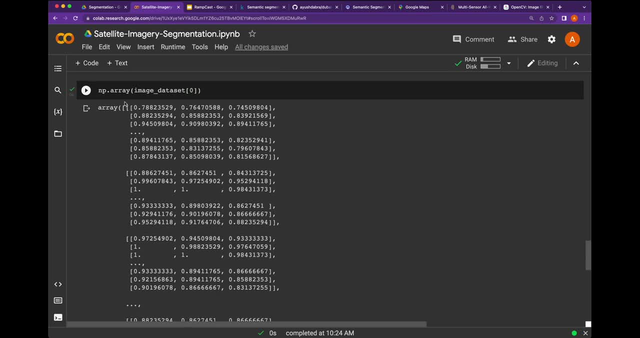 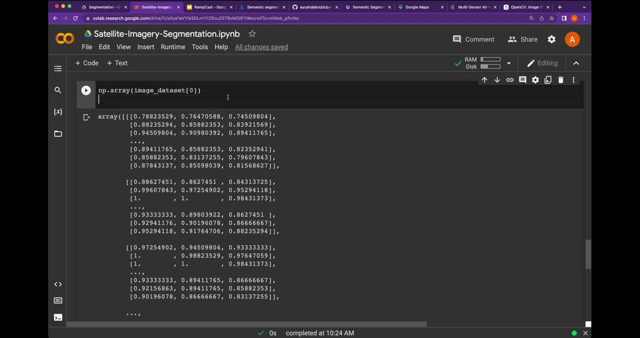 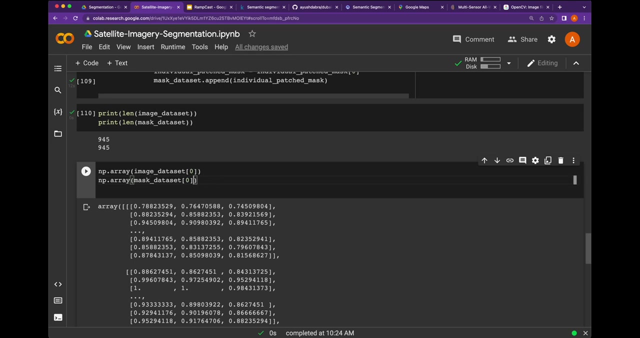 image data set. now it's became the numpy array, so we want to make sure that the data is uniform in the two of them. so we are going to perform a very quick check for all of the images in the mask data set and for all of the images to the image data set, and 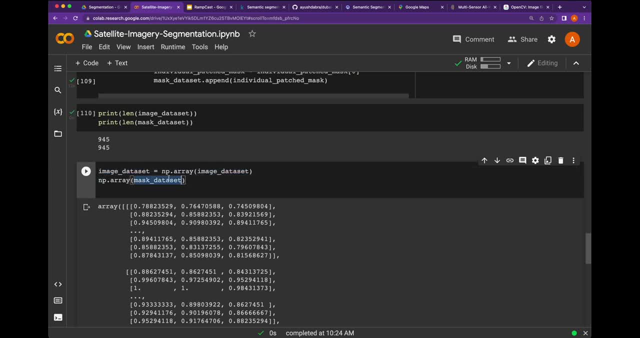 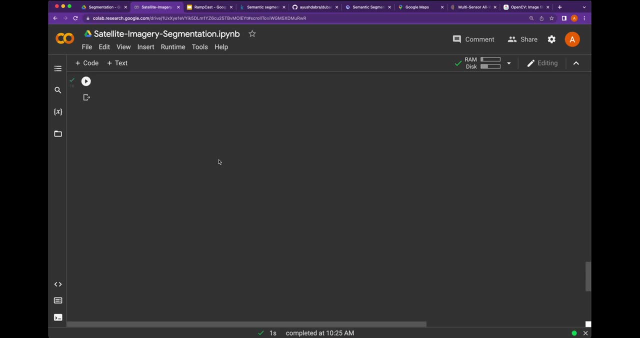 we make sure everything is uniform here, and for the mask data set and np div array. so this is just a confirmation that everything is in the numpy array image here. it does not change anything for all images. so that's what we will look for here and this is so. this is the ranking of the old image for all images taken from our Mod. 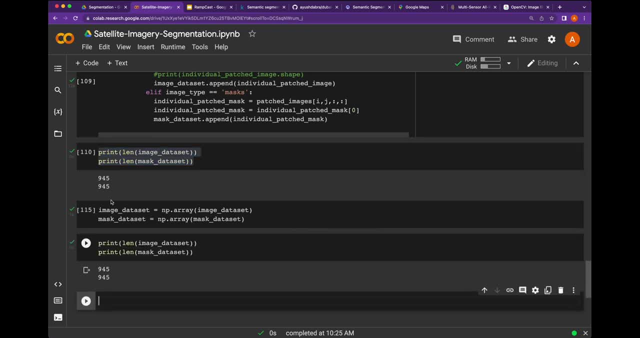 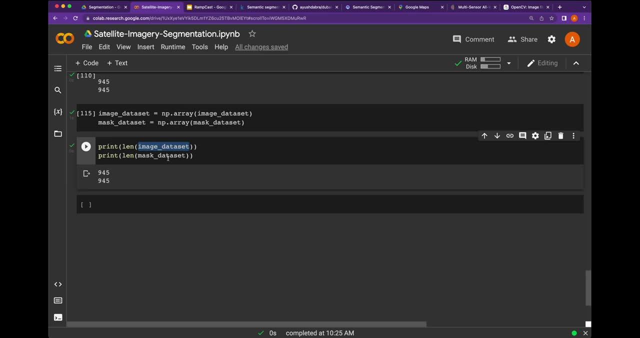 anything in terms of the size of your images. so if you see, here that is still, everything is same size. here now we need to show the images which are stored inside this data set, so let's try to work on that. so, in order to show these images, we need to use the library called the matplotlib, so let's. 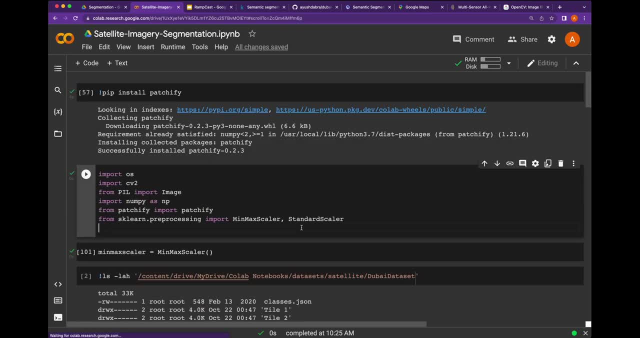 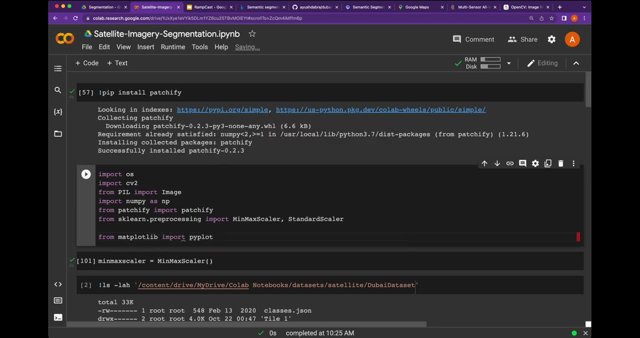 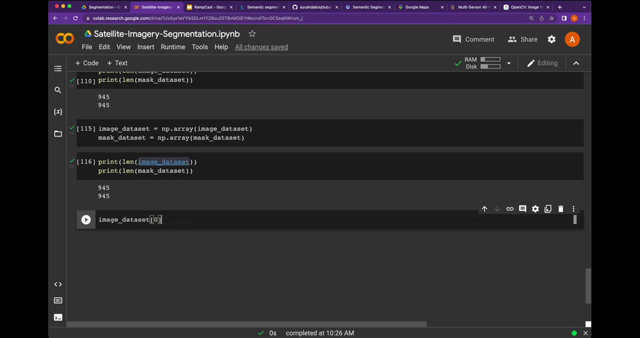 import that library. first we can come here from matplotlib import. I plot as plt. so now we have the plt object which is referencing the pi plot, but we can use the plt. so let's take the one of the image here. so this is the image number zero, which is is a numpy array. so if you 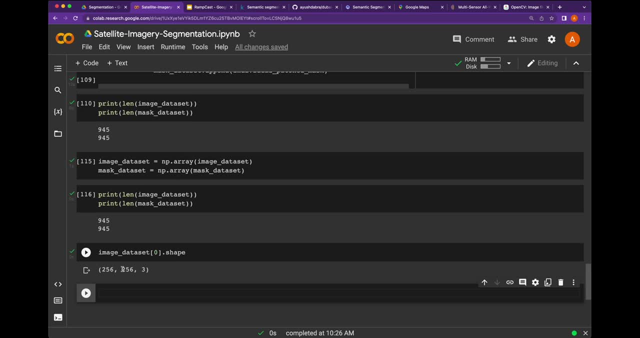 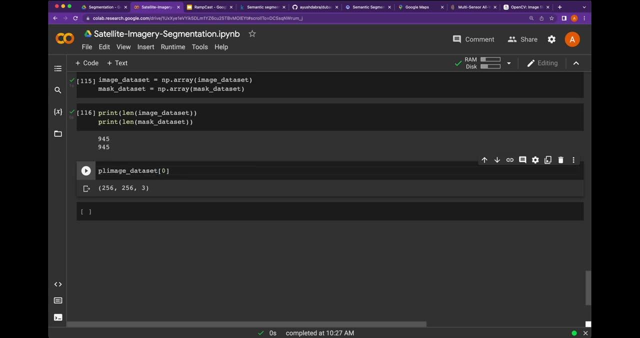 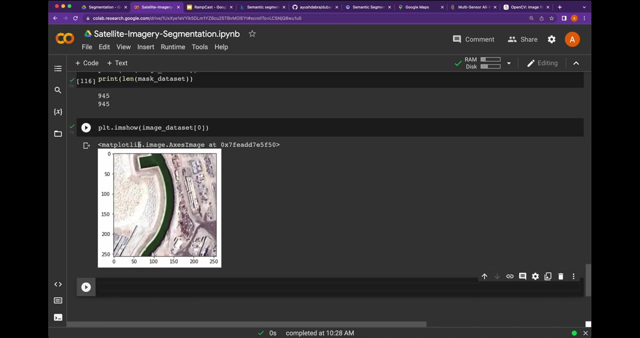 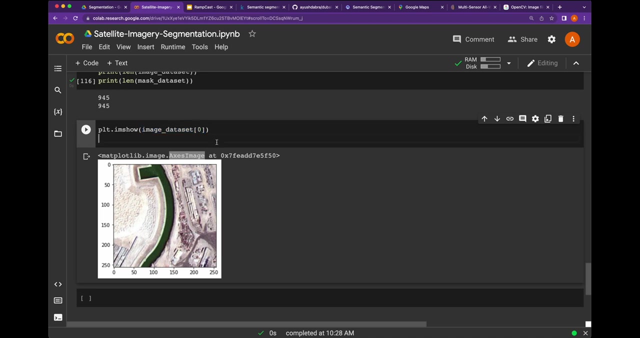 look into this image of shape is 256 by 256 of one. so now we can actually show this image using I am show method of plt of pi plot. so plt dot I am show. this is our input image, which is actually the matplotlib is taking this image and showing it. however, if you will take this image, you will say: let me show you. 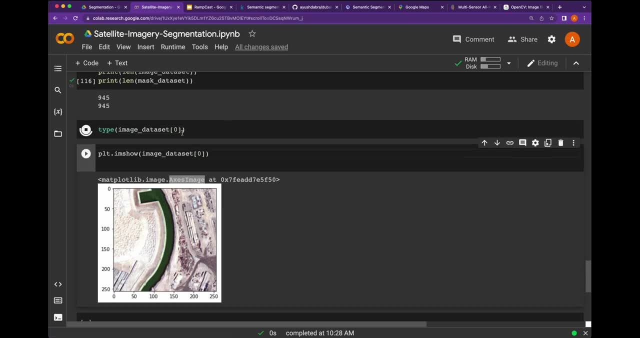 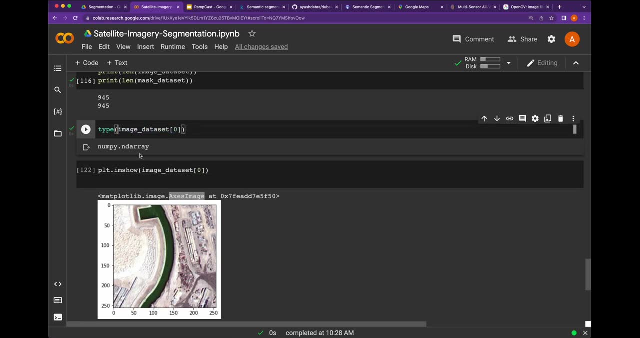 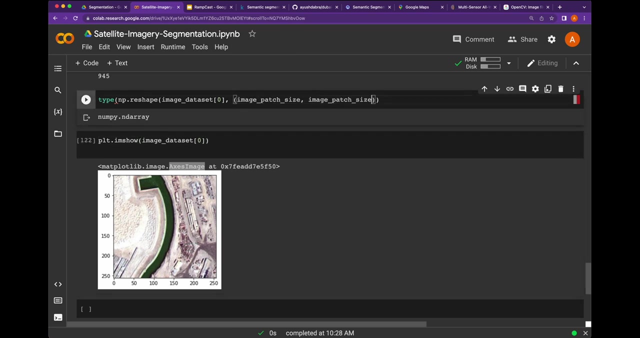 the type of this image is actually numpy array and if you will take this image, for example, and you say I would want to do numpy dot reshape, you take this given image and you would want to convert that to whatever your patch size is, you could say I would want to change to this this of three. so this is numpy nd array. so whether 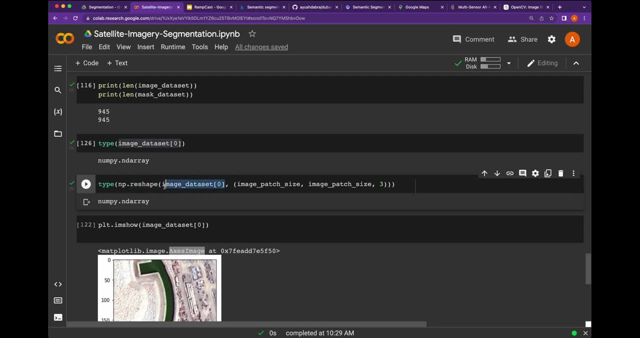 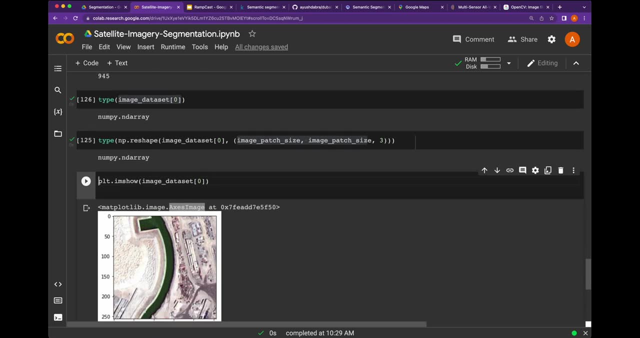 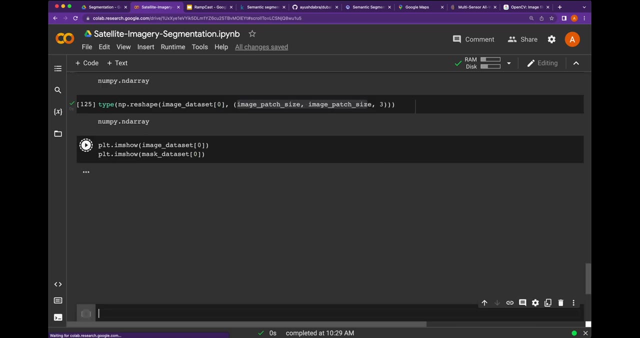 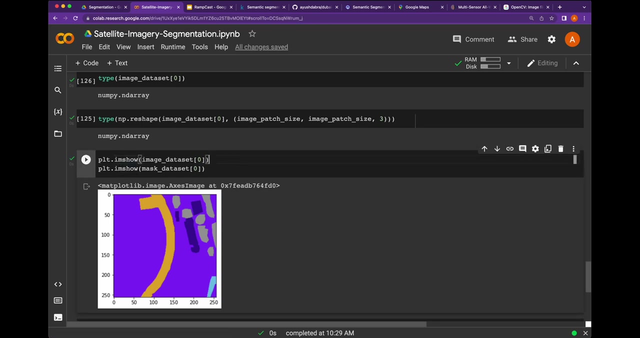 you use this image or you reshape it based on input image and back to this way they both are exactly the same. so now we can also show here the plt dot I am show and we can also say that what is the corresponding mask image. so here we need to show these two images side by side. so we need to do little more coding to create. 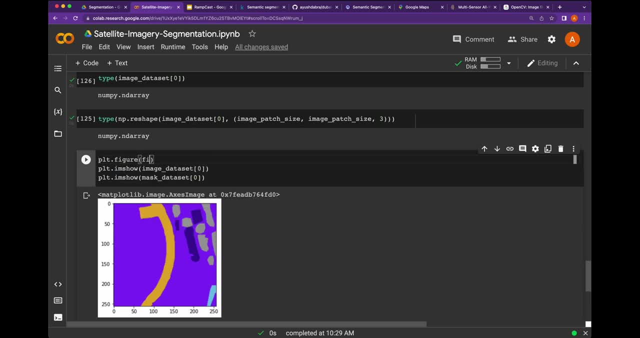 the subplot plt dot figure and you can define the figures fixed size. and you could say: my fixed size is 14 by 10, so make it 8 and you can create the subplot. you call this first subplot and this subplot is going to have the first image. then you can create the another sub, plot, two, and after that 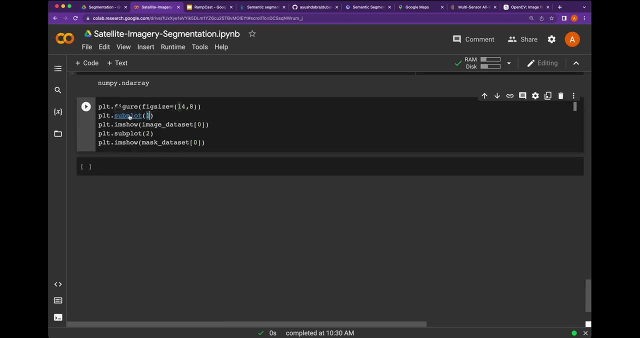 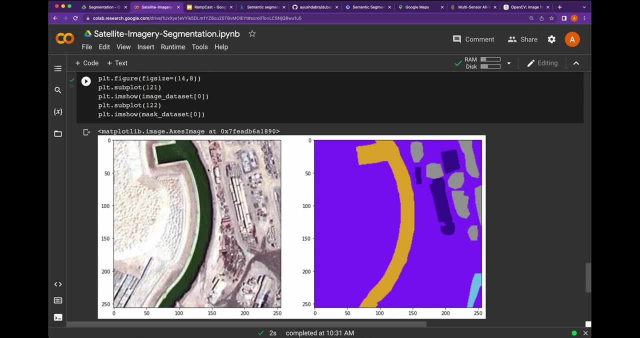 we need to. the subplot must be the three digit number, because that's where the subplotting is been defined. so we need to make sure that this number is 121. this number is 122.. let's run this code and as you could see that we have the left side is the original. the right side, we have the. 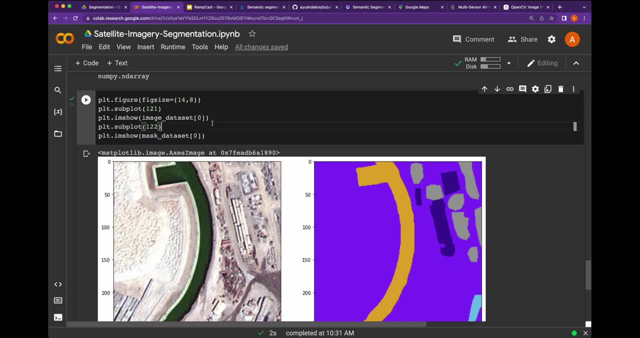 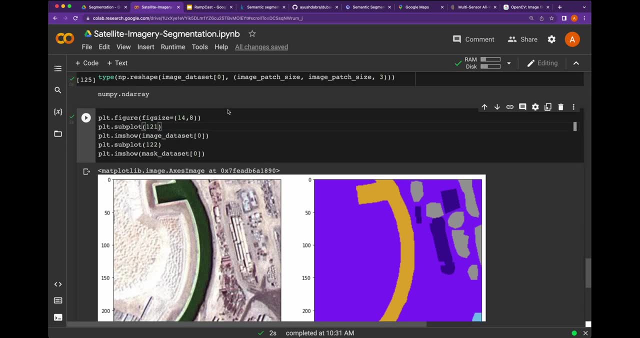 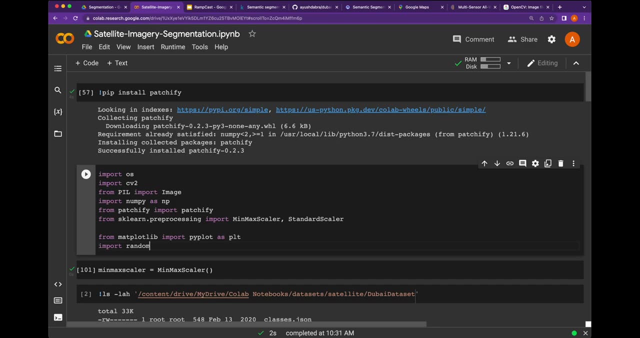 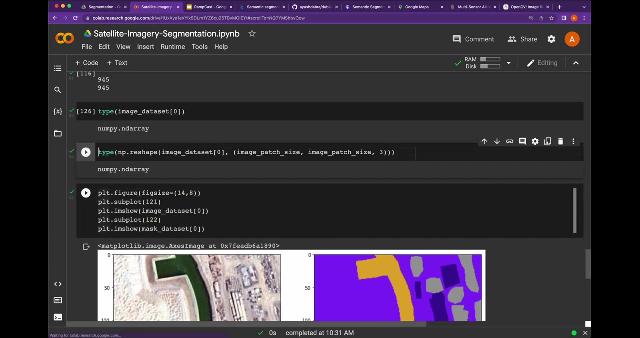 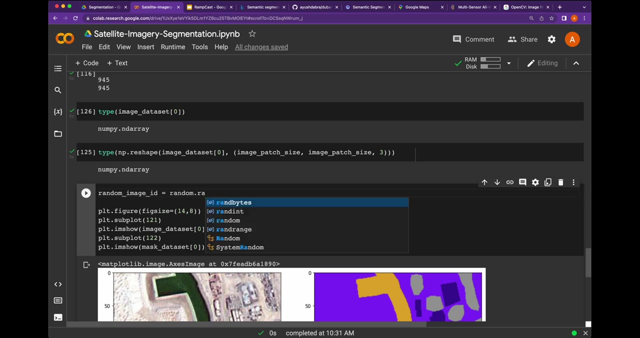 mask image. now we need to make sure that these numbers should be the random, so we could get an idea of any image stored in our image as well as the mask data set. so let's import the random. import random and then we can actually get the image ID. so you can get here. you can say: random image ID is equal to random, dot, friend, int and here: 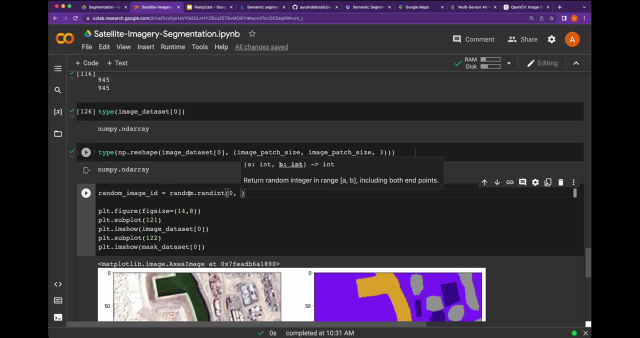 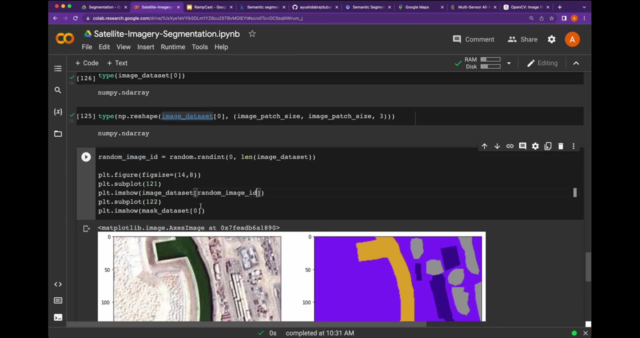 we are just creating a range so you could say the total length between 0 to. whatever the length of our data set is, we can use image data set, length of image data set and that will generate a random image ID that we can inject here or inject here. 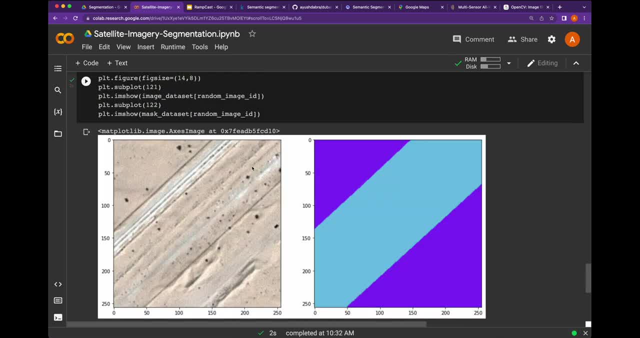 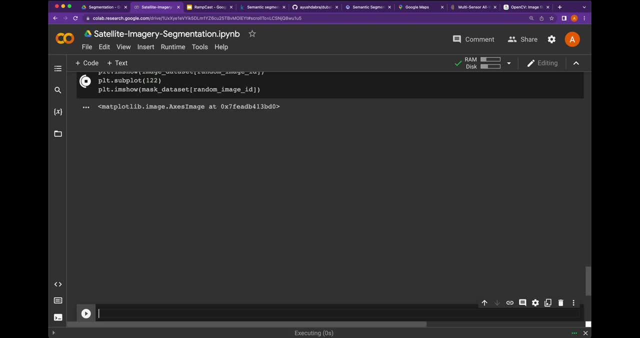 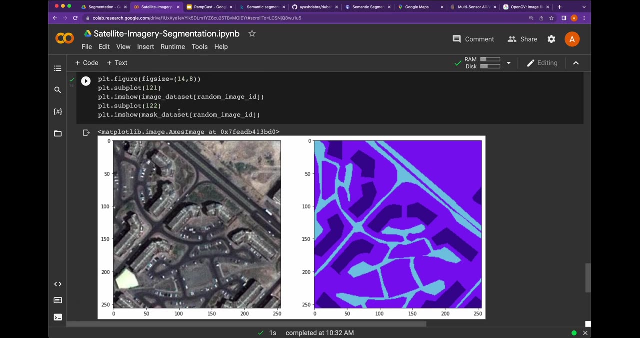 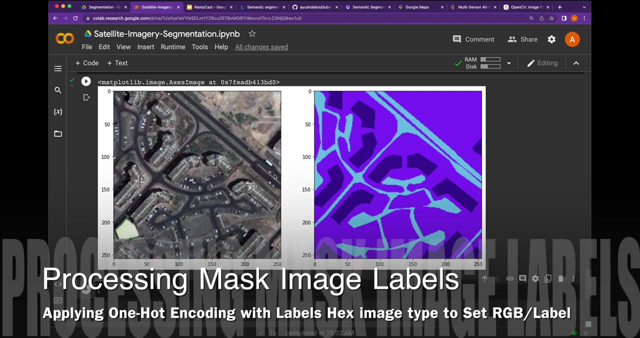 and that's where a random image will be selected. as you could see, you can get a very good idea how these images has been stored in our image, as well as the mask data set. in the next step, we need to process the labels and add the one hot encoding. so this is what we 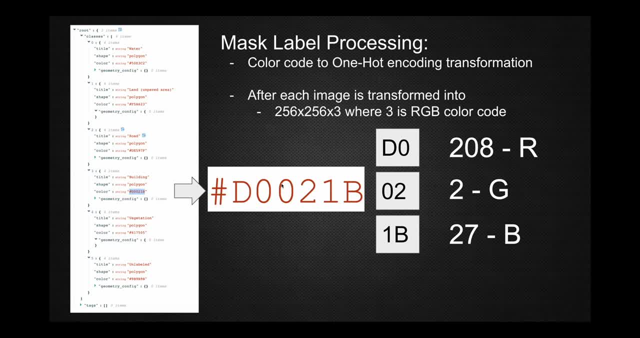 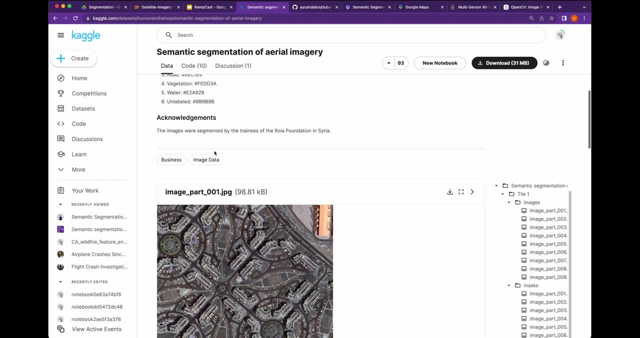 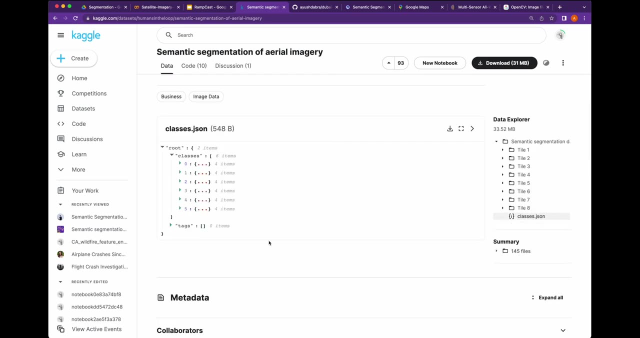 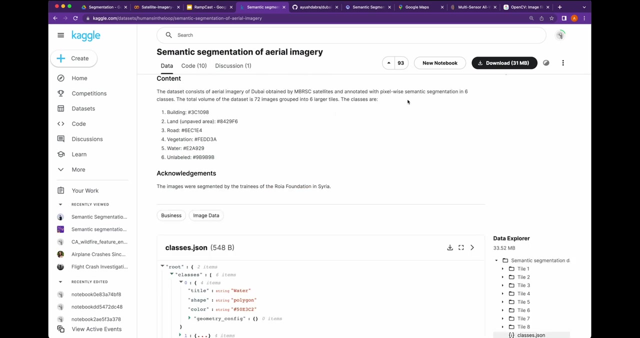 have seen that given image, we need to make sure that we are able to generate the one hot encoding for our labels. so, looking into the JSON file which is available with this data set, as you could see that here are the water and water value is 50E3C2. however, the segmentation when it was done, the water value has been changed. 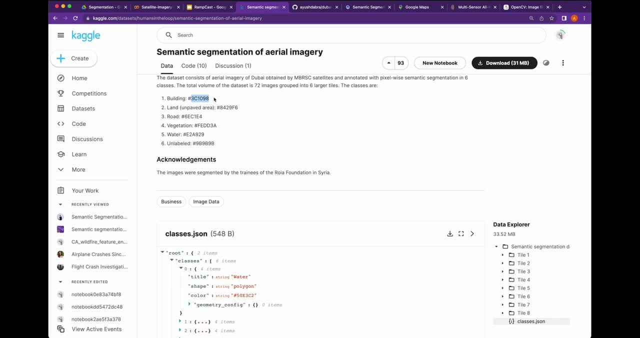 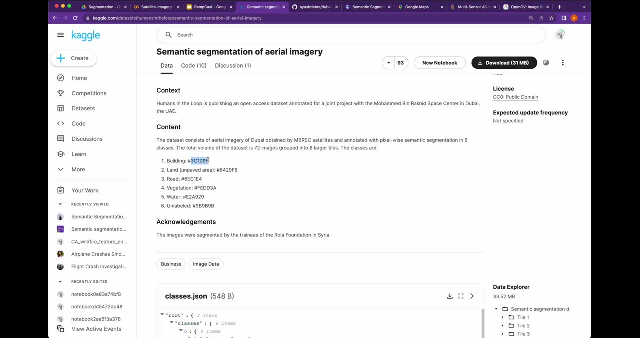 from this value to this value. if you look into the building value, here is a d00 to 1B. however, the actual building value is 3C1098. so we are going to use this annotation to process our one hot encoding. let's come back here. so we are going to write the. 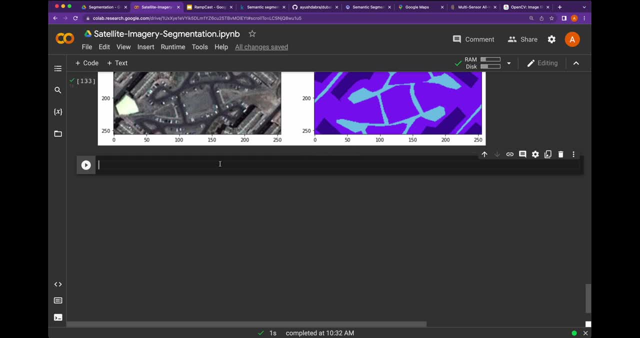 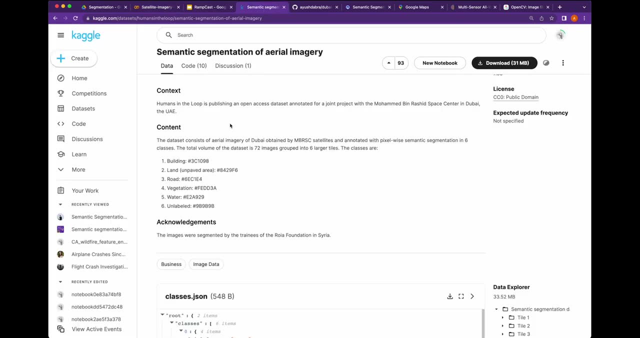 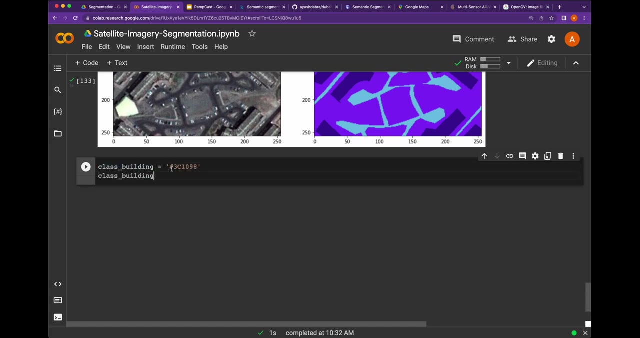 python code to convert from hex value to RGB. so let's decide: the building class is building and the building code is this. so first we need to make sure that we do not use hash here, so we could say l strip and remove the pound, and remember we need to split this value into the three segment: this, this, this. so we need 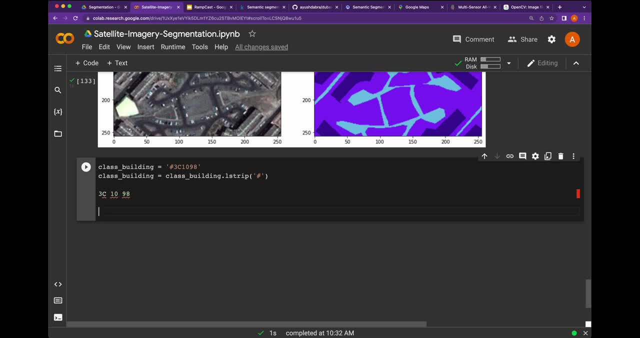 to write a particular code here. so we need to generate everything into a tuple for I in. then you can give range, so you can say zero, two and four. that's is where your range is, and then you are going to create the tuples based on that, so you could. 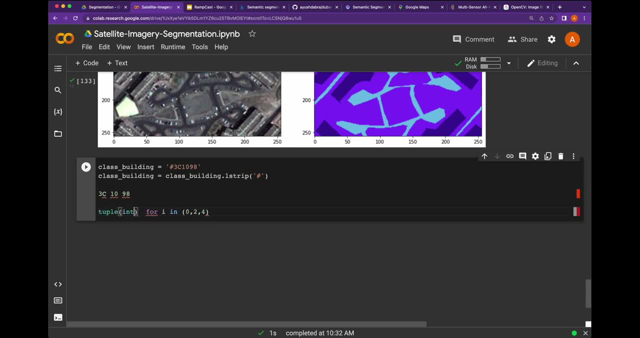 say the int, the tuple of integer value of given this class building, and when you are using this value, you could say you can take this: I colon, I plus two, and what we need to take this integer of this value. so we take these value and because this is a hex, so we need to make sure. 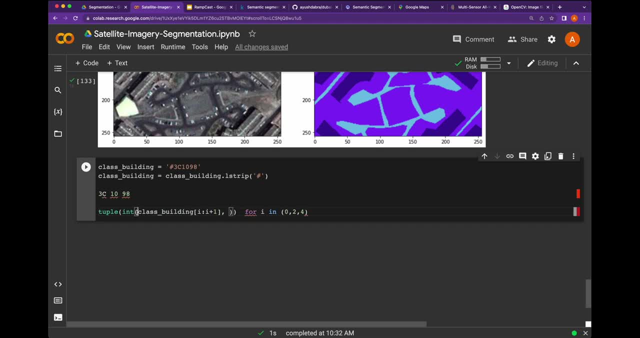 that this value is actually being processed by the value of 16, which is the base for hex decimal. so the integer it should be here, comma 16.. so I think that should be the proper fit. okay, now it's set. so we still need one parenthesis to complete it out. so now it should not be an error, and then 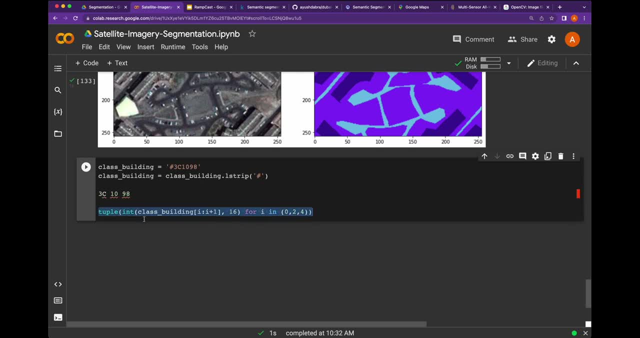 this whole tuple is what we need to convert that to numpy array. so process it. let's see what happens. this tuple became three one and nine. oh, it should be two, because this is one, but if we change this to I plus two, now you are getting 60 because remember, the base 16 of 319 was exactly three one and nine. 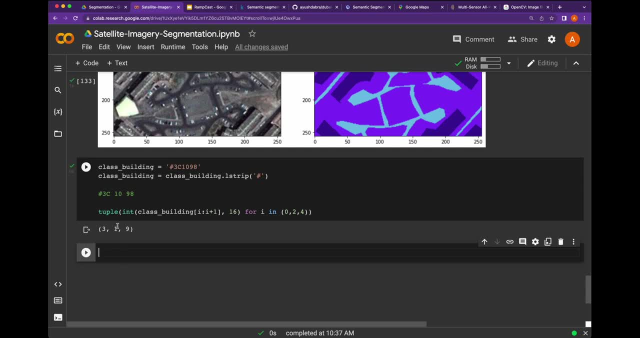 sorry, let's go back to one here. so the base 16 of 319 is always going to get the exact same number. however, once you say I plus two, you are getting the 3C became 60, 10 became 16, and nine it became 152. and now we need to take this thing, convert that to np array, so np dot. 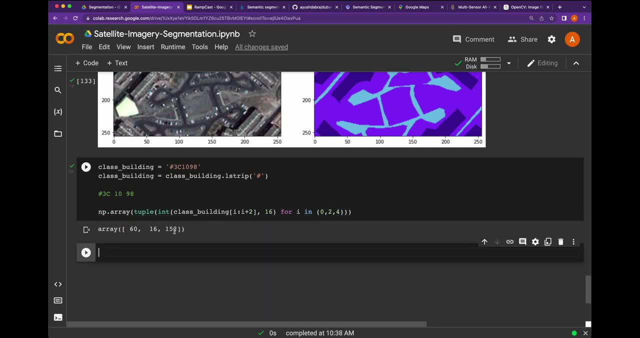 array, that's our array and that is what is our class building. so that's become the class building. so let me close this: that's how you got the class building. if you would want to print, you can get the class of building similar to that. we can take this and we can change this to land. 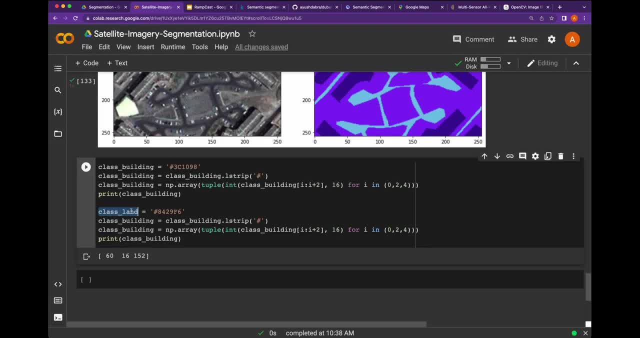 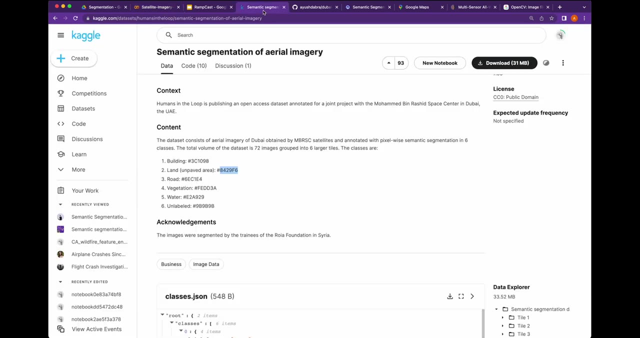 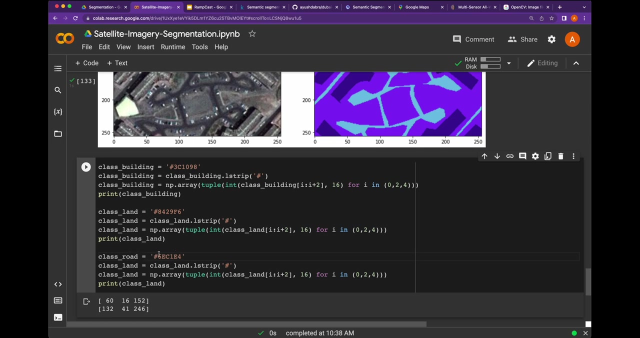 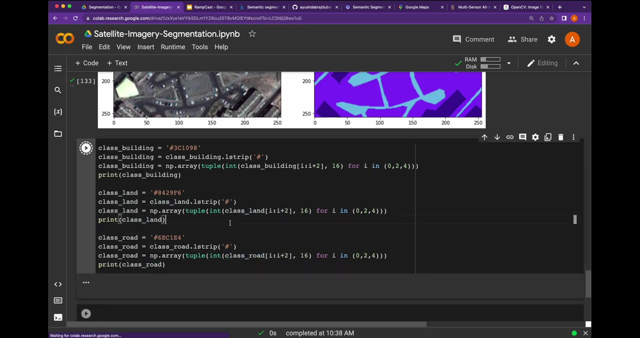 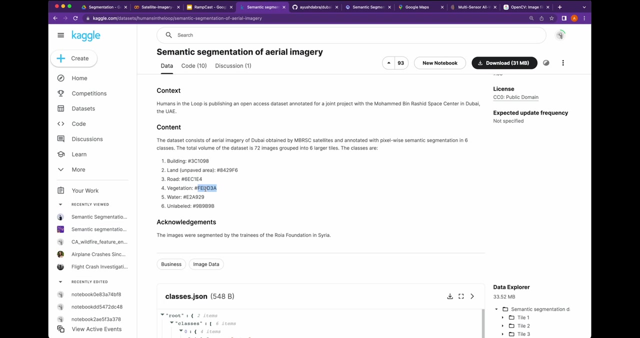 this is the value of land, and this land is what. now we are getting the value of length. next we need to do for each of these labels. third is our road. that is our road. next in line is vegetation. next in line is vegetation. next in line is vegetation. 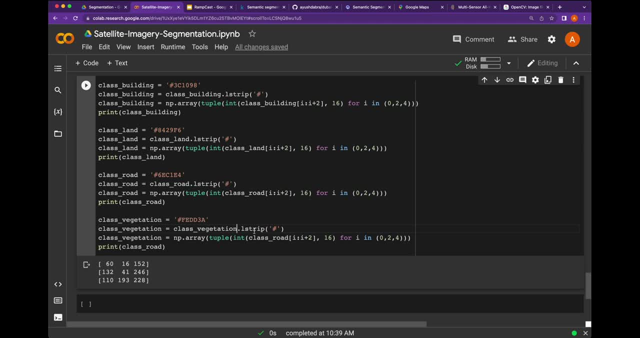 foreign, foreign. we have got the four rows module kind of sort of shut. we're trying to develop something in the nayime, we are going to develop something here called street views that connect all purpose. and we have got the four rows module kind of sort of transfer quality to one, every class Having ran over. so we 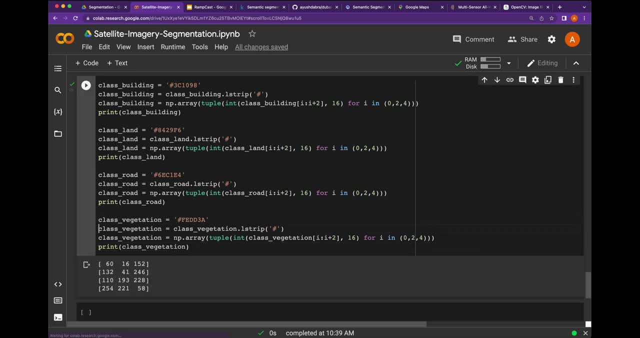 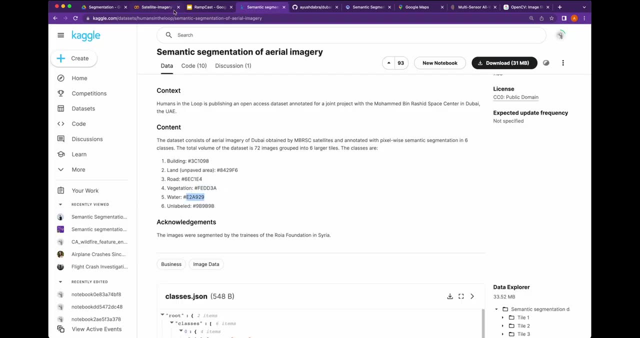 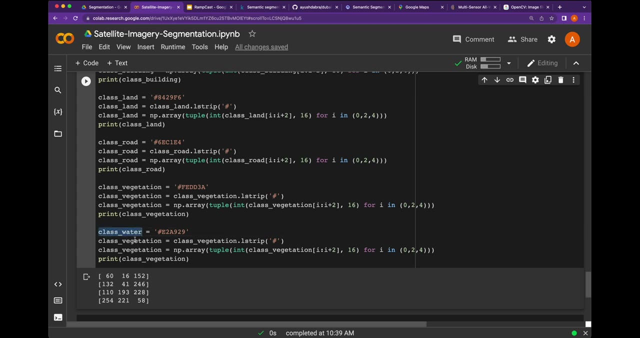 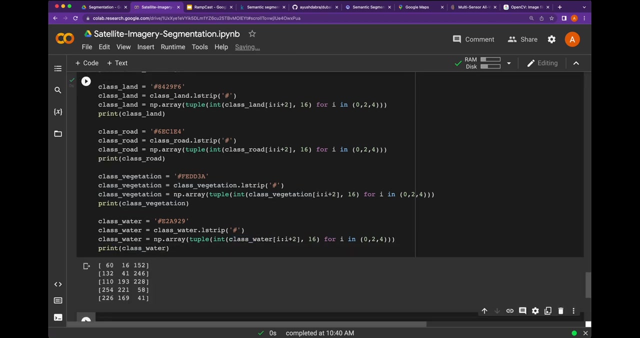 and now we can just take two steps- you see this from here- on how to get all your different infrastructure, all these systems are also part of this. okay, links from this trabajo: vamos con c? onun got vegetation covered, two more to go water. and the last one is the unclassified or unlabeled. 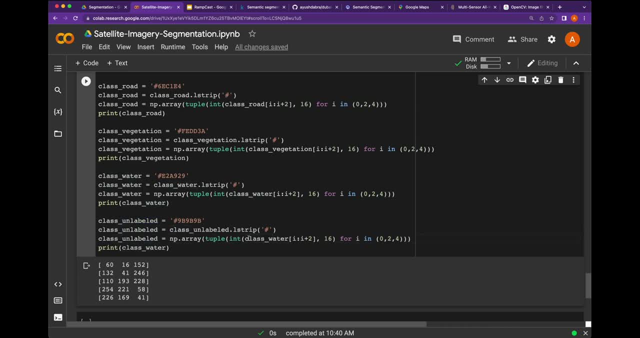 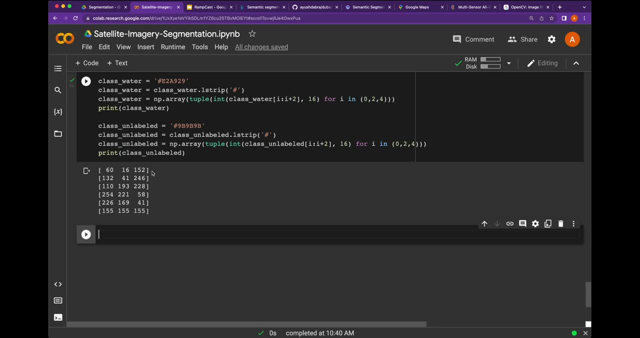 and all of these labels we have got into the class of numpy array. so these are our labels and because these labels only belong to our mask data set, we need to create a method which takes the rgb value and convert it to 2d label. so now let's try to get the labels out. i will try to. 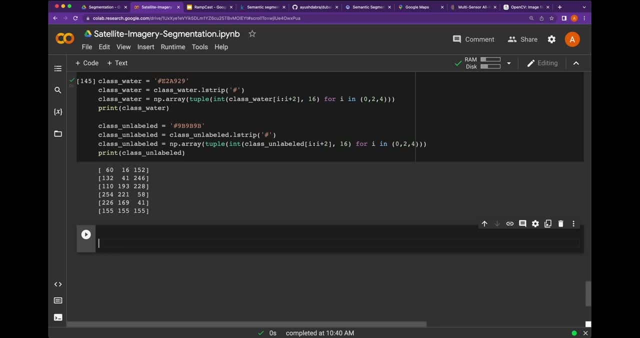 show you how we could get that thing too. so let's try to get the labels out. so let's try to get the labels out. so labels, so let's see how we can get. remember, we need to iterate whole mask data set so we can say, for i in the range of mask data set and the mask data set range going to be 0 to its mask. 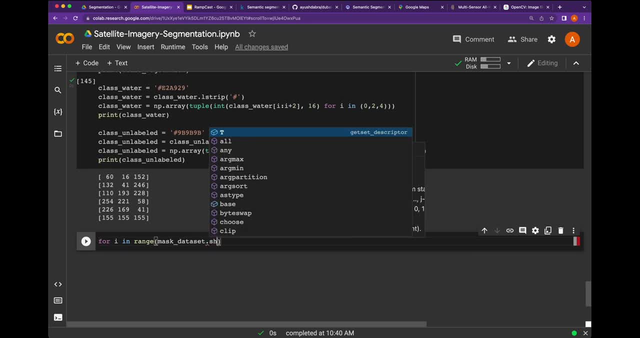 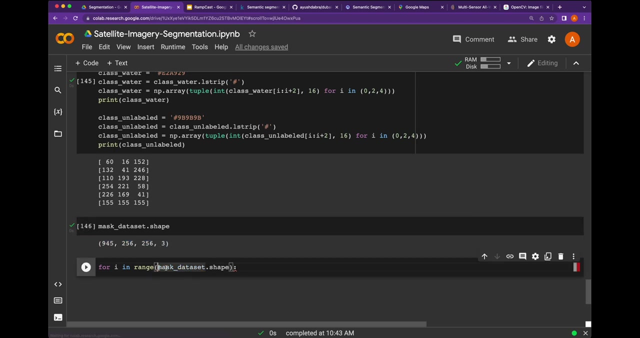 data set shape. so if we so the range, we want to create whatever the mask data set shape is. so let's get what is the shape. there are 945 images of size this, so the range will became shape of 0, so 945. so we need to get the range from 0 to 945. 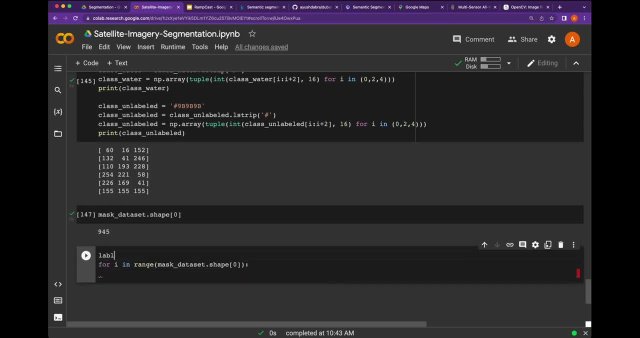 and we need to store all of these value into a labels data set. so that's our labels data set and we can say: label is equal to whatever we are getting from. so we need to take this mask data set of the input image of i, so the zero of whatever we are. 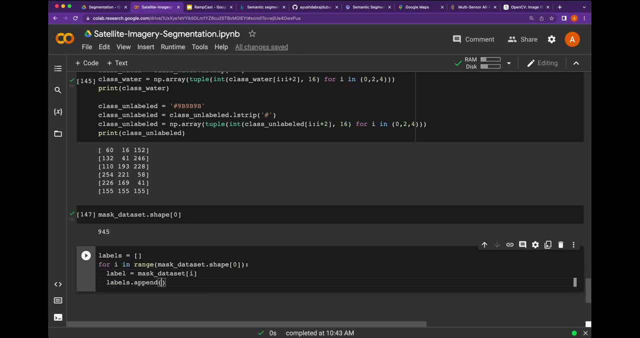 passing. so that will be the image. would be labels, dot, and, and that label is going to store. so we need to write a method which takes this and generate the label out for us. so that method is what we are: generate the label out for us. so that method is what we are going to write here. we will say: 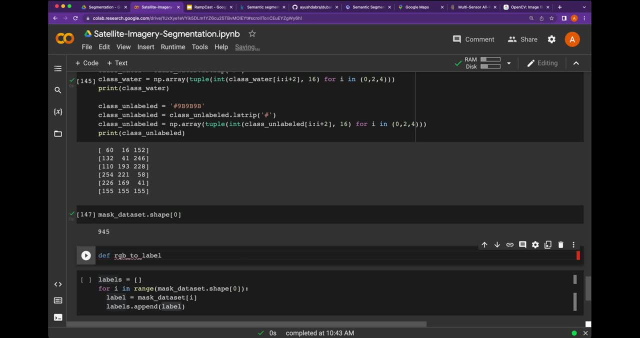 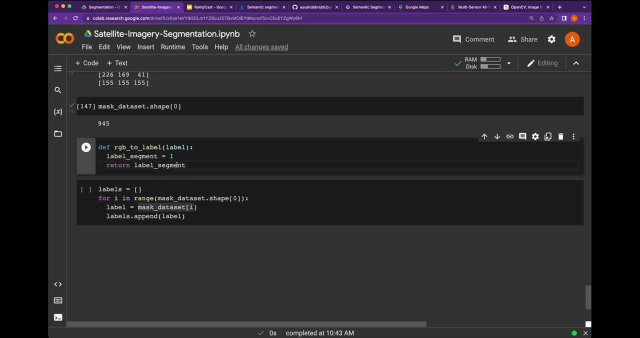 define rgb2 label and which is going to take a label value, whatever it's really being here and what it does is actually return the label segment. so label segment is what is going to return, just right here, and then we can say: return label segment. so this label segment is going to be. 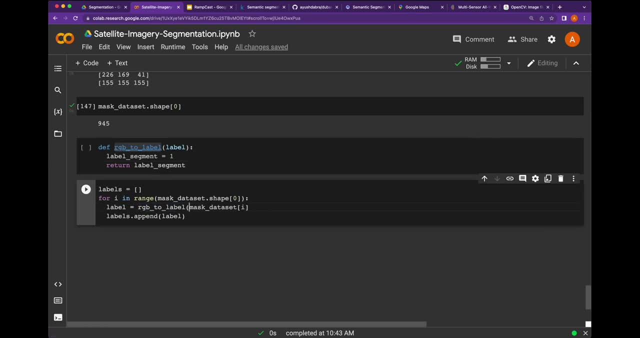 stored. so we will take this method here and we will pass the input. so less here, let's here. so that's our method. there is nothing code here which we need to write here, so depending on this code. so if you will say what is the length of our labels, it will be the length of our mask data set. we. 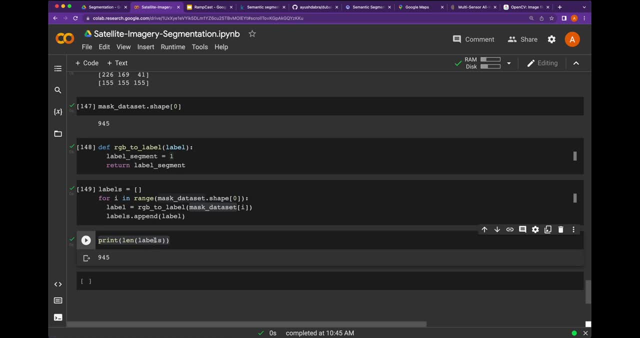 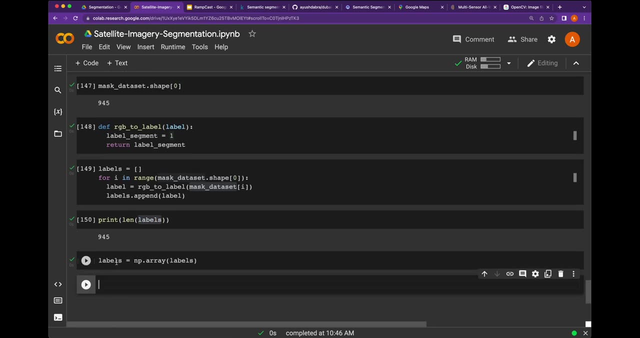 can say the length of our labels. so we can say length of our labels. we can say length of our convert this whole labels. we could say the labels are equal to numpy dot array of labels and then we can get the unique value of labels which we found in labels here. so if you look into the label, 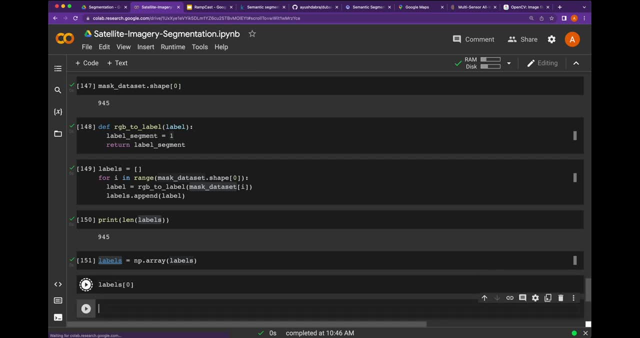 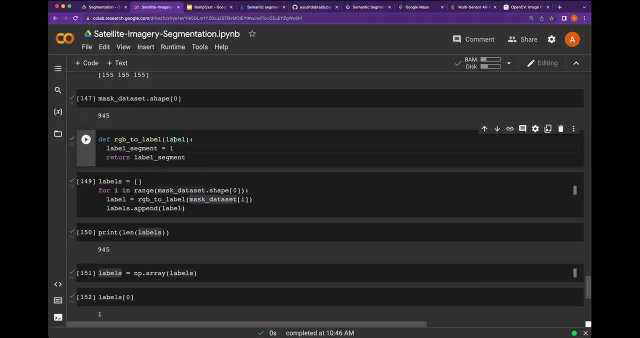 and the value, what we are finding into the zero, you will find one because that is what we are storing. so let's try to write code here. so this label or this input is what is really being set as this mask image data set correct. so what we need to do? we need to make sure that the label 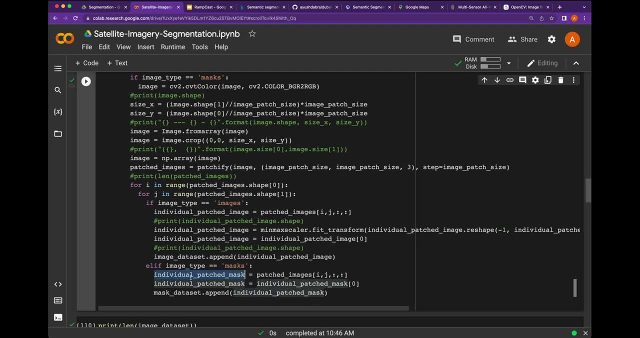 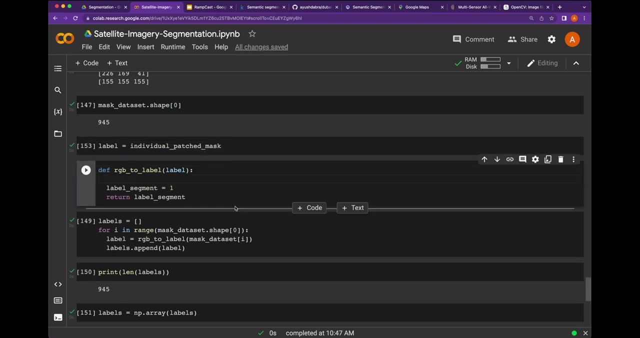 is equal to this patch mask, which we have created individual patch mask, so let me set it here. so that is our individual patch mask. so the based on this mask data set is input. we need to create an object which has the same size but filled with zero, so we could say the label segment is equal to. 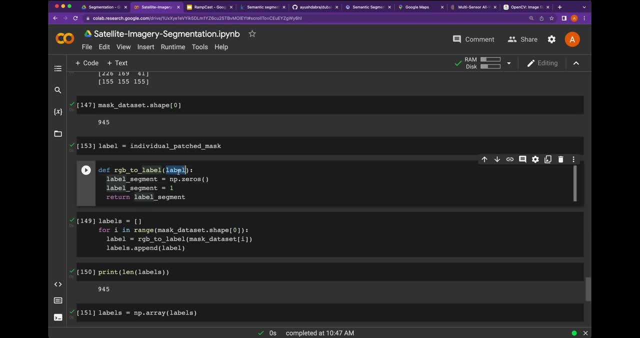 np dot zeros. but we need to provide this size so we can say shape of this and we can also say that if type should be, we need to provide the d type, which is np dot uint8. so this is what the label segment size. so this is exactly the size. so if you, 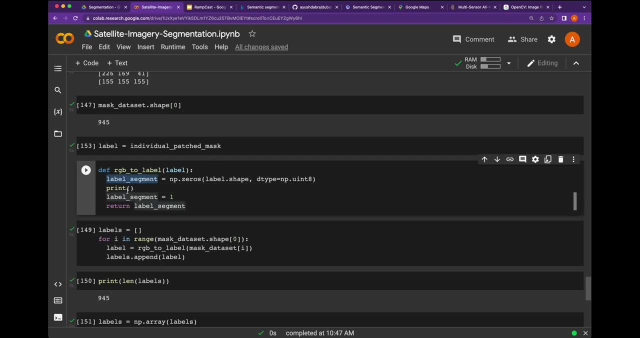 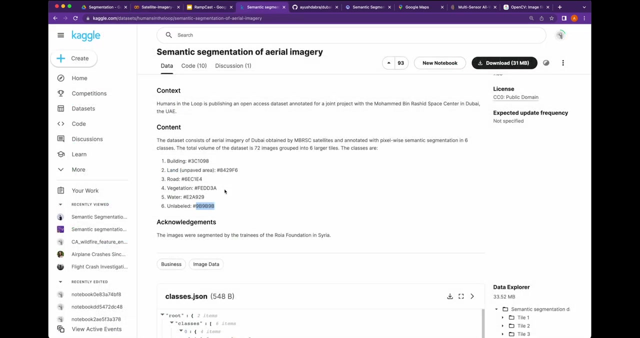 go ahead and you can say: print off label, segment, dot shape. that is what is going to print. so let me just run this code. if you input here, you will see this is a zero value, all filled with 256 by 256 of 3.. now we can look into the code. the water code is zero, then the 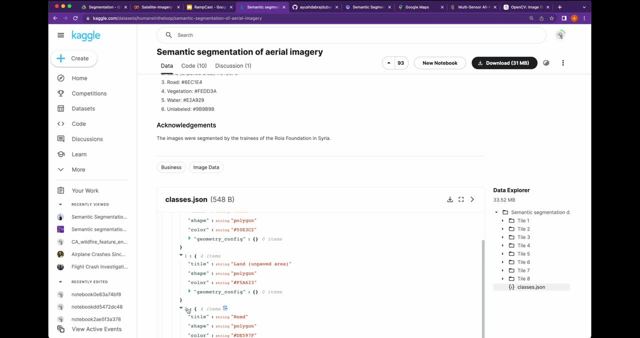 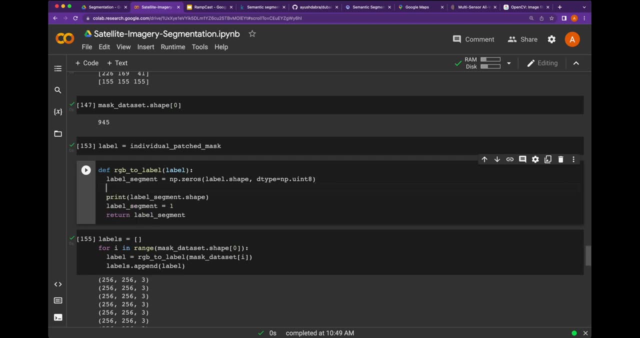 land code is one, the road code is two. so we need to follow this coding and we need to apply here, we could say, the label segment and then we need to make sure that we are processing it so numpy dot all. and if the label is equal to water, 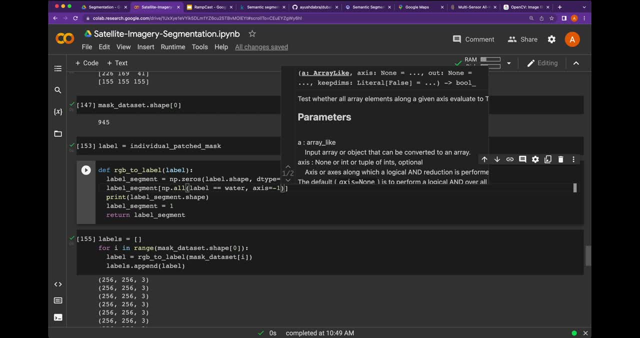 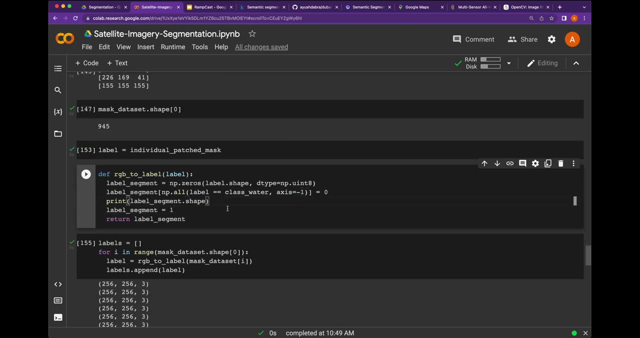 axis is negative, one is equal to, is equal to zero, so that is what is going to generate the class of water. that's where we got the class of water, so we need to perform exact same thing for all of these values. let's remove this. we don't really need this code anymore. so the 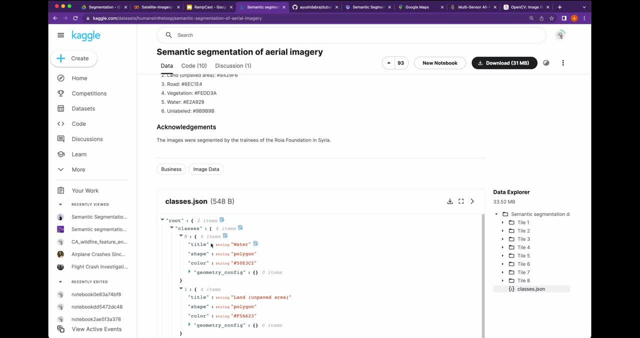 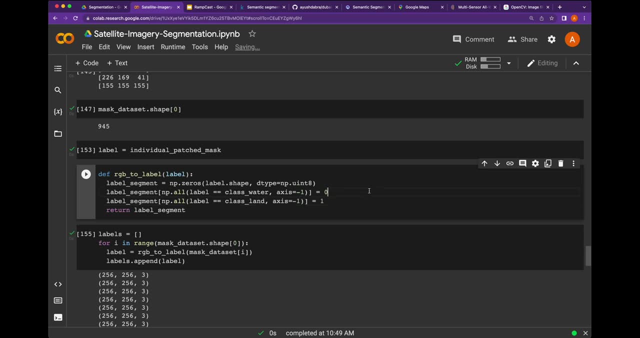 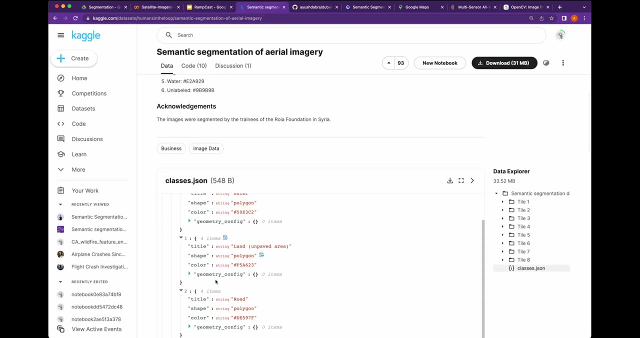 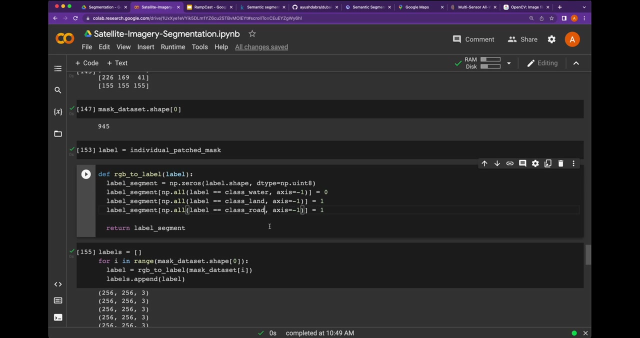 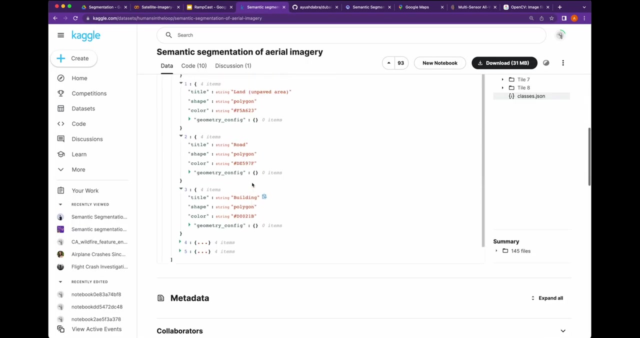 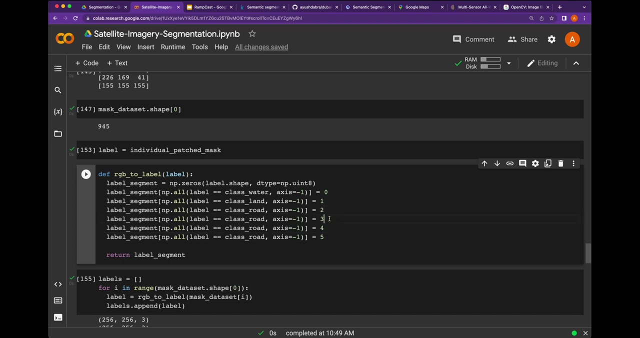 value, one we are going to use for after water, the one is for land, two is for road, two, three, four and five. two is road, is building, four is vegetation, five is unlabeled, two is road, three is building, four is vegetation and last one is unlabeled. so all of these classes has been processed and 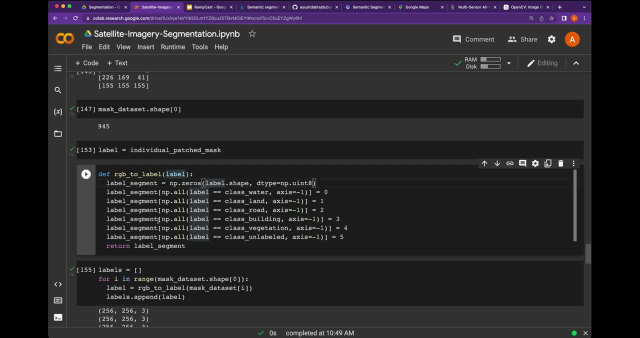 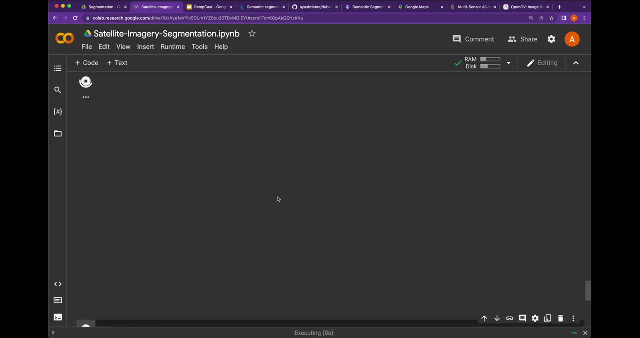 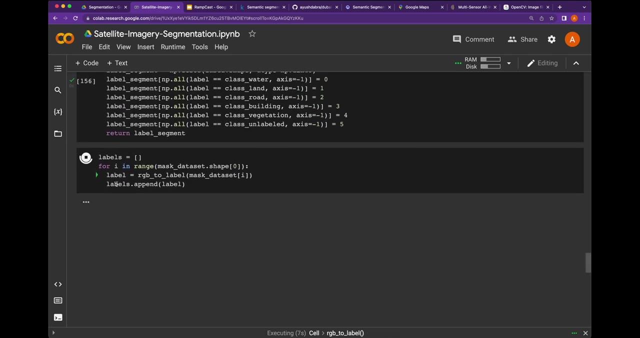 whatever the class of that mask image is going to be stored here. so let's run this method at this point from this code all the image content has been processing and then result is going to be stored into this labels data set. the size of labels data set will be the size of 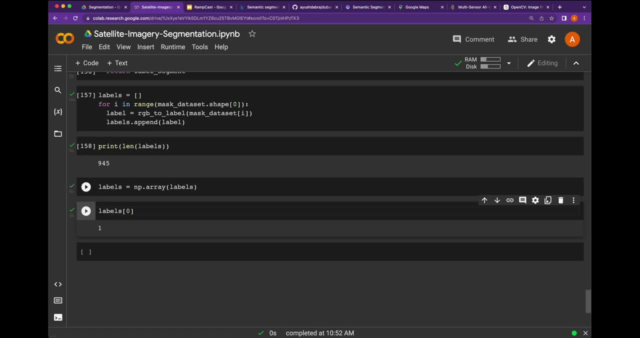 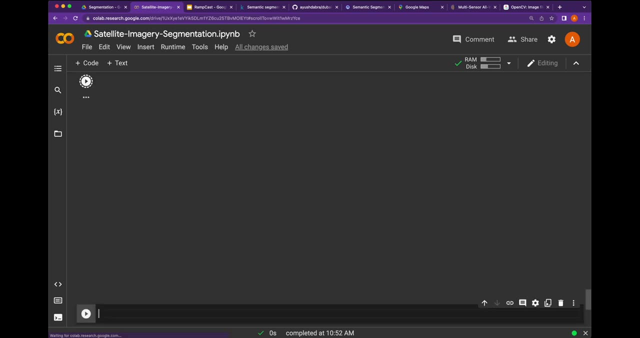 the mask data set. we are converting to the numpy array. and now if we look into the what is in label zero, you could see everything is one. what is the labels three? we are going to get some of these value, depending on whatever it is. so this is how you are going to get the value of labels. 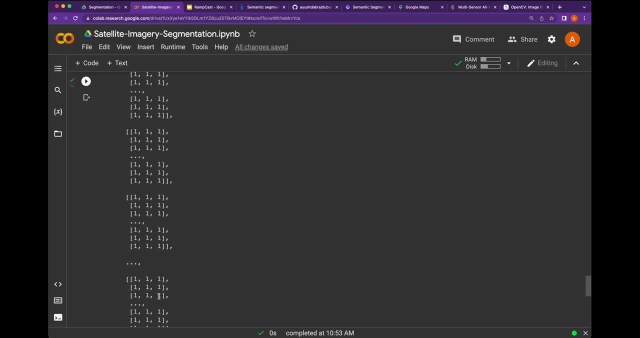 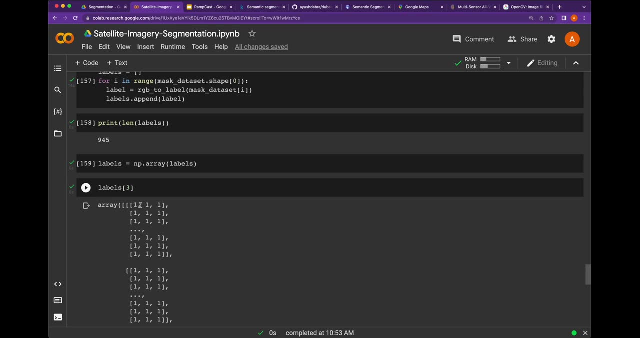 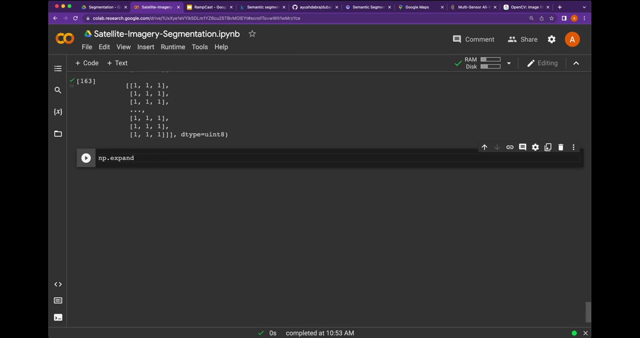 right now. i just wanted to show you that when you are seeing the label, you are seeing the result. something look like this way. so we need to make sure that we take this and we expand it, everything in a single row. so in order to expansion, we could say np, dot. expand dimensions for the. 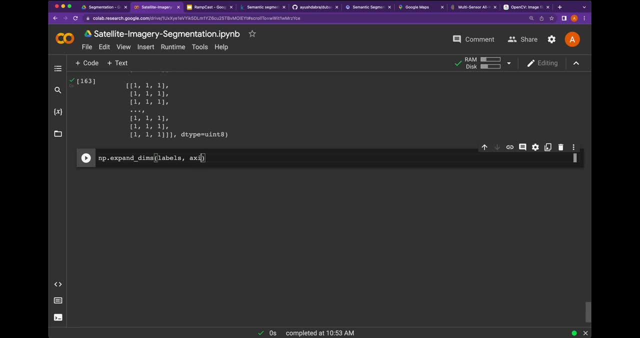 labels and we want to which axis? so you could say axis 3. this is how we are going to expand all these labels. now, if you take this label and say what is the zero, something is not right here, because i was expecting to see all of these values. they are: 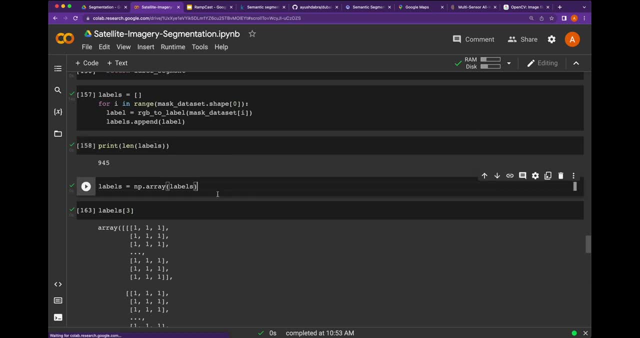 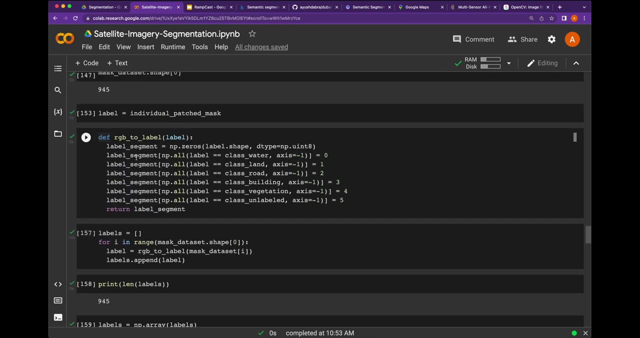 expanded and they are all in one array, rather than in the size of one by one, by one three and then for the size of 256 by 256. so let's take a look where the problem is. so, as you see that we, this expansion did not work, so we need to look into our this method, the segmentation. so here, 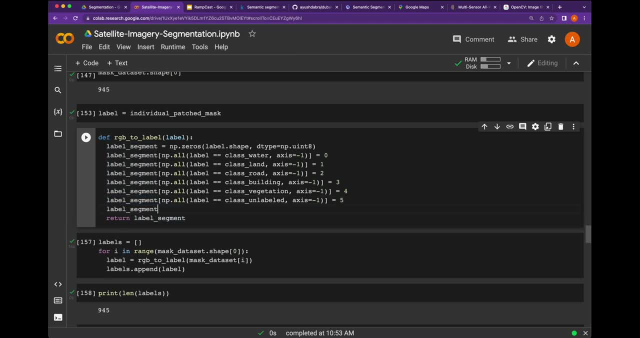 we are getting segment. we need to make a change in our segmentation. segmentation is that it's equals to. we take this and we slice it from colon comma, colon comma zero. because before we perform, let me show you that we take this label, segment and we print the label. 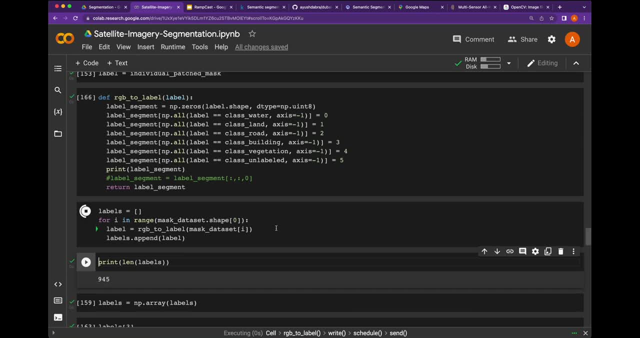 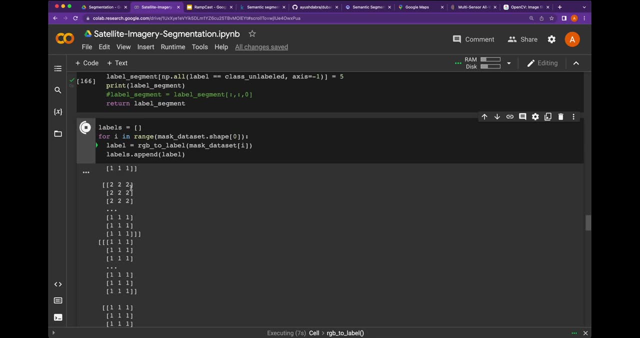 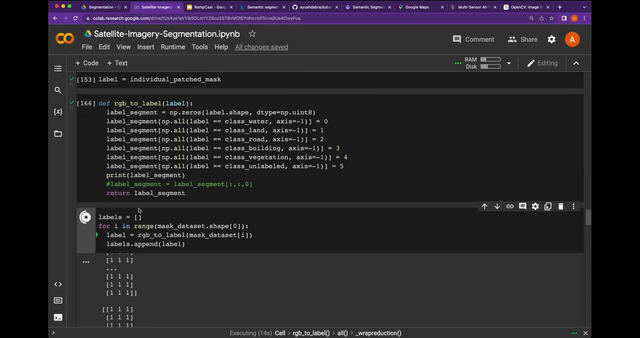 segment here and if you run this code, you are going to see the result. so you are getting this label segment this way. so we need to make sure that we take only one value out of this segment, because there are already multiple of these values. so in order to process that, we can write this code. 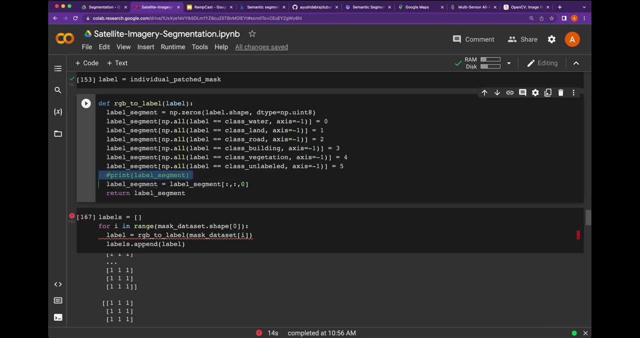 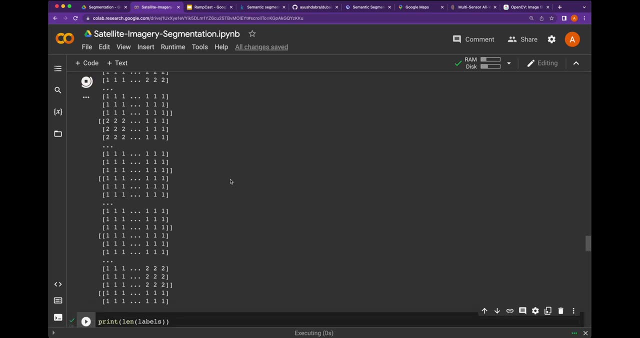 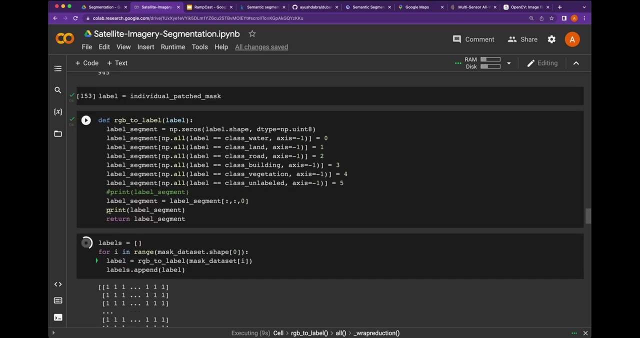 which takes this label segment and get one value out. so let's run this code again and then rerun this code. now you are getting the one value out of all of those segments, you, so this would be a better code. let me close this. stop it run again. 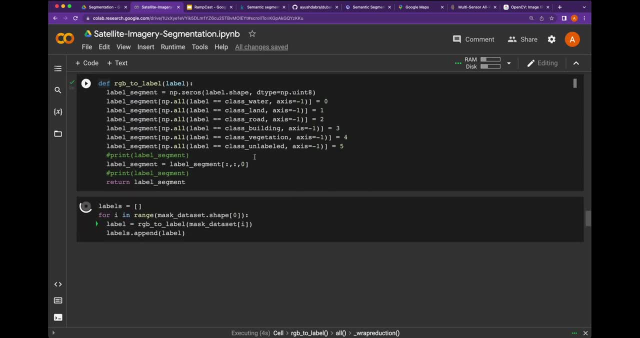 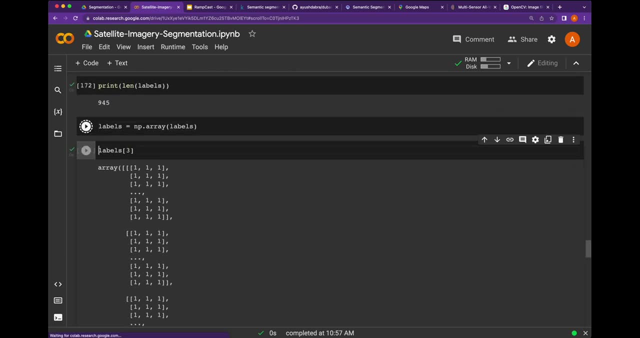 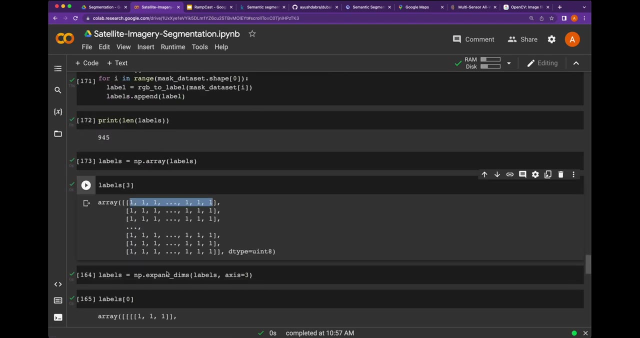 we run this whole code again. so now we have better formatted values stored in our labels data set. the size is still the same. we are making sure all the values in numpy array. now if we look into the labels you could see that all the labels are this: now we are changing the dimension. 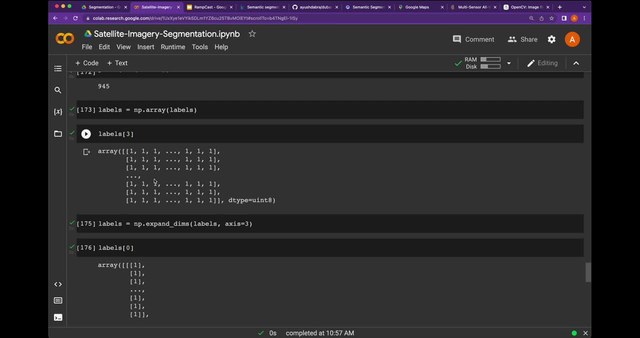 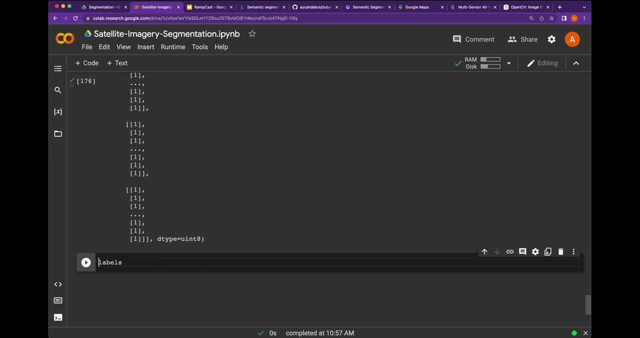 and now you could see that our dimension has been expanded from this direction to that way. so let's come back here. you could say: I need the unique value so you could use numpy dot unique labels and let's see what we are going to get. so we are going to get zero to five. so those 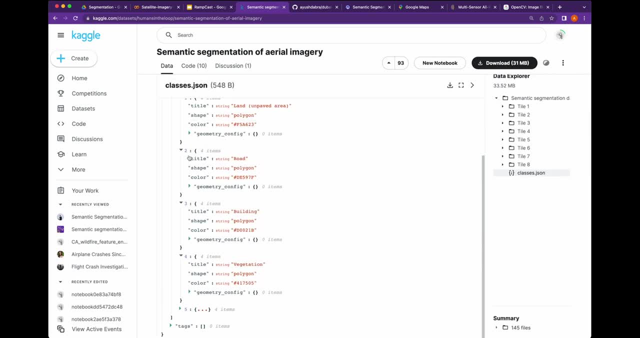 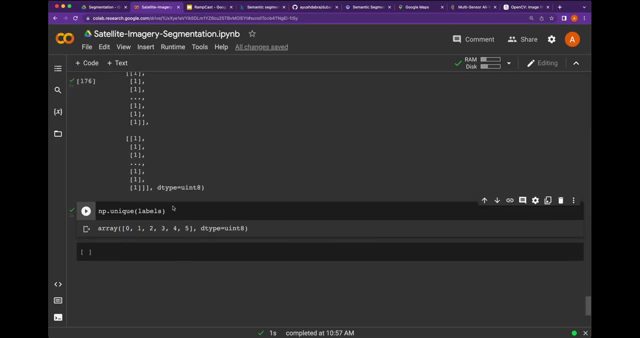 are the labels which you have is stored in in your mask classes and that's what we are getting: the unique values coming out from our mask data set. so this labels data set has these unique value, one to five. you could say print. okay, here will be the values and 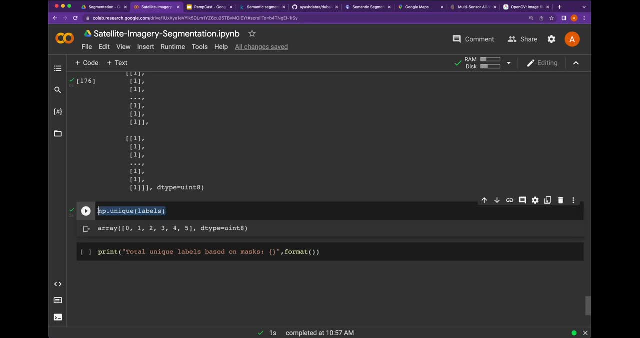 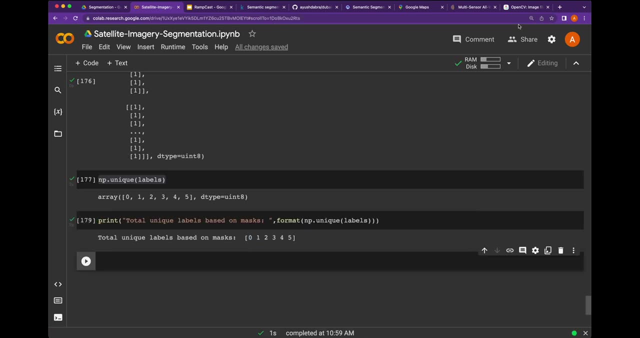 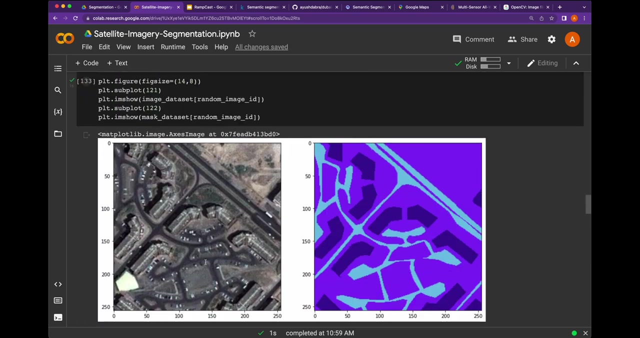 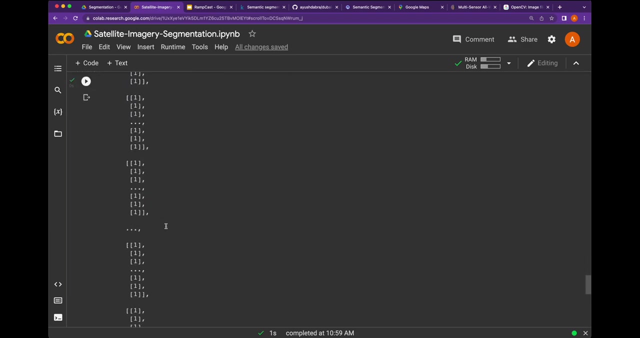 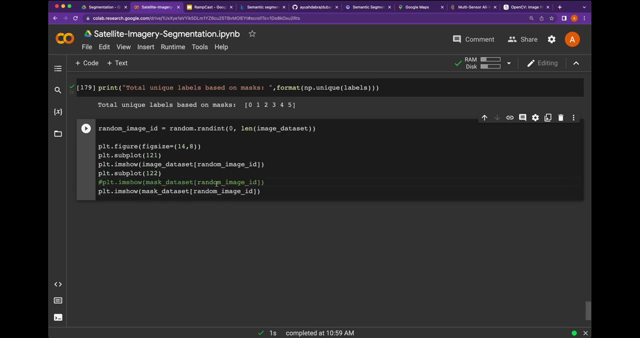 then format is going to be this value from this, based on mask. these are the 0 to 5 unique values. now we can render the output based on labels. we can come back to our printing code. that was our method printing code. we take this here and, rather than using this, we could actually change this to the labels. 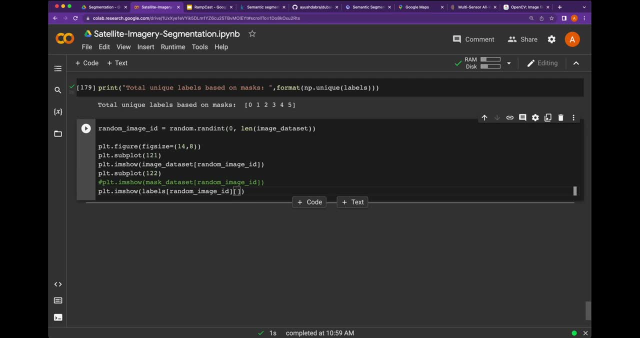 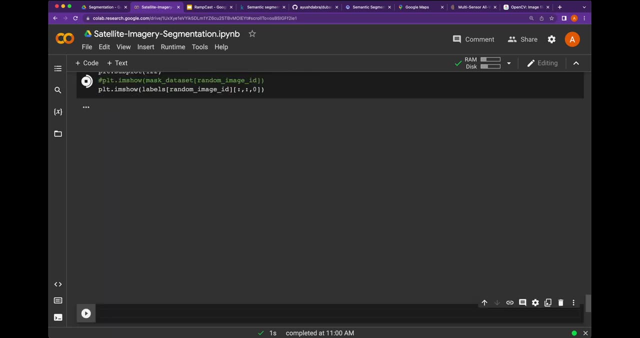 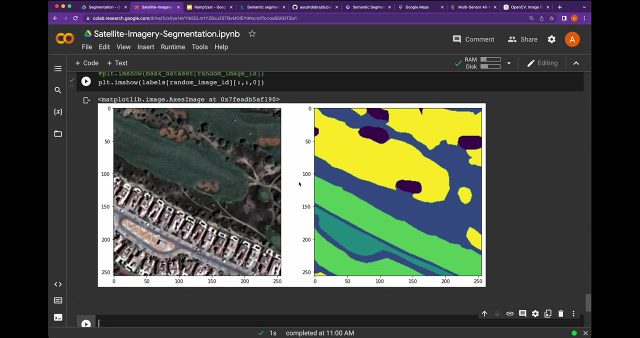 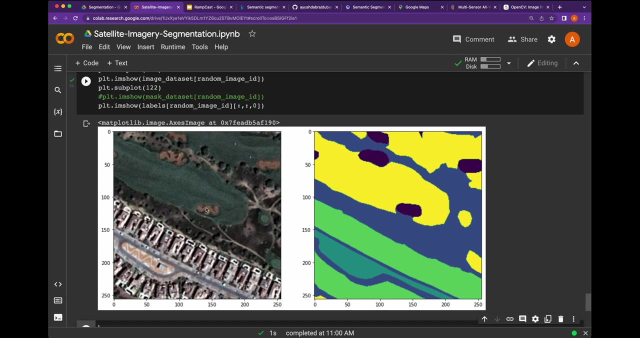 and we just really need to slice it. so let me first show you result and show you the reason how we are going to slice it and based on the labels, here you could get the results: houses, water, body, whatever it is. so now you are using the labels. so if we want to really 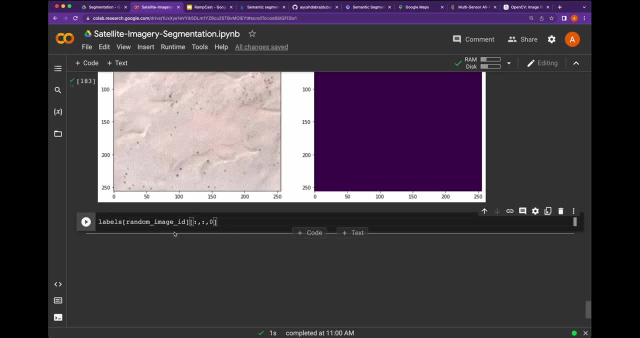 get an idea what it is, so you can take the labels, you can use the first image. that is what you are getting. but you see that most of the values are inside the one two array. so that's why we, if we try to slice it, we say what is in zero you are going to get. 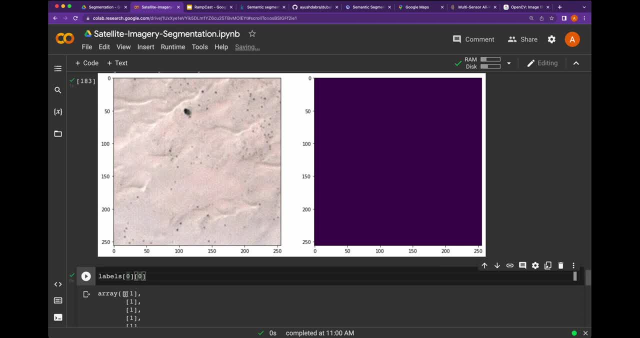 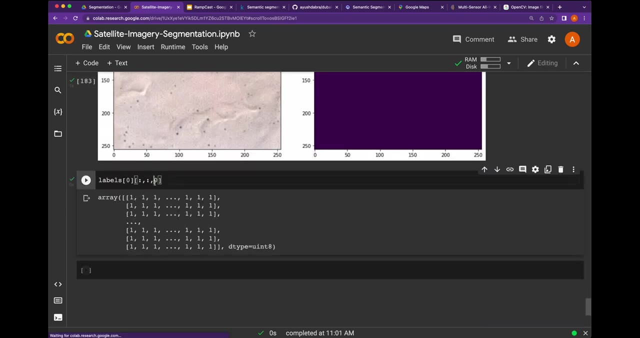 this way, then if you say i would want to get even further, so that's why you are slicing, so the slicing is: go to slice one, slice two and then give me the last value. so you can see that if you try to do the slice value, you are going to get these values out. so this is. 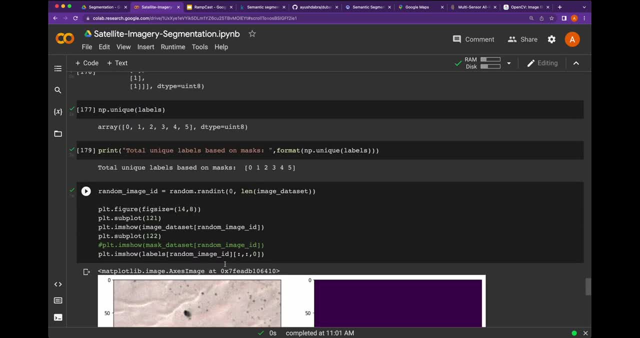 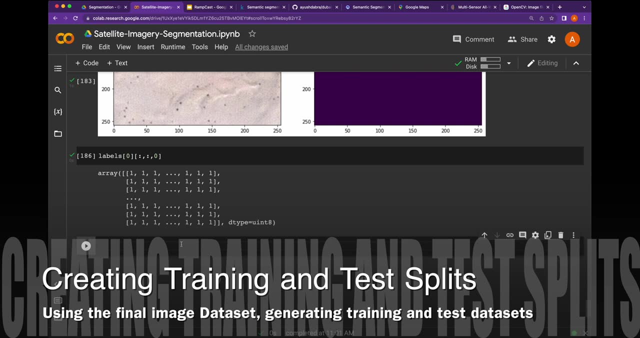 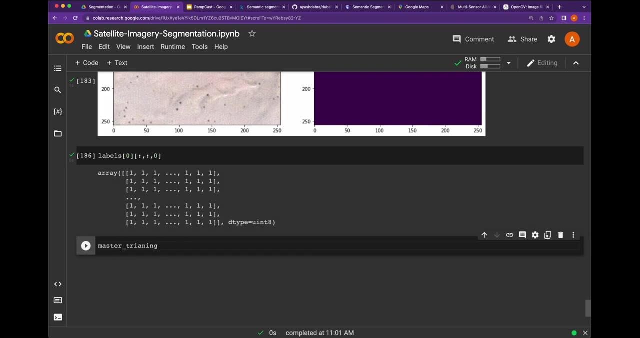 what has been used in order to process the images here. so that's why zero slice of that at this point we have final data set is our the image data set. so that will be our master training data set. so we could say master training data set is going to be the image dataset. 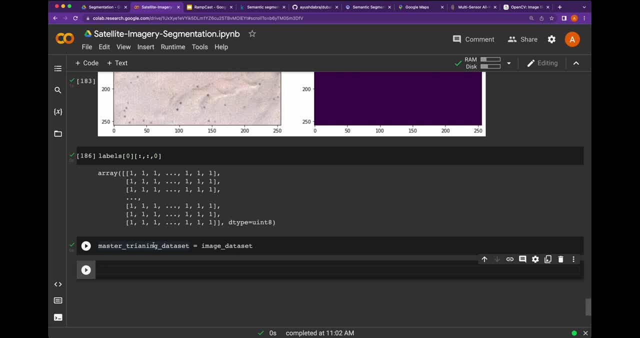 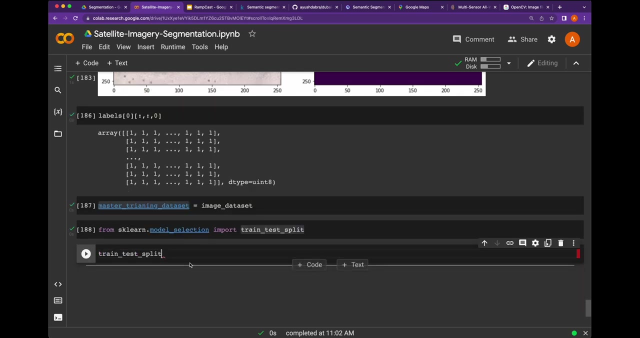 set. so that's our master training data set. now we can use the s scikit-learn, the train test split method, to split this into the training as well as the test data set. so we could say: from sk learn, dot model selection. we are importing train test split, so now we are going to use this. 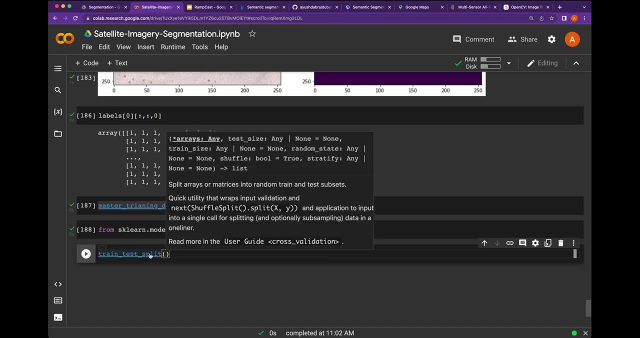 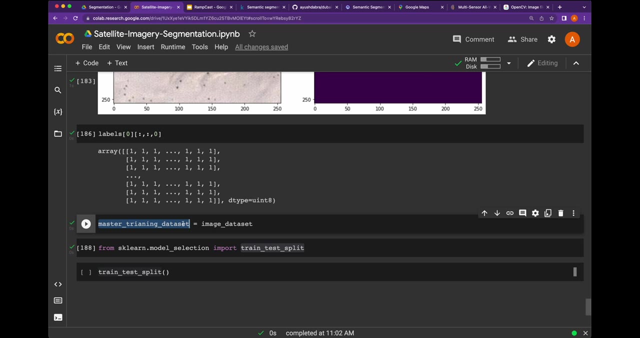 train test split method. so if you look into this- the definition of this method- this method really needs the input data set as well as the corresponding labels data set. so we need the corresponding labels. so we already have the input data set, but what is the labels category? so now, 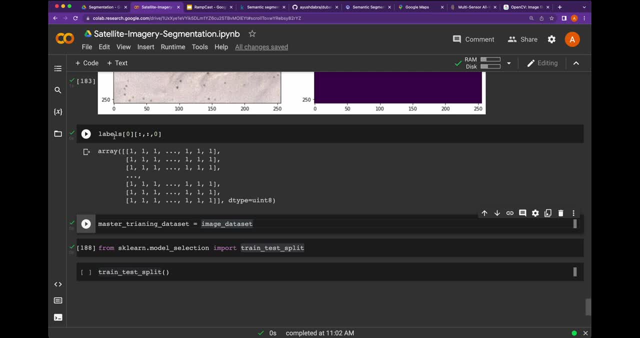 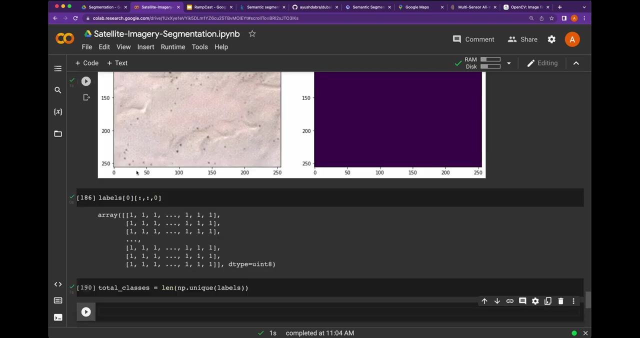 we need to make sure that we could generate the labels from our labels. so let me come back here and total classes. now we have total classes, which is going to be the np dot unique in our labels, the length of it. let's run this code: if we look into what is the unique total classes, you will get 6025. so we already know this part. 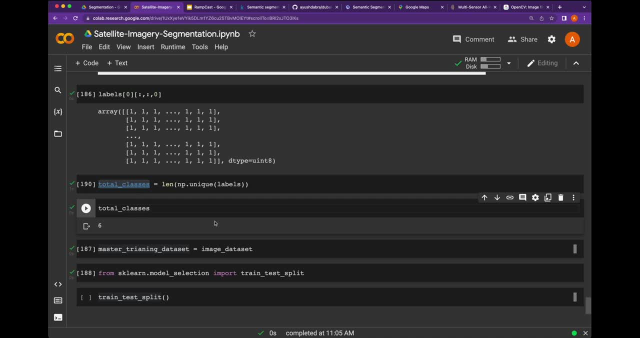 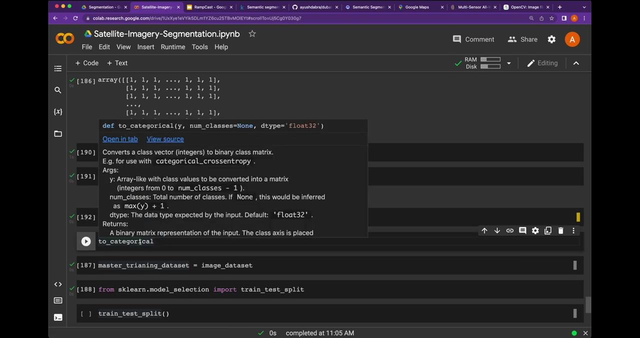 so now we need to create the categorical data sets for our classes. we could use the tensorflow keras utility, keras utility, which convert the categorical. so we could say from tensorflow dot, keras dot utils, import to categorical. and if you look into the two categorical, you need to process the labels data. 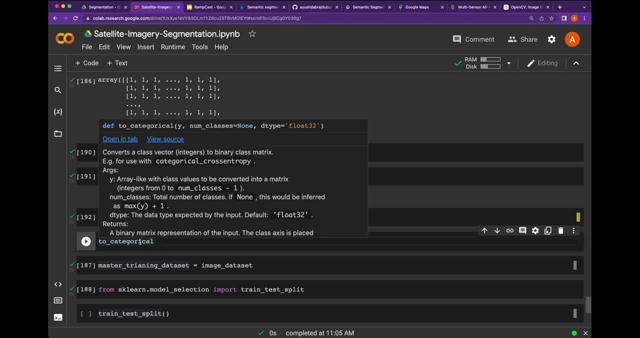 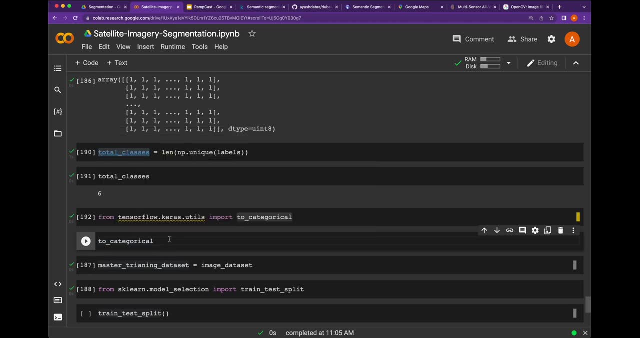 set as y total number of classes you need to provide and if you wouldn't want to provide the data type, otherwise we'll use the default data type. so we need to provide the labels data set, which is our input data set. we also need to provide the total number of classes, so the num 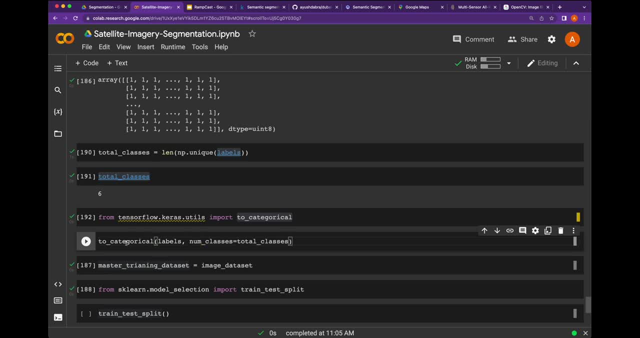 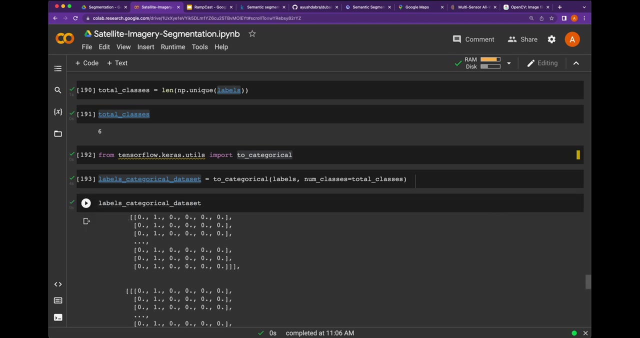 classes is the total number of classes. that's where categorical and this is what going to create the labels data set. so we could say: labels, categorical data set. let's take a look what is inside here. now you could see that all that categorical- one, two, depending on whatever it is. 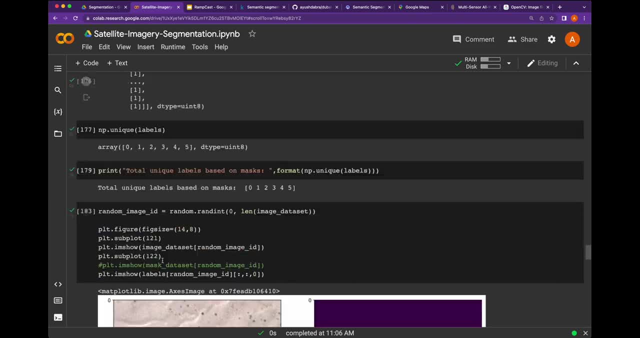 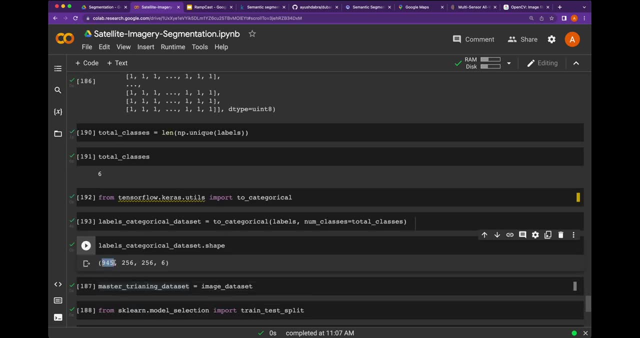 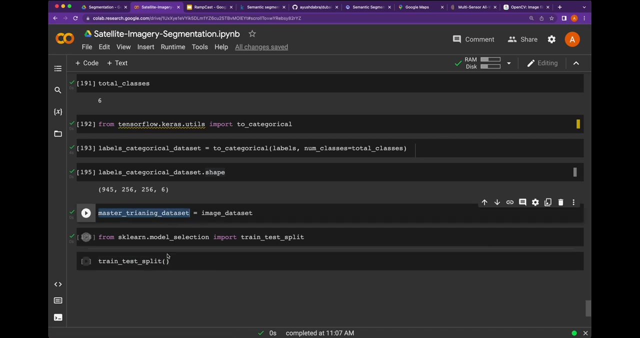 that's where our labels categorical data set is. we could shape so, for every masked label is size of 256 by 256 by six, because there are six classes. so this really proves that this data set is going to match our input requirement. so in this case the split is going to take this as an input. categorical data says as the labels. 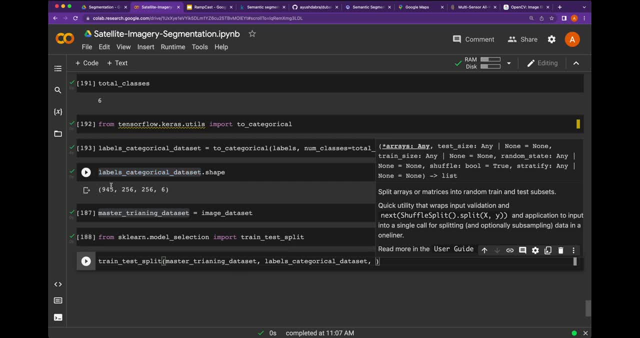 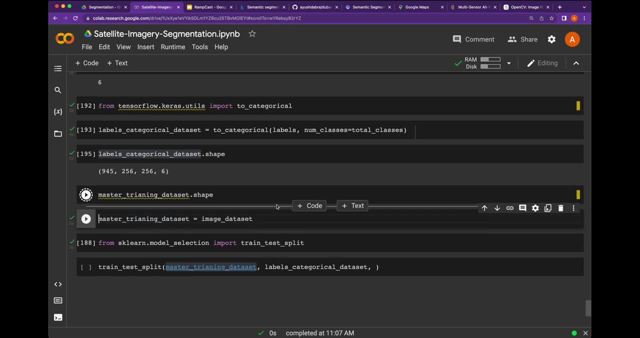 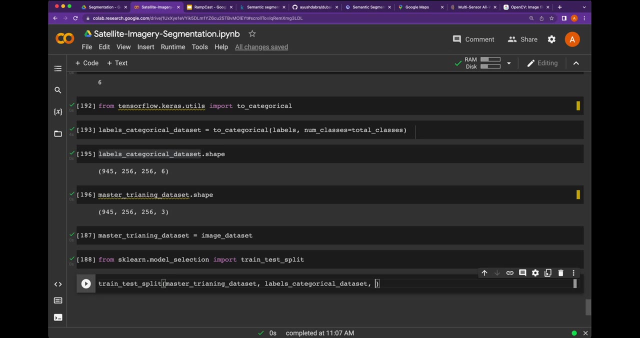 data set. so it really matches the 256 by 256 for 956 if you take this and let me give this shape of it too. so this is the rgb. these are the classes. everything is same. Now we need to provide the split size. We could say the test data set should be the 10%. 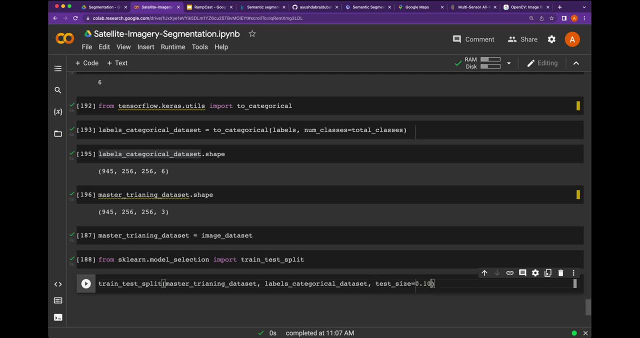 Let's put the 10%, which is 0.10.. I'll make it 15.. So 85, 15 split Random- I think this is the random state- Give 100.. So that's where we are going to get our output. 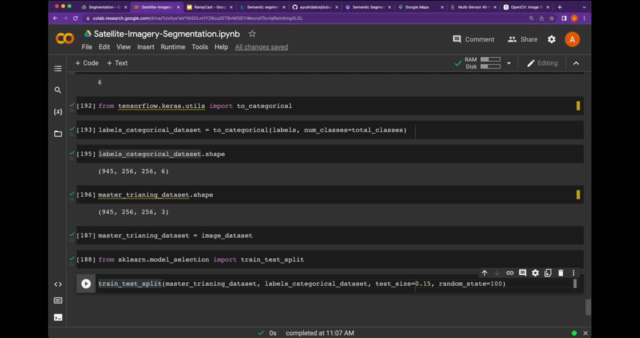 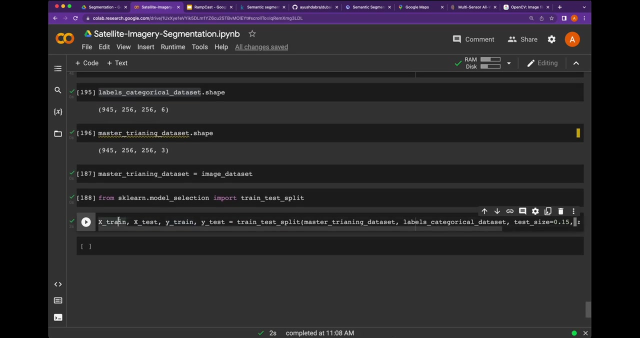 That output is going to be stored into the train and test split. So you could say X of train X of test, Y of train, Y of test. Run this code. Now, if we take this, let's print their shape. 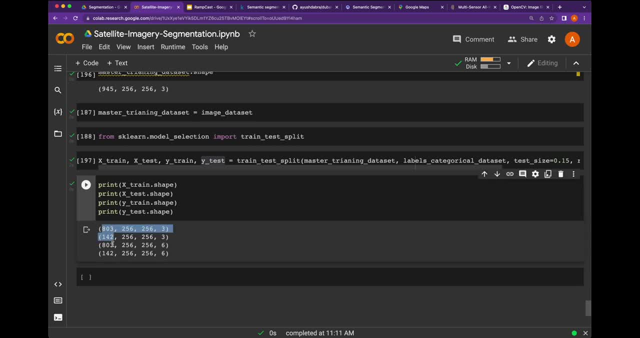 Print it. 945 images has been distributed in this one and as this way, So it's the same split. So what is the height and width? If you would want to get what is the image height, that will be the- whatever your training is- dot shape of 0.. 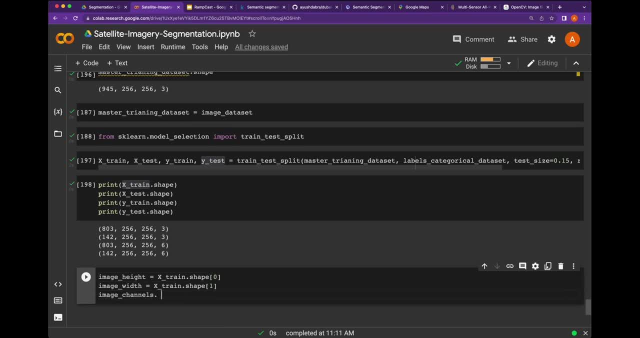 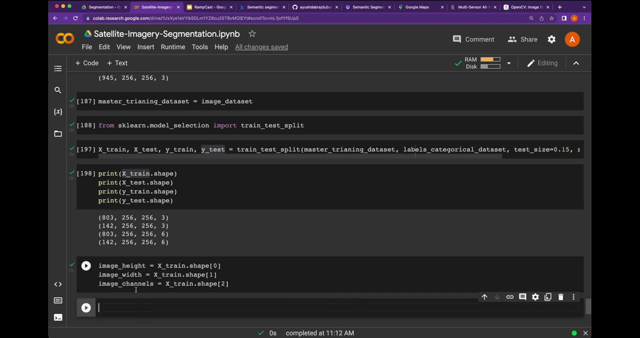 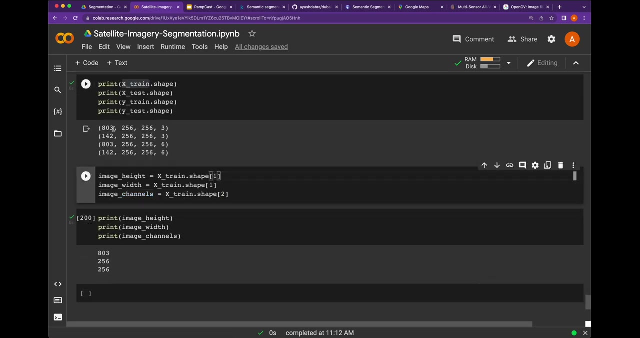 If you would want to get the image width, it will be the 1. Channels. you could actually use this, and that will be the 2. That's how you can get these values and then you can print them out. also- Sorry, it should be the 1, because the very first one, that's the size. 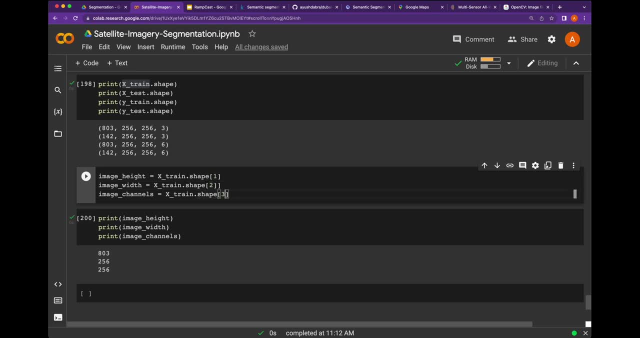 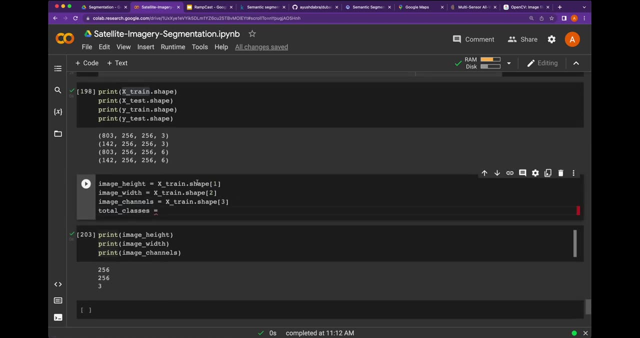 That should be the 2 and that should be the 3.. So 256, 256 by 3.. If you'd want to get the total number of, you will need the last element from the Y train or Y test. So you could say here the Y train of the shape 3.. 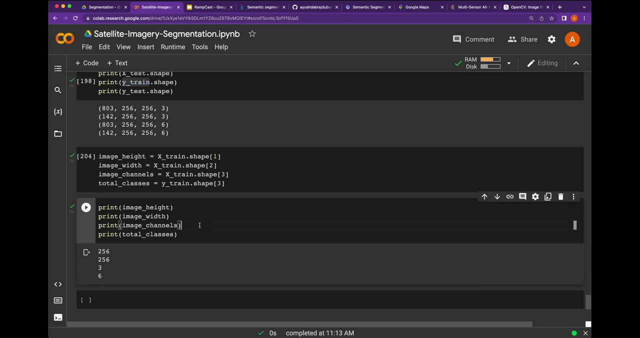 That's how you will get a total classes. So we are going to close our tutorial for the part one of this workshop here related with data preparation for our deep learning with satellite imagery. In the second video we are going to Perform end-to-end machine learning using the unit deep learning model and we are going to start from there.